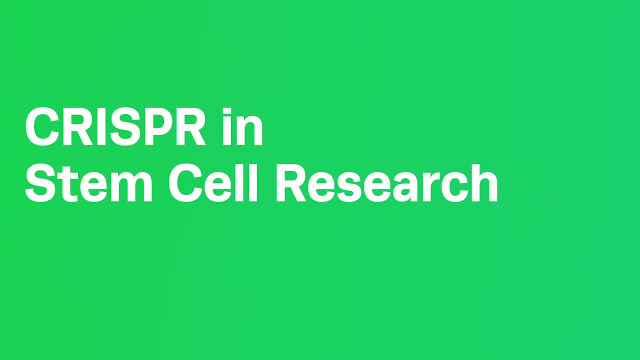 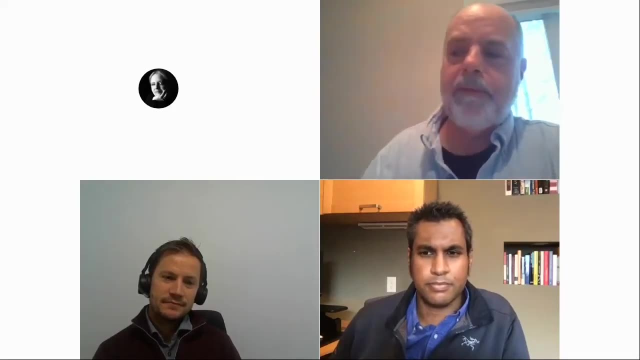 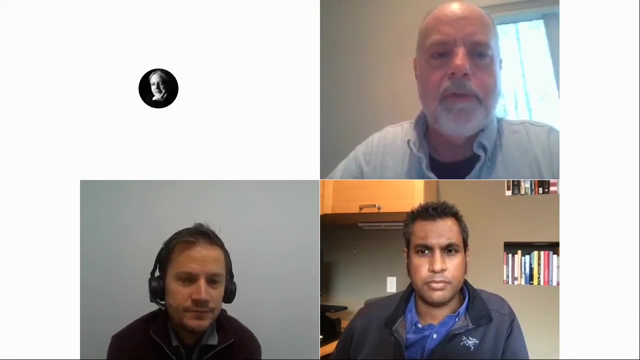 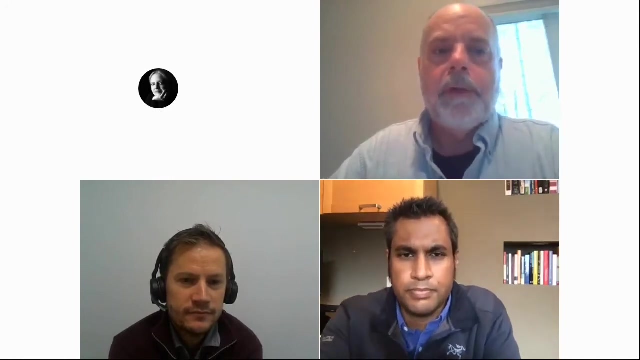 This is the session on CRISPR in stem cell research. We have three great talks, so please stick around. We're going to be talking about the application of CRISPR technology to induce pluripotent stem cells as models of normal biology and disease. 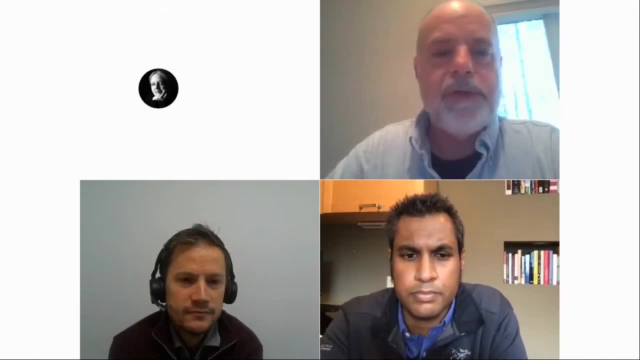 and also CRISPR activation and interference technology applied in hematopoietic stem cells. My name is Bill Skarns, I'm a professor at the Jackson Laboratory for Genomic Medicine in Farmington, Connecticut, and I will start by talking about high-throughput gene editing. 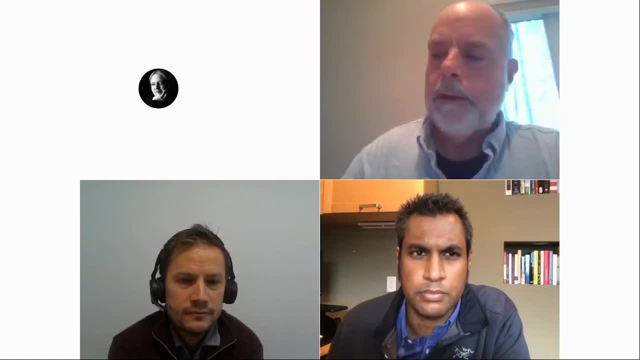 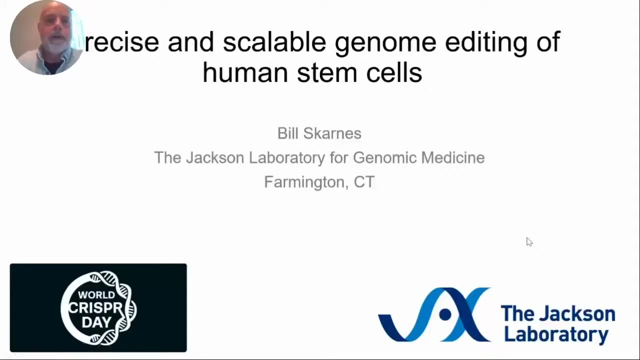 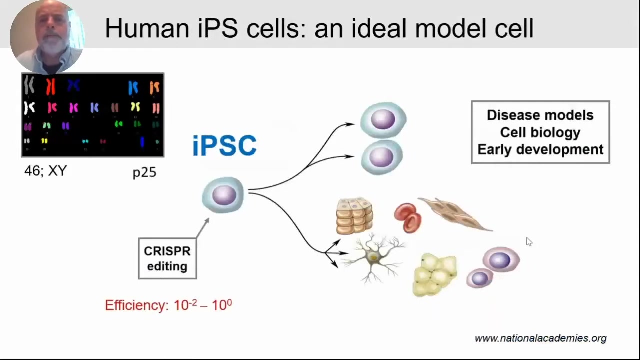 using CRISPR technology in induced pluripotent stem cells of humans. Let me share my screen, Okay. so the title of my talk is Precise and Scalable Genome Editing of Human Stem Cells, and I've been working with engineering of stem cells for over 30 years. I started 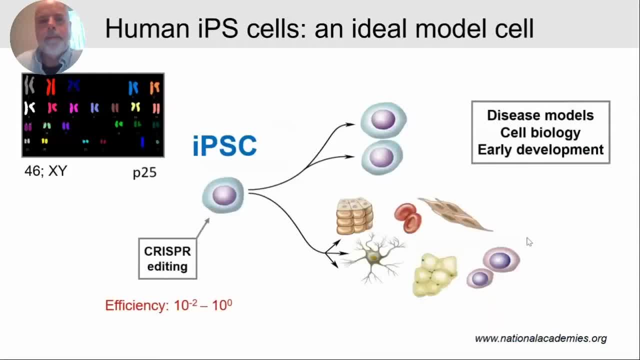 with mouse embryonic stem cells, which was about the only cell type that was easily engineered using conventional gene targeting strategies. Human iPS cells and ES cells were very difficult to engineer in the early days until CRISPR technology came along, and so I think the CRISPR technology has really opened. 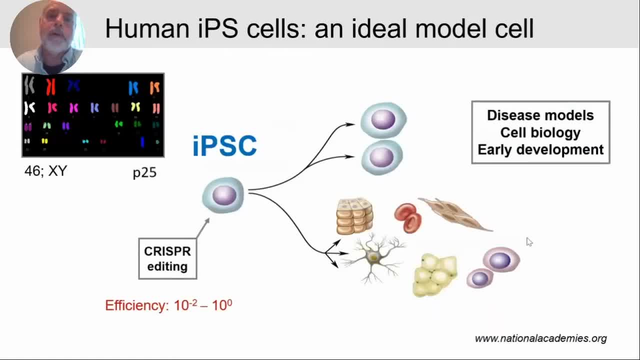 up the possibility to actually start thinking about doing large genetic screens in a model cell, and I think the human iPS cell would be an ideal model cell to understand human biology and disease. So these induced pluripotent stem cells, sometimes referred to as the homeless cell type, Polyps, diurnal cells, can 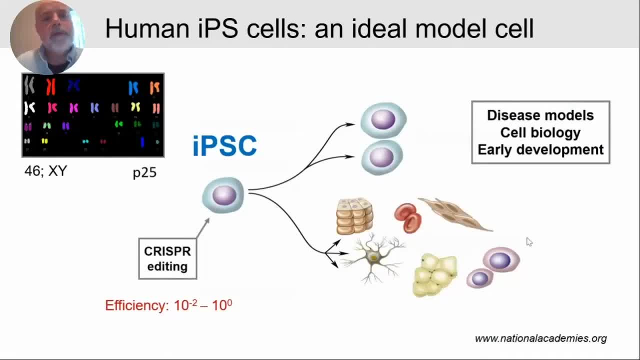 be maintained indefinitely in culture and they're relatively stable, so they can maintain a normal karyotype for at least 25 passages in culture. that's not to say that they can't pick up other kinds of mutations or small rearrangements and so on, but they do maintain a normal karyotype for quite a. 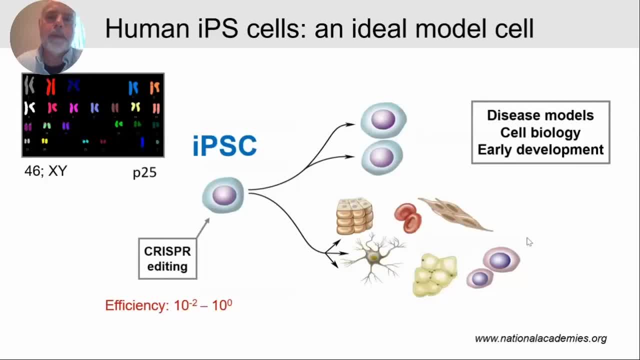 long time, which makes them a good, I think, stable model to work with. Now, induced completing in stem cells also have the property you often have to keep in your diet. you can differentiate these into virtually any cell type of the human body, So we can use these. 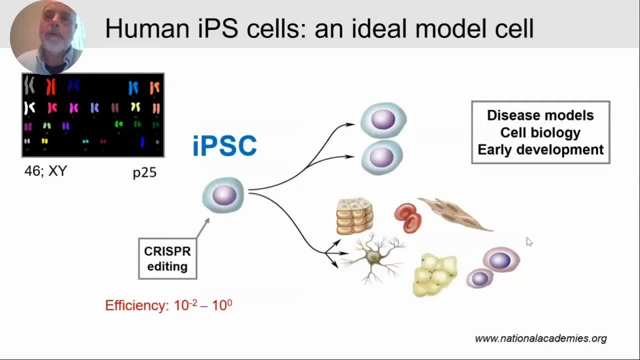 iPS cells to model what's going on in different cell types. We can model diseases in different cell types And I think they're just a fantastic platform for just understanding basic cell biology and early development, because these are normal diploid cells. This is unlike other cell types. 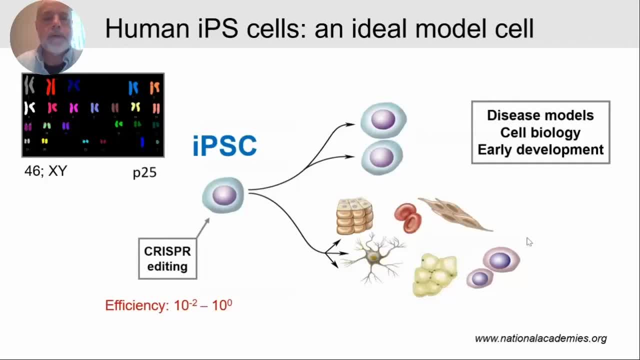 which have highly abnormal genomes. Now I'm going to concentrate really on the CRISPR editing potential in human iPS cells And I will show you some data which is very impressive, where the efficiency of CRISPR editing is now approaching 100%. 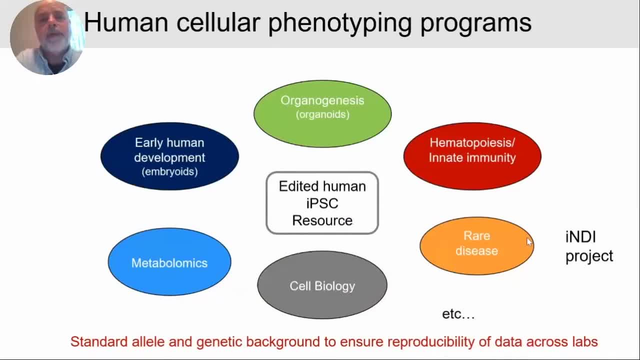 So with such efficiency in editing of human iPS cells, one could envision in the future organized programs of cellular phenotyping around a resource of edited human iPS cells, because we have access to a wide range of biology in human iPS cells, which include early human development, with 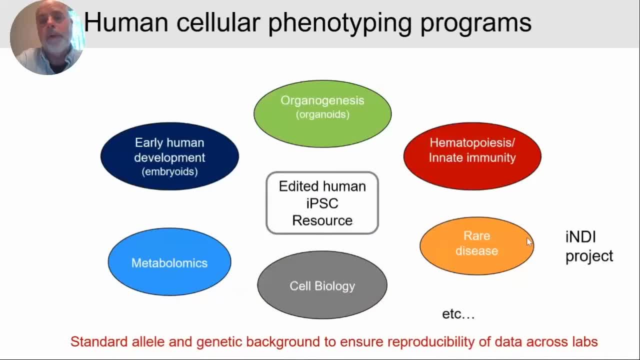 the development of embryoid cultures, organ development. with organoid technologies We can study hematopoiesis and innate immunity. We can apply large genome-wide screening like metabolomics. We can do detailed cell biology. And what I want to focus on today is a rare disease project that we've just started with the NIH, which we call the INDI. 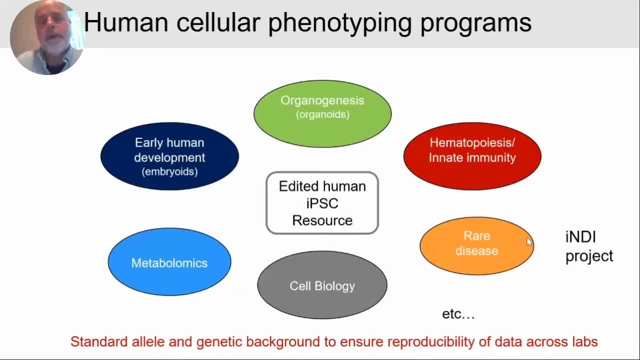 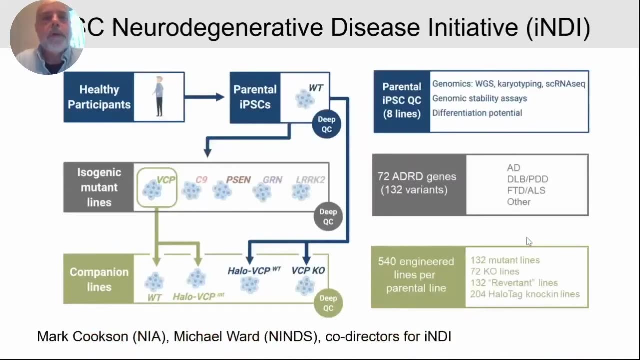 project, And I think the advantage of thinking about this in an organized way is that we can generate standard alleles on standard genetic backgrounds for the research community to ensure reproducibility of data across different labs. So the project that we started in June is called. 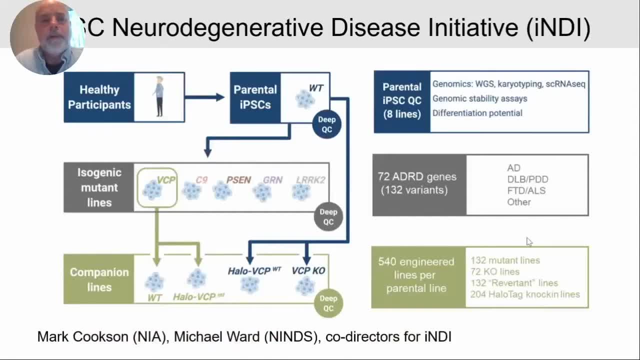 the iPS Neurodegenerative Disease Initiative. This was the first project in March of 2020.. And it was an international project that the university and the Institute have co-authored and are now in a. This is led by two very talented scientists at the NIH, Mark Cookson and Michael Ward. 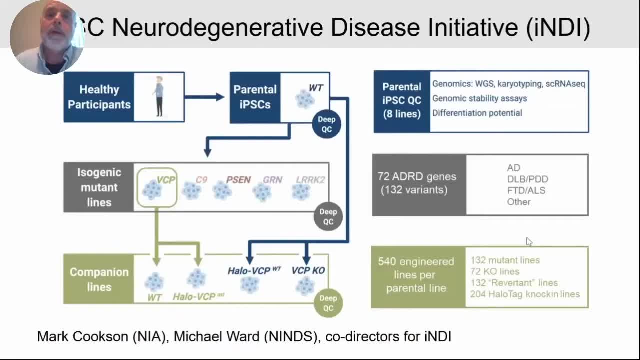 and they envisioned this project as a way to develop disease models of Alzheimer's disease and related dementia, but starting with a wild-type, what we call reference iPS cell lines. So, as opposed to using patient-derived iPS cell lines, we can actually engineer. 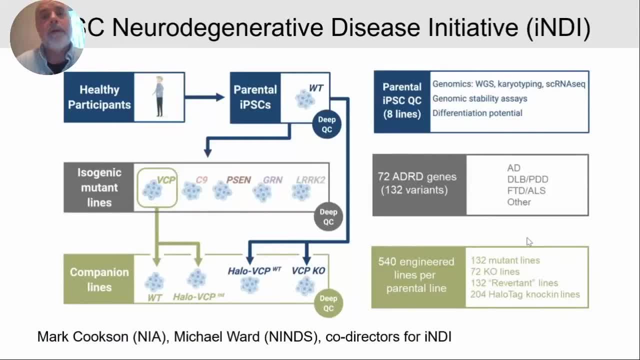 patient mutations into a wild-type background from a healthy participant to generate large numbers of disease models. And so this project is going to. it's a very ambitious project and it's going to go on for about four or five years where we will be introducing 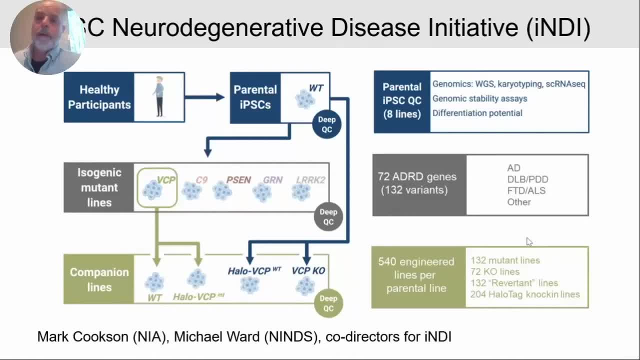 mutations that are specific for Alzheimer's disease and related dementia into a wild-type genetic background. We will be characterizing these clones very deeply to make sure that they have maintained a normal genome and have normal differentiation properties and that these cell lines will then go out to the community for detailed study. So in addition to the patient, 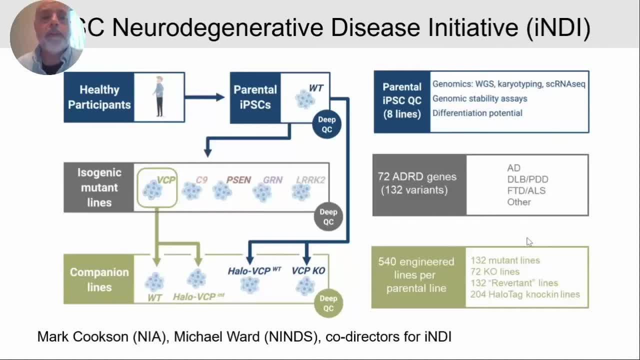 mutations. we also are going to start generating what we call companion lines in the patients' brain. So, in addition toJalopy, the patient mutation gene or DNA genome is can be a…int Polsce, and one of these lines is going to include a very important 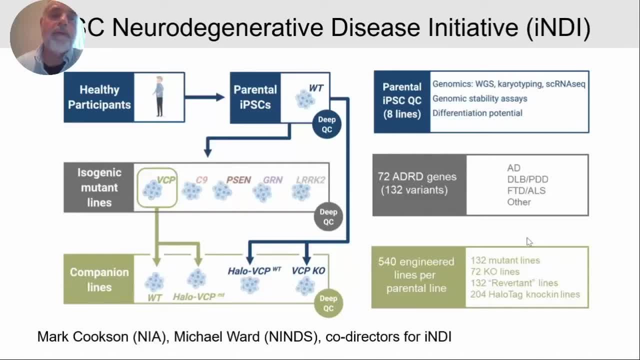 control, which is to take the patient mutation and revert it to wild-type, And this should be extremely useful in controlling for any genome instability or off-target mutations that might have of a cellset. And in addition, we will be making tagged versions of the mutant gene and the wild-type gene and we'll have- we're going to have a startup. 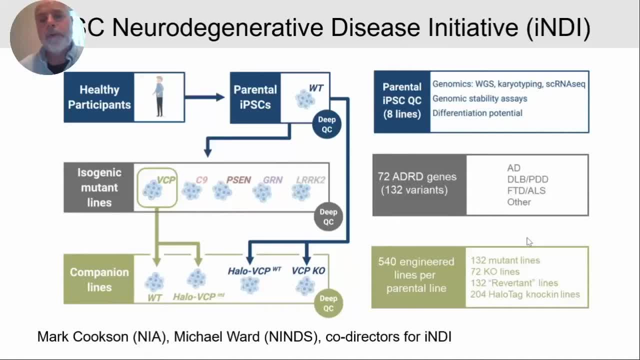 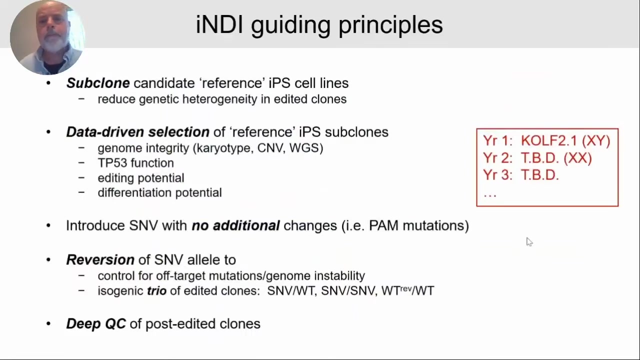 we'll also be making complete knockouts of each of these genes. So the research community will have a set of deeply characterized IPS cell lines of these, of these genotypes, for study, and the project is is quite ambitious. so we're proposing to generate over 500 engineered cell lines per year in this project. Now some of the guiding principles that 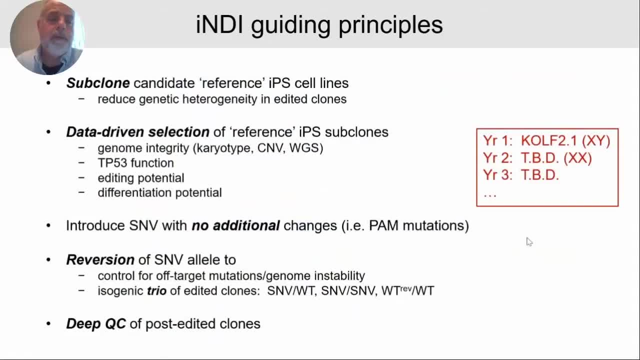 we came up with for the project- this was a discussion between Mark Cookson, Michael Ward, myself and other collaborators- is to really do this in a systematic and careful way. So the first principle is that we wanted to sub-clone the candidate reference IPS cell line, Even though 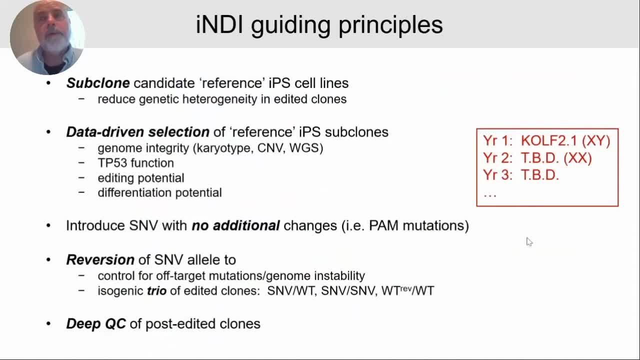 the IPS cell line is a clone in a dish when it's originally generated from a person, from an individual. there's a lot of work to be done to make sure that the cell line is in the right place. There's a lot of work to be done to make sure that the cell line is in the right place, So 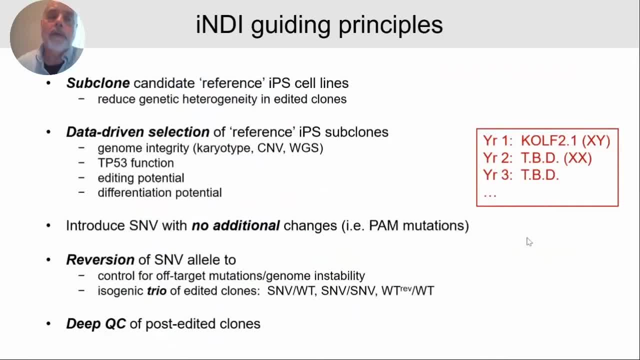 there's a lot of work to be done to make sure that the cell line is in the right place. There's often a chance that that cell line is not pure, that there could be genetic heterogeneity in that cell line, particularly if it's been cultured for a period of time. So when we start thinking about 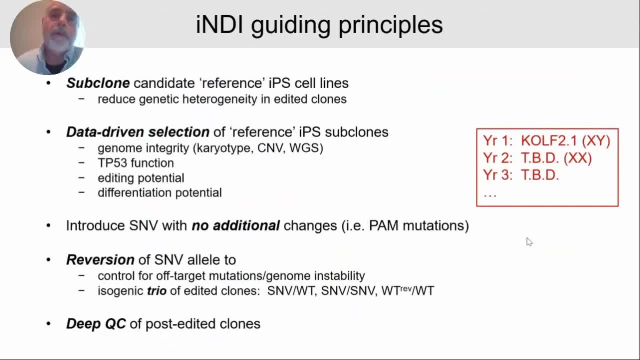 editing IPS cell lines, the first thing that we will do is isolate individual clones. So if there's any genetic heterogeneity in these starting cell population, that's going to segregate into the clones and that's going to confound the analysis of the phenotype. So the first step in all this is to 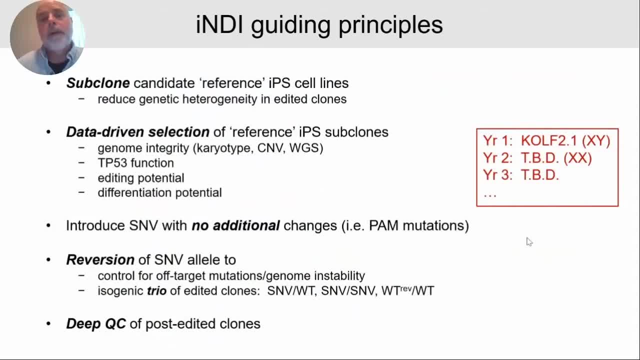 subclone candidate reference IPS cell lines, which we've done. We've actually screened subclones of eight different IPS cell lines from Northern European population for this first year of study, And then the next step was to use data-driven selection to identify the reference IPS subclone. 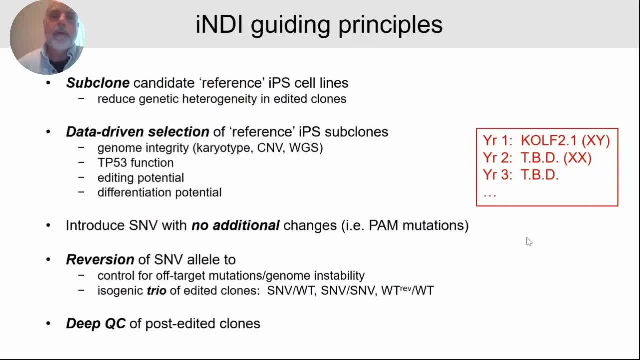 that will be used for each year of production. So this data includes genome integrity assays, the karyotype copy, number variation, even down to whole genome sequence. We assay for TP53 function. We look at their editing potential, differentiation potential, So that we've gone through this process. 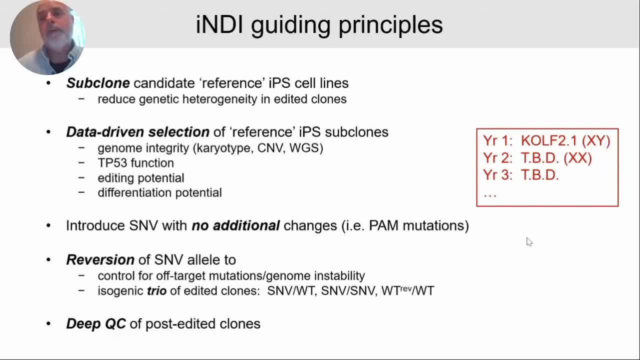 and for year one of production, we've identified a cell line called CULF2.1,, which is a male cell line, And then we will follow this year on year with different IPS cell lines. And for year two, we're going to repeat the same set of editing experiments in a female line, that's. 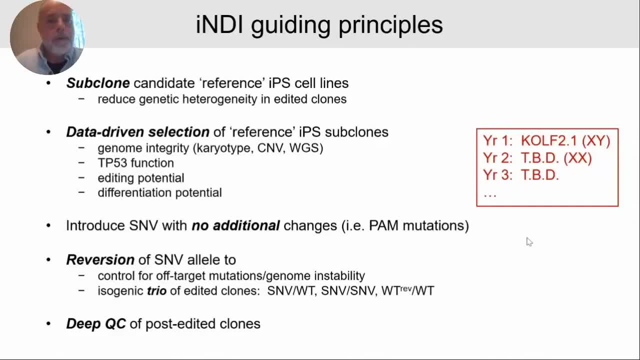 yet to be identified. So a third guiding principle is: we want to introduce only the SNV, the single nucleotide variant that is causative of disease, without adding any additional nucleotide variants. And one of the reasons why we add additional changes is to prevent. 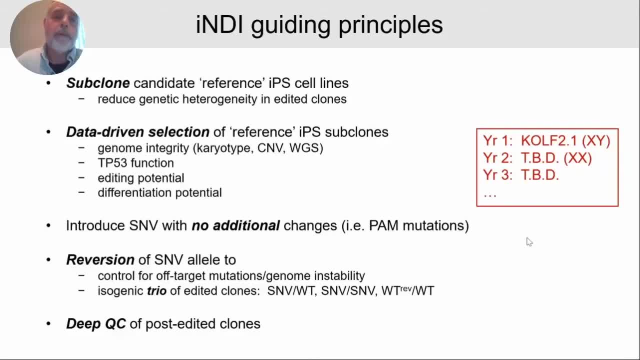 recutting of the LEO by Cas9. But for this project we want to make sure that we can revert this mutation. So we don't want to be adding any additional changes anyway. So we won't be adding PAM mutations, So we're just. 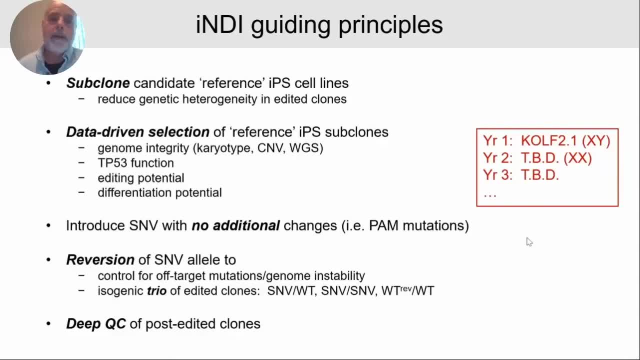 going to be introducing the single nucleotide variant And that then allows us to create reversions of these clones, So we can revert the SNV allele And, as I said earlier, this will control for any off-target mutations or genome instability that may have occurred during the. 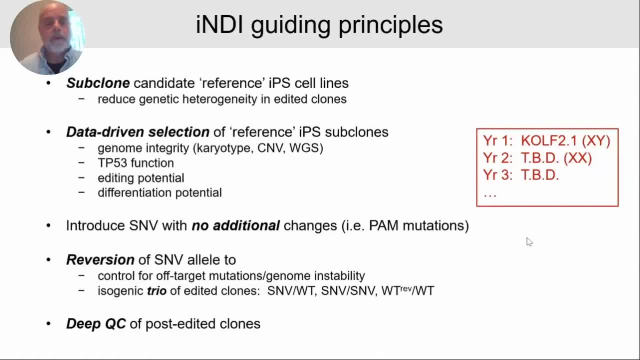 generation of the SNV clones, And so what we will be offering scientists will be an isogenic trio of clones, which includes the SNV in a heterozygous and a homozygous state, as well as the revertant of the heterozygous SNV clone back to wild type, And, finally, from lessons that we've learned over. 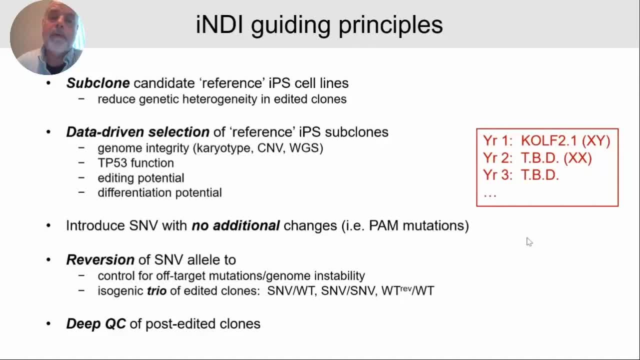 the past five, six years about CRISPR-Cas9 editing and just culturing of iPS cells is that we want to be careful that we do not select for abnormal clones, And so we're going to be executing deep quality control of post-edited clones before making them available. 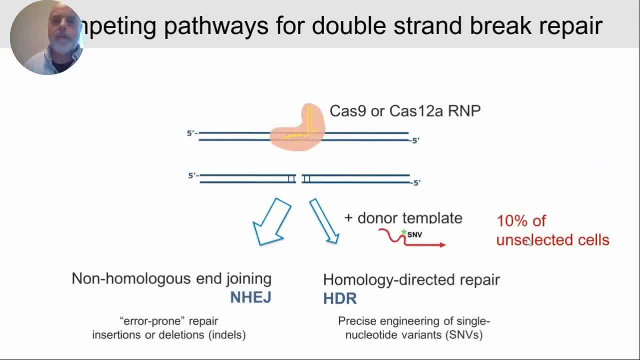 So let's just talk about the way in which we generate single nucleotide variants in human iPS cells. Of course, we use Cas9 or Cas12a programmable nucleases for this, and we're using them in the RNP format. This is the most efficient. 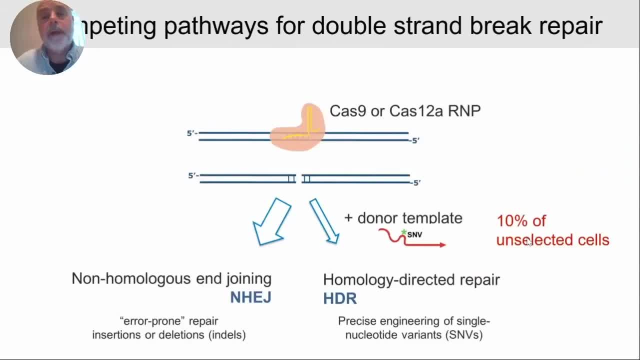 way to introduce Cas9 or Cas12a activity into iPS cells. So what happens is that you get a double stranded break and then we have two possible pathways for the repair of those double strand breaks. The dominant pathway in iPS cells is non-homologous end joining. This is where the two 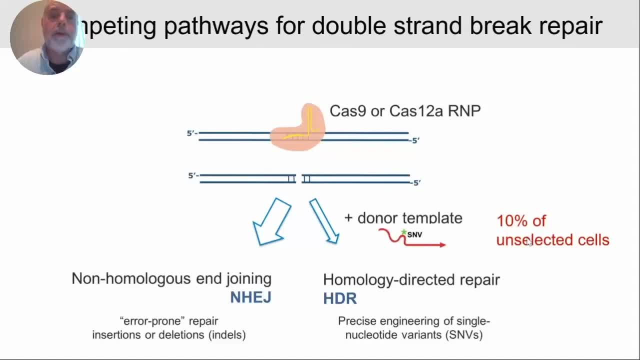 ends are brought together by NHEJ in an error-prone repair mechanism which often leads to a single nucleotide variant, And so we can also use the single nucleotide variant to introduce single nucleotide variants in the gene If we add a donor template which has 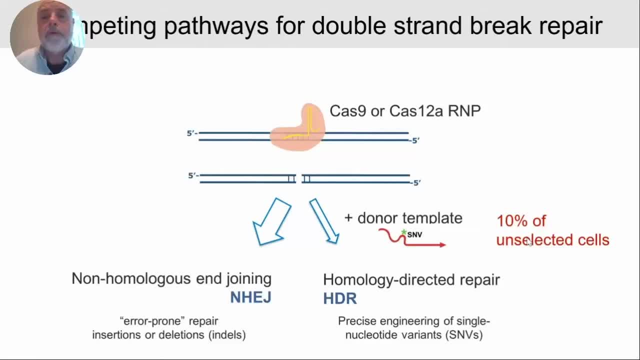 homology to this region around the breakpoint. we can also, with nucleotide precision, introduce single nucleotide variants using a simple oligonucleotide donor with a single base change. However, that's fairly inefficient. When we started this, even with Cas9 RNP delivery, we were getting. 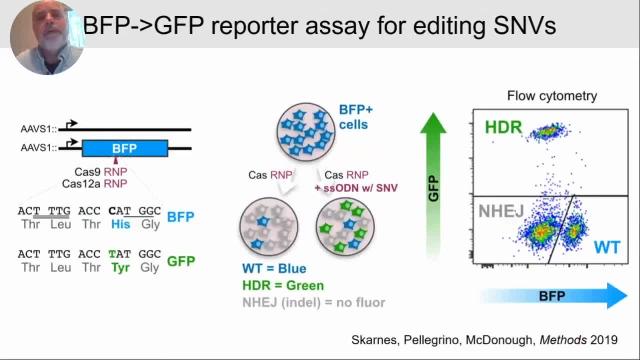 a single nucleotide variant with a single base change. So to improve this we developed a BFP-GFP reporter assay for editing SNVs. It's based on Jacob Korn's BFP-GFP assay But in this case we're looking at just making a single change, a C to T change, which changes the histidine and BFP. 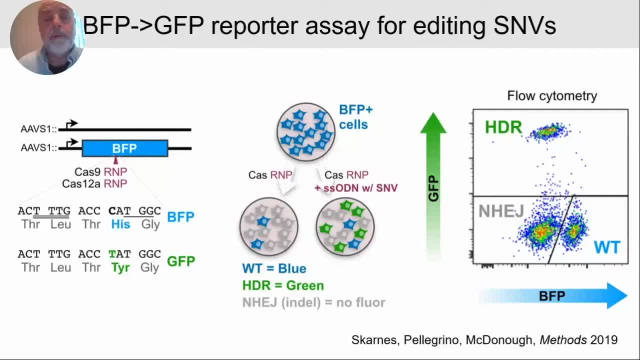 to a tyrosine residue which makes the protein fluoresce as a green fluorescent protein. So we go BFP to GFP with just a single base change. You can see here the C to T. And then we just run that through FACS after we allow the cells to recover And we can accurately 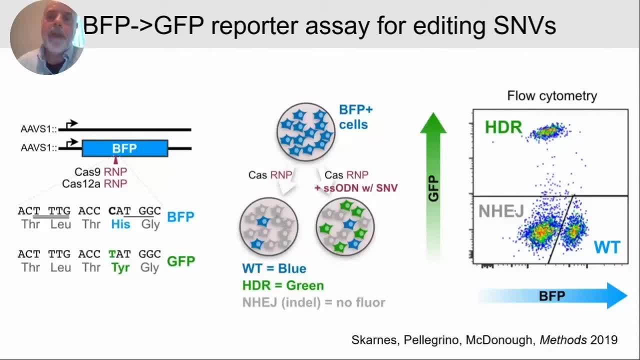 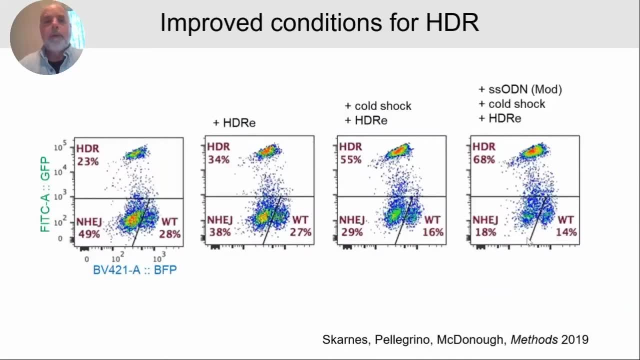 quantitate the amount of HDR, NHEJ and unedited alleles in this pool of cells. So we tested a bunch of different conditions and reagents over a period of two or three years And it really became clear that the BFP-GFP assay was the most effective way to test the BFP-GFP assay. 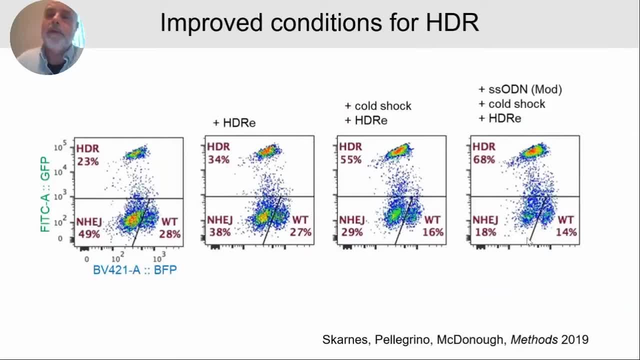 So we tested a bunch of different conditions and reagents over a period of two or three years And it really boils down to three different conditions which have made a significant effect on improving HDR efficiency. So the first is to add HDR enhancer. This is a small molecule which is a 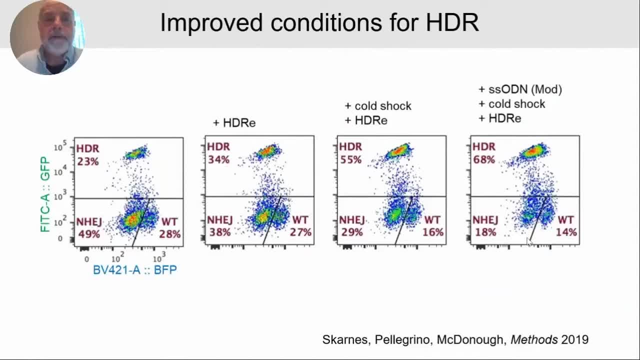 human ligase IV inhibitor And that's effective in promoting HDR. If we combine that with cold shock, we see even further improvement, up to 50% HDR efficiency. And then if we add a single-stranded oligonucleotide which has been modified at both ends, 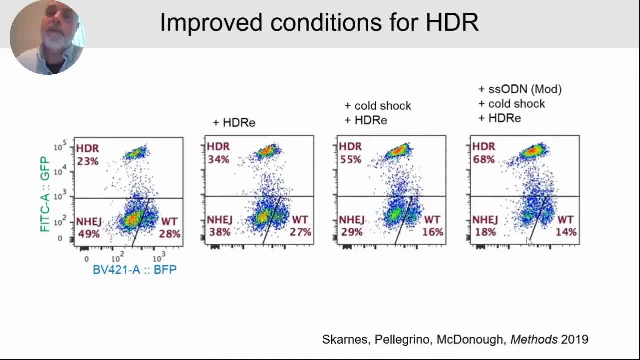 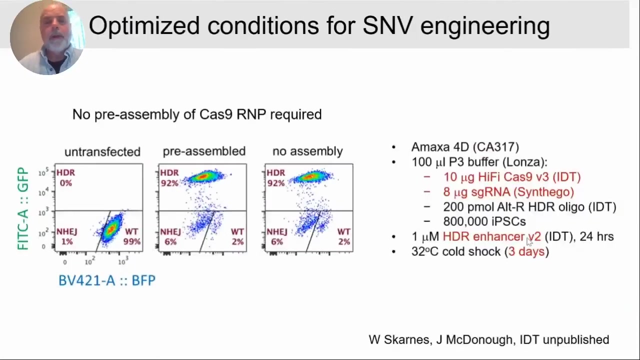 this is the product from IDT. we can get up to 70% HDR efficiency. So you can see, with just changes, these small changes in conditions, we can reverse this bias towards NHEJ in favor of HDR, And this was published last year in a methods paper And so 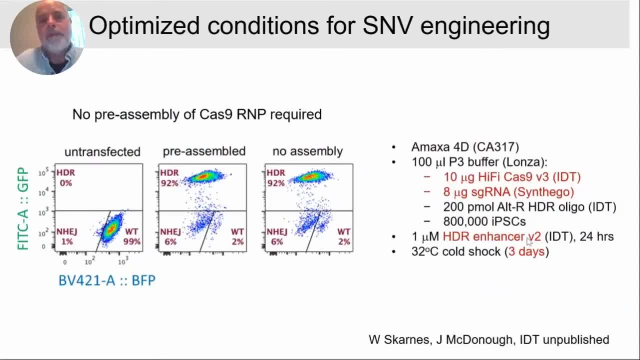 since then we've made a few more tweaks and optimized the conditions even further, So we've reduced the amount of Cas9 RNP that we add, We have substituted a new HDR enhancer called Version 2 from IDT, which should be commercially available soon, And we've extended cold shock to three days. 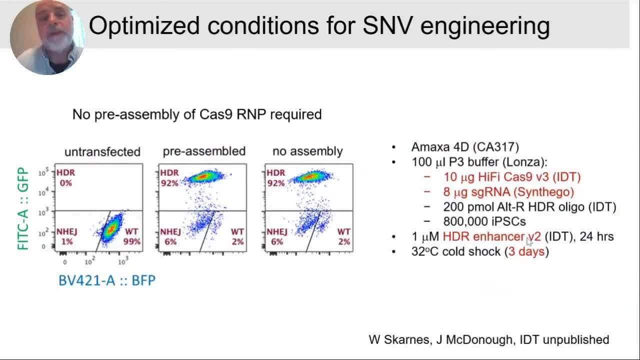 And you can see that we're now getting above 90% HDR efficiency, with very few unmodified alleles and very little NHEJ, Dr David Erickson PhD. So this is quite remarkable. Another very interesting result was to find that we don't. 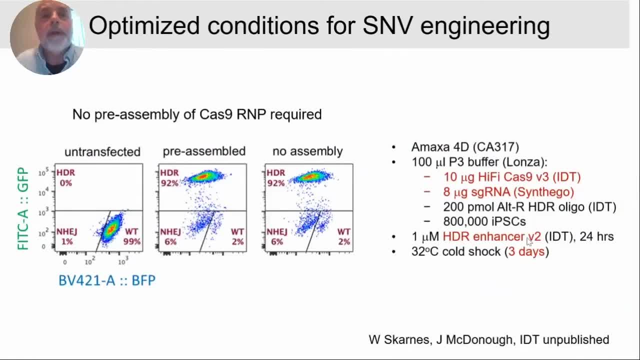 require a pre-assembly step of the Cas9 RNP. So initially we would add Cas9 protein and synthetic guide RNA together in a test tube and let it sit for an hour before doing the nucleofaction. But we find that we can actually add it directly to the nucleofaction with no time for assembly and 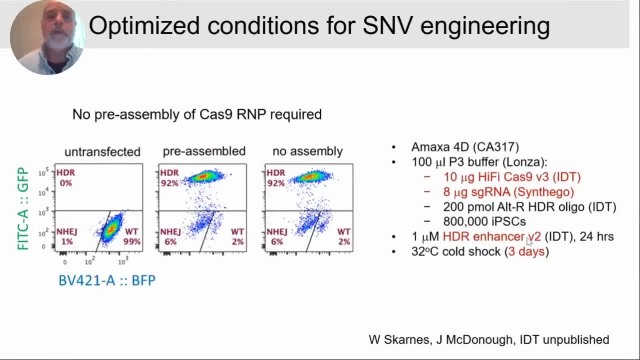 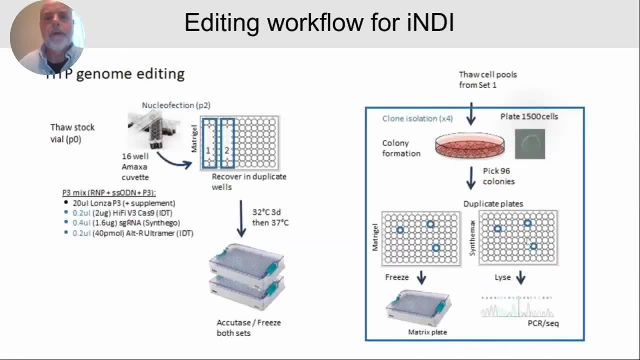 get similar results. So this is very convenient, Dr David Erickson PhD. And it shows you that this Cas9 RNP is actually getting assembled quite efficiently in the cell, Dr David Erickson PhD. So we have a very simple editing workflow for this project. So we're doing these nucleofactions now. 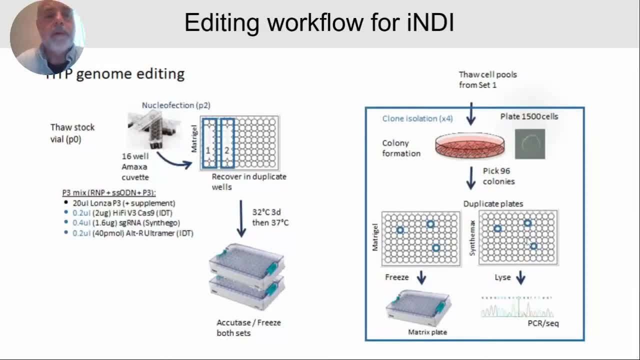 in parallel in small volumes in a 16-well maxi-cuvette. It's showing you the conditions that we use. So after nucleofaction we allow the cells to recover, then we freeze them away, Dr David Erickson, PhD, And at our leisure we can thaw these cell pools. Dr David Erickson PhD. as many as we need Dr David Erickson PhD, So we can thaw these cell pools. Dr David Erickson PhD. as many as we need Dr David Erickson PhD, So we can thaw these cell pools. 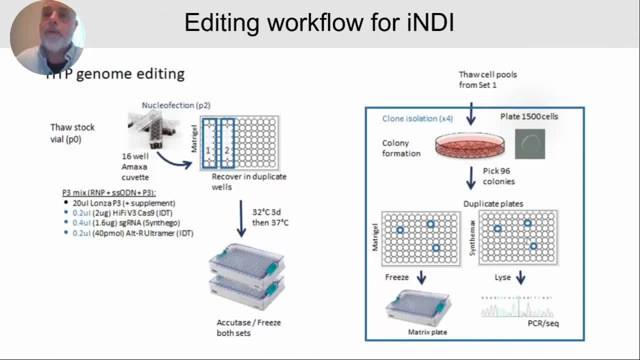 Dr David Erickson PhD, as many as we'd like in a week, And we would then do single cell cloning, which is essentially to plate a low number of cells onto a 10-centimeter dish. We would plate typically 1,500 cells and wait for colonies to appear and then pick those colonies. 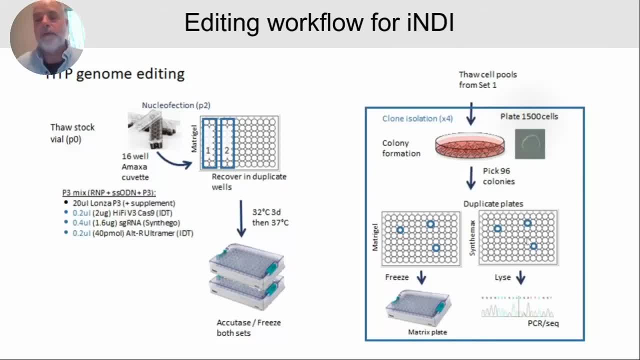 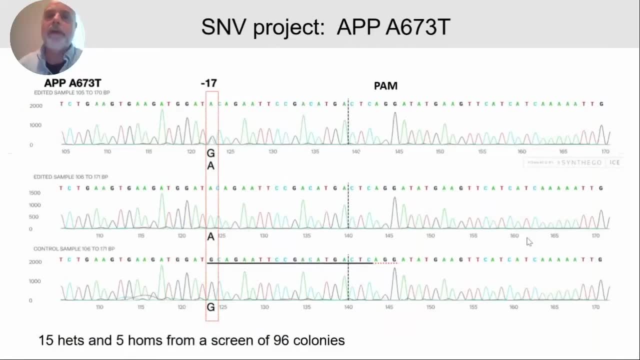 into duplicate plates- one which we freeze and one which we lyse- and genotype Dr David Erickson PhD. So here's an example. It's an impressive example of one of our first experiments using these optimized conditions. Dr David Erickson PhD. 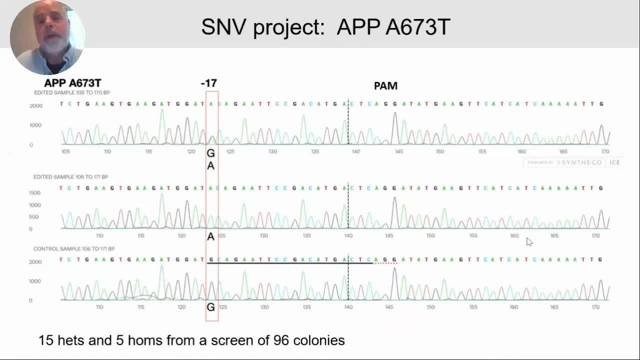 Where we were trying to make a single nucleotide change outside of the seed region for the guide RNAs. You can see here it's the last position of the guide or the first base of the guide sequence, And we were able to get plenty of heterozygote and 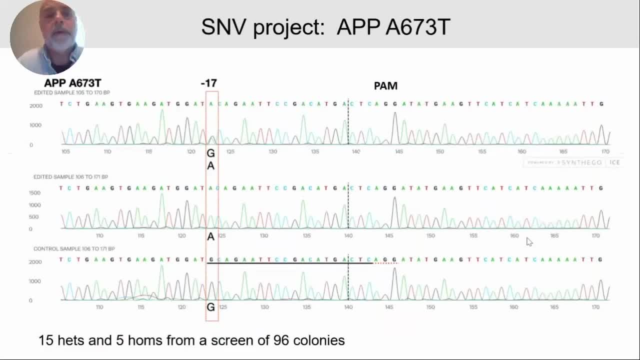 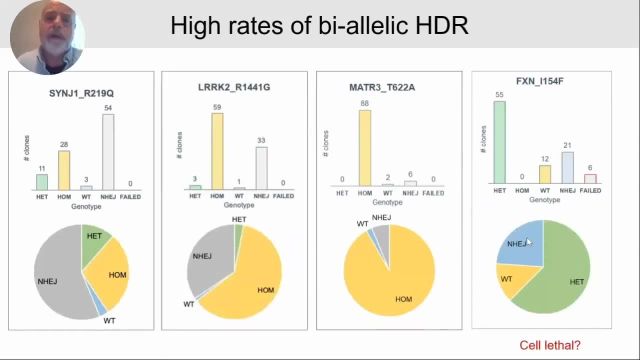 homozygote clones from a screen of 96, even with a single nucleotide change in this position, Dr David Erickson, PhD. So we've now done over 70 of these experiments and we have genotyping data for these now. And 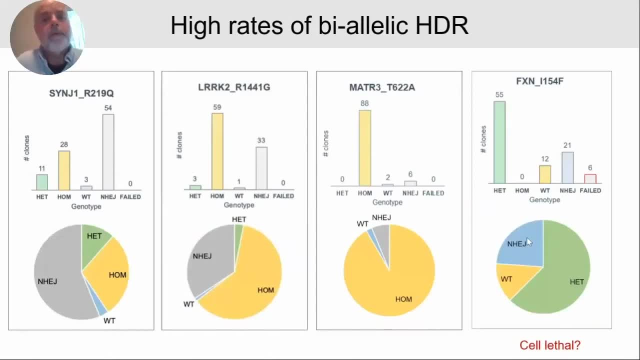 this is typical results that we're seeing, which are quite remarkable. So, on the left, about a third of the experiments are giving us a good number of heterozygotes and homozygotes, SNV clones, But about two thirds- these are the two panels in the middle. 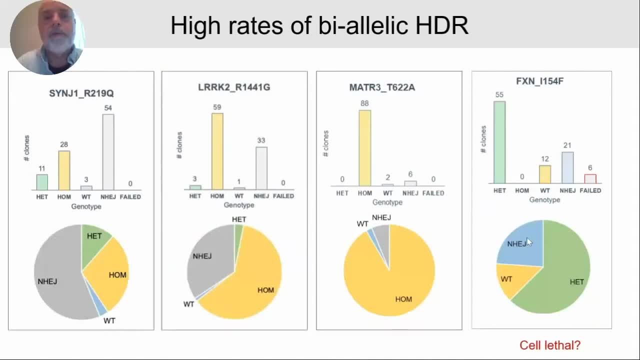 you can see, are giving us an overwhelming number of homozygotes, with very few heterozygotes, clones, And we believe that's because the efficiency of editing is so high that there are very few wild type or unedited alleles left in cells. 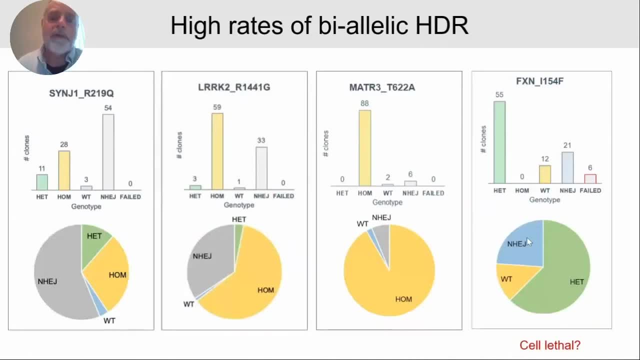 so we don't get heterozygote clones. So by optimizing these conditions, we've actually created a problem for ourselves. We're not getting the genotypes that we want for many of these experiments, which are heterozygote clones. We're getting plenty of homozygotes. 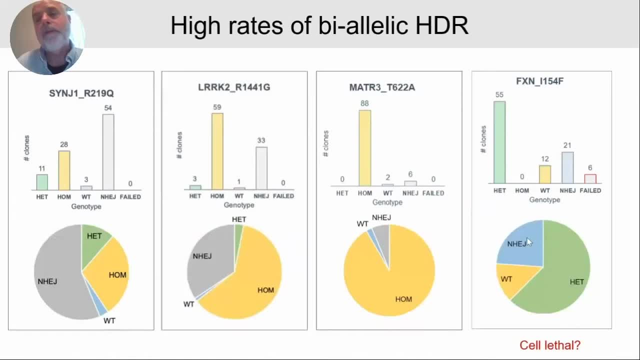 but not enough heads. Dr David Erickson, PhD. The example in the far right is actually interesting because it looks like that this is a gene which is essential in human iPS cells, because we're not able to get- and I'm not saying that we're not going to get- a gene that's essential in human iPS cells. 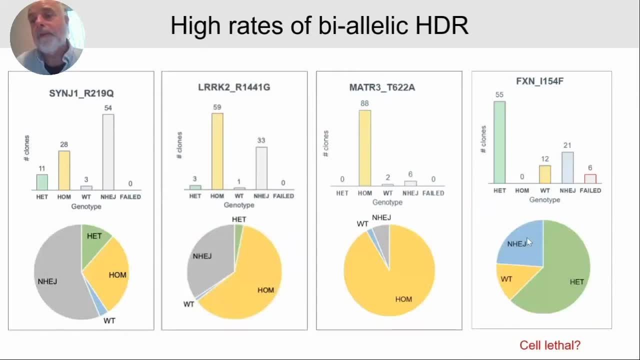 but we're going to get a gene that's essential in human iPS cells, because we're not able to get any homozygote clones but we get a huge number of heterozygotes clones. So that's an indication we think of a cell-lethal phenotype, But fortunately these are rare among the 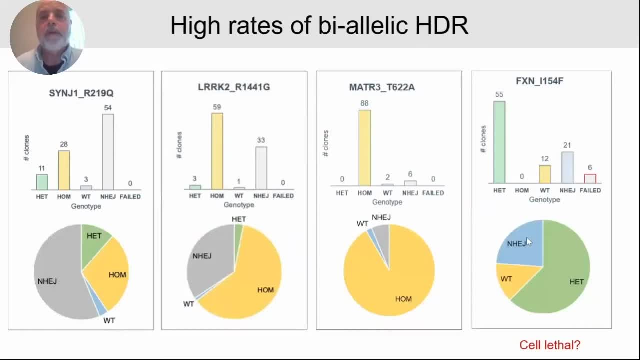 genes that we are targeting currently Dr David Erickson, PhD. Okay, So how do we deal with this problem of getting too high of an editing, too high rate of biallelic editing of cells? So what we want to do is be able to control the zygosity. 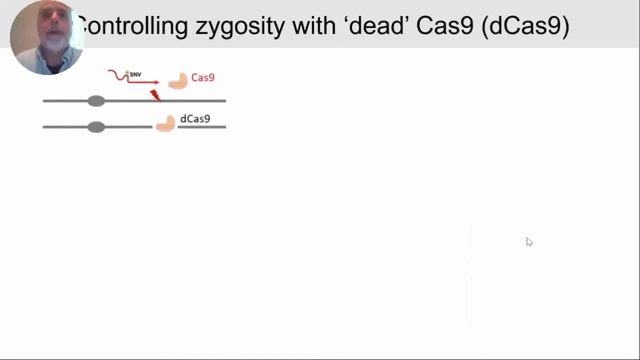 of the cells that come out of editing. So we want to control the outcome in cells And we've managed to do this with a very simple trick, which is to add dead Cas9 to the nucleofection. So the idea is very simple: If we have a mixture of Cas9 and 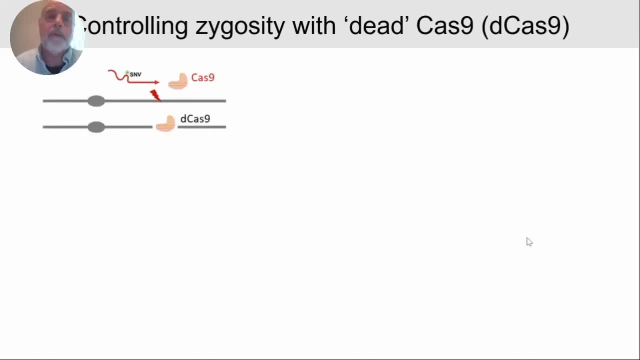 dead Cas9 in the nucleofection. we would expect the dead Cas9 will bind at some frequency to the target site, but it won't cleave that target site. It will just sit there and block it from getting cleaved by active Cas9.. Dr David Erickson, PhD. 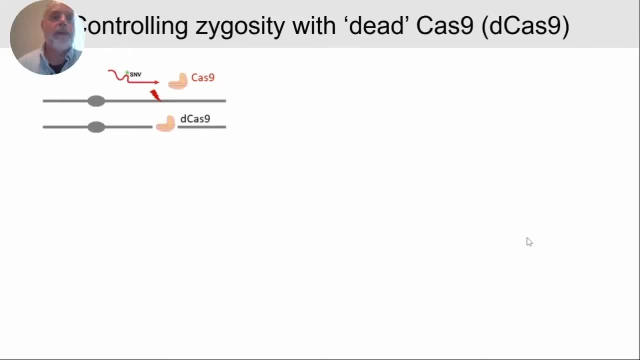 And on the other chromosome, active Cas9, we'll go ahead and make the break and we'll get the SNV And this seems to work quite well. using the BFPGFP assay, Again we can see that if we mix Cas9 and dCas9 together at a one to four ratio, we can really shift. 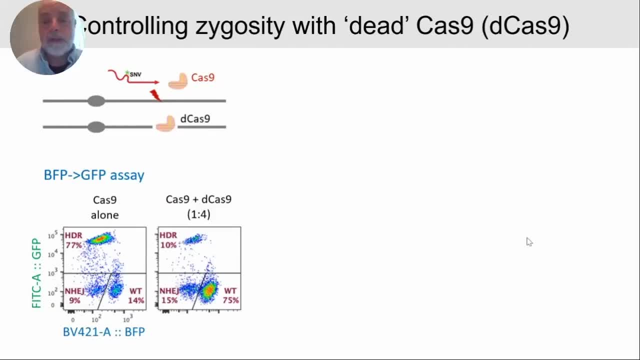 the balance of alleles from HDR back to wild type. So we've carried out a pilot experiment where we took several of these examples, where we got overwhelming numbers of homozygous HDR And we just added in increasing amounts of Cas9 and dCas9. And you can see very clearly how. 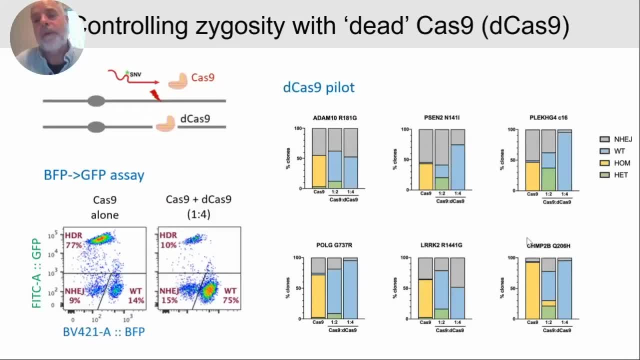 we can change the zygosity of the clones that come from these experiments. One in four gets us almost entirely wild type again, whereas a one in two intermediate amount of Cas9- dCas9,. we're starting to see a good number of heterozygous clones, So we're following. 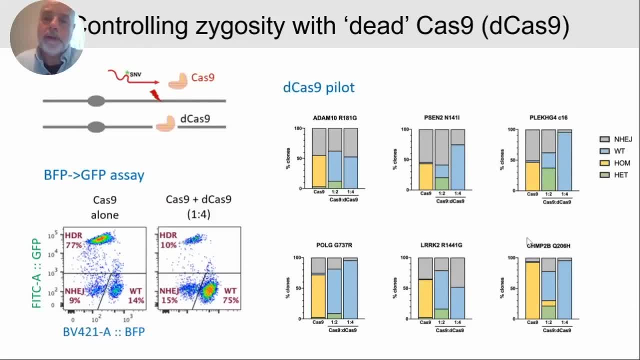 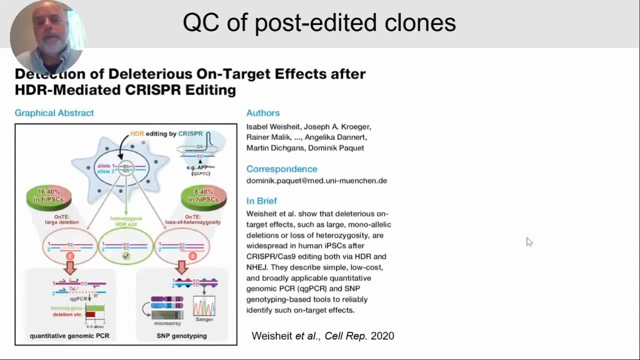 this up now with trying to test even slightly lower concentrations of dCas9 to see if we can find conditions that give us a good mixture of heterozygous and homozygous clones. So this year a very important paper was published by Dominic Paquet. 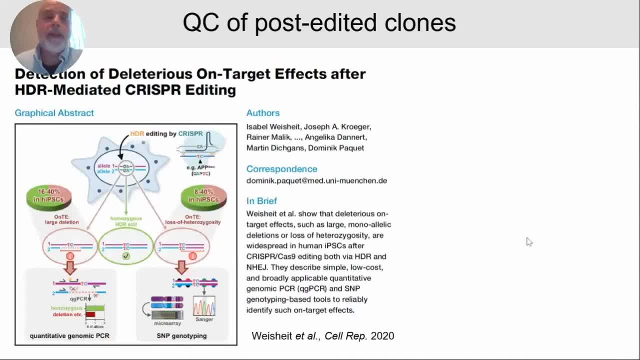 who looked very carefully at iPS cells that have been edited to find that there's quite a lot of on-target effects that are occurring in edited iPS cell clones, And what they documented was up to 40% of the iPS cell clones had deletions of one copy of the gene or one region around the. 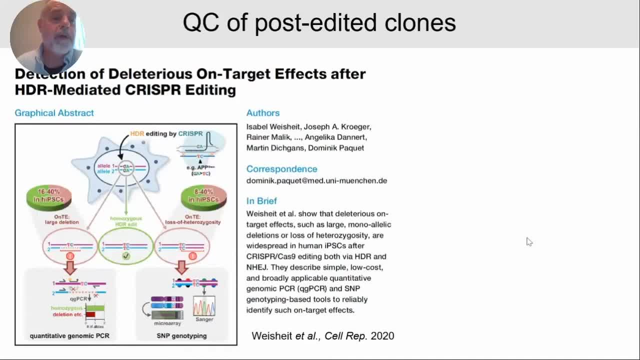 target site on one chromosome. That's a problem, because then you end up with a mutated gene on one chromosome and your SNV on the other. The second problem is that they saw copy-neutral loss of heterozygosity. So what happens is your double-stranded break induces loss of. 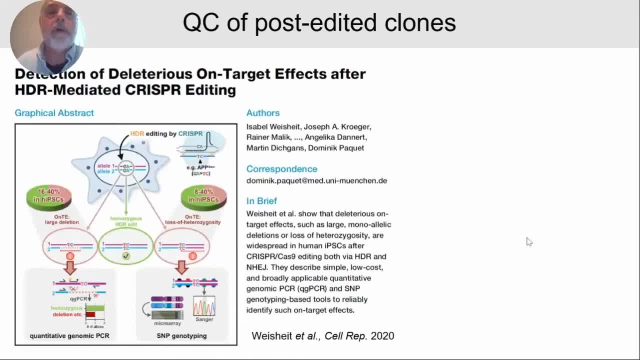 heterozygosity, which can extend for megabases, яет a lot of the energy that goes down downstream of the target to the end of the chromosome. So these are events that we really want to avoid. So for the INDIE project, we're going to 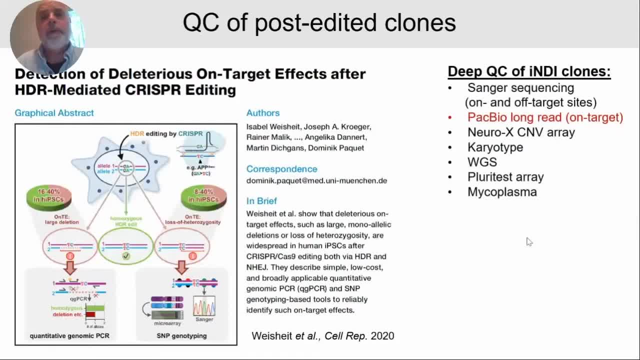 run many assays to make sure that these post-edited clones are normal. So we'll start with Sanger, sequencing it both on and off-target sites, And then we'll use PacBio long-read technology to look for these problems of on-target effects where we might have a deletion of theInstante. 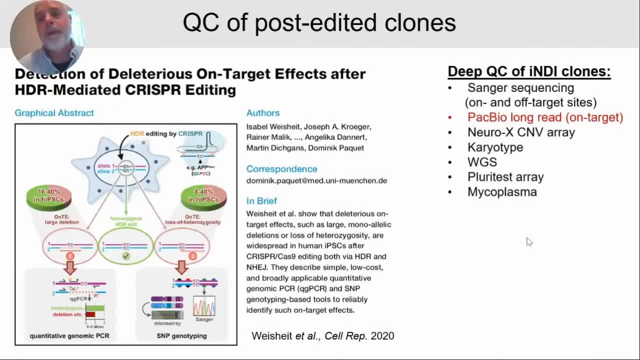 or we might have loss of heterozygosity. we'll also be looking at copy number variation within the clone. we'll carry, type it to whole genome sequence and flurry test in micro plasma. so these clones are going to be very carefully QC'd and we'd be able to add to the information on what happens to IPS. 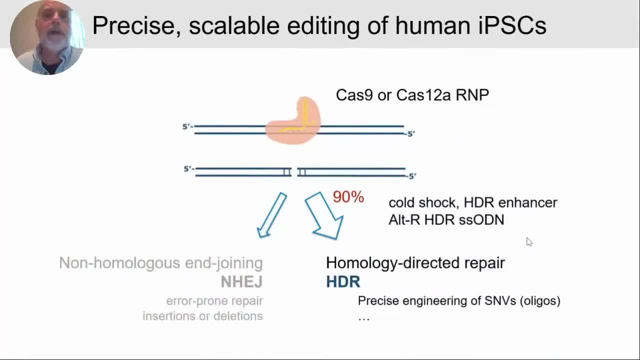 clones after editing. so, to summarize, I think we have developed very efficient and precise methods for editing human IPS cells, which is which is scalable, so we can actually start to think now about generating genome-wide collections of IPS cell lines with various kinds of alleles. the first kind of allele that we're 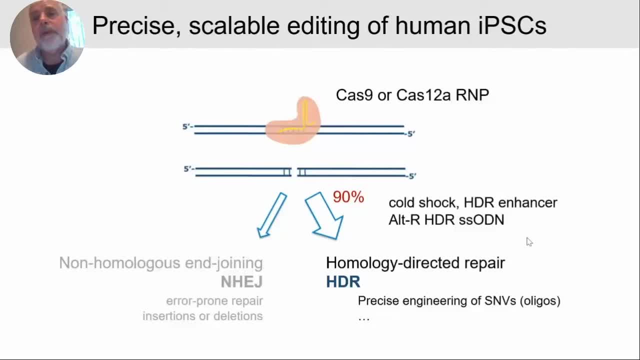 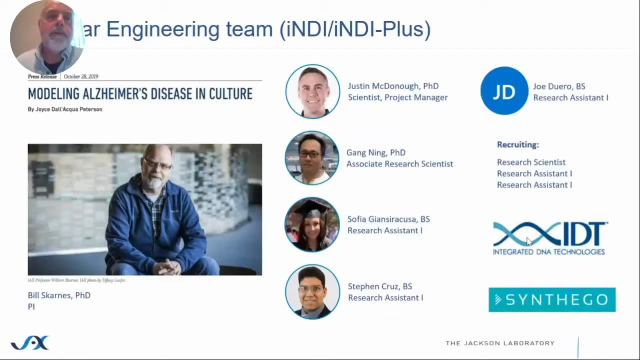 starting with is a simple one- SNVs- but we might be able to use these. we expect we'll be able to use these conditions and technologies to generate other, more complex alleles in the future. so let me just introduce you to the people who have helped with this project. 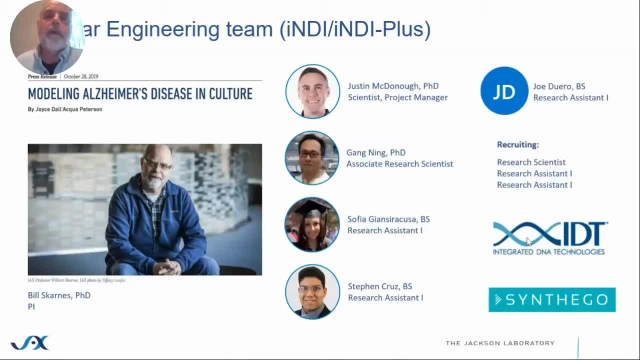 most importantly, Justin McDonough, who is the project manager for Indy- he also runs the core in cell editing service at the JAX GM- and a number of talented research scientists and technicians, and- and we're currently expanding this to include additional research assistants and scientists. I also really want to 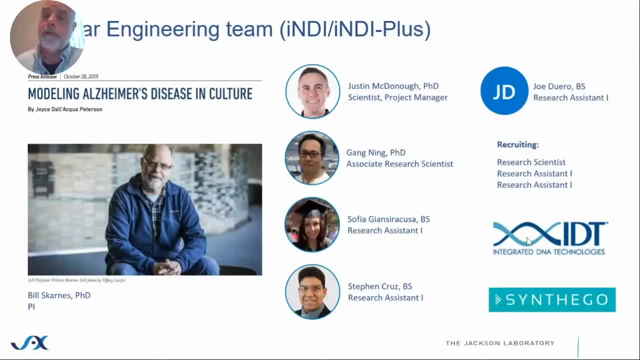 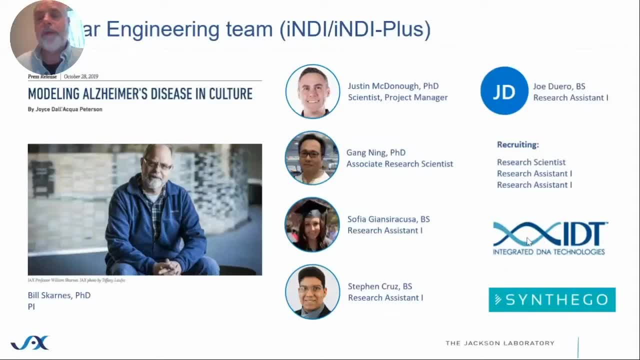 so new, new reagents with us as they, as they develop them at IDT, which includes the HDR enhancer in the end blocked oligonucleotides, which made it make a big difference, and, of course, citizen ago who have provided us with these very effective synthetic guide RNA is for this research. so with that I'll stop and 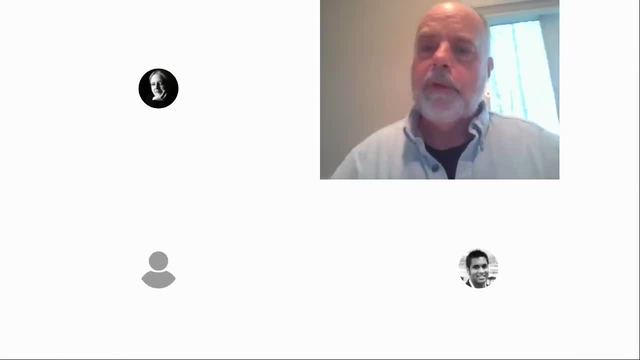 take questions. one question from James Cooper is: how difficult is it to edit a cell line introducing SNVs only without mutations to the PAM? Well, initially we thought this might be a problem because if you're just making a single nucleotide change in your target sequence, that's just a one base. 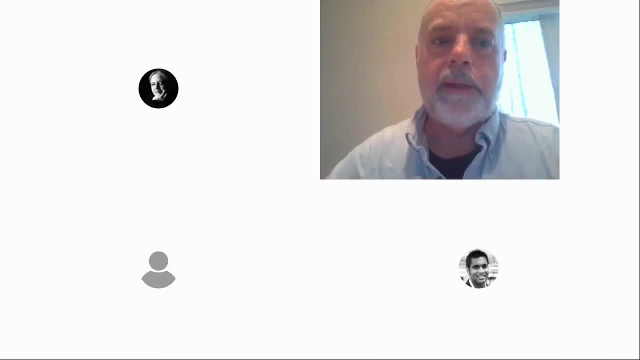 difference to the guide RNA And so you might expect that you would get that guide RNA coming back and re-cleaving the modified allele and inducing damage in that modified allele. But because we're using Cas9 RNP and we are limiting the amounts that we put into cells, 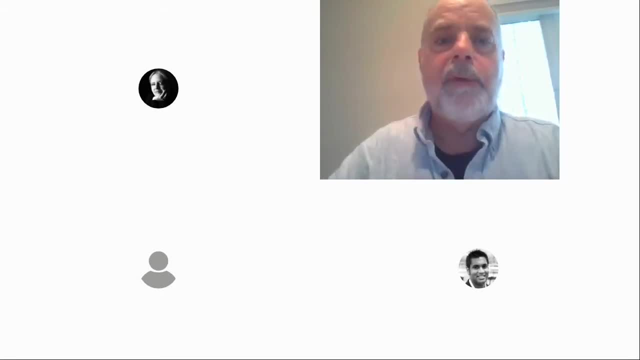 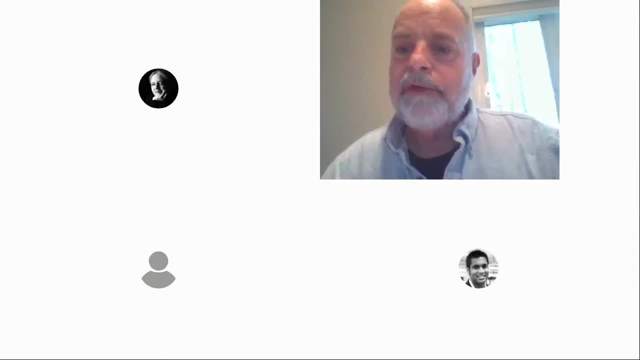 But that was a little bit of a surprise. So do you see any issues with genome integrity in your second step data-driven selection of reference IPS cell lines? So I think, second step, data-driven selection, So yes. so in selecting the cell lines, there were eight candidate lines. There were. 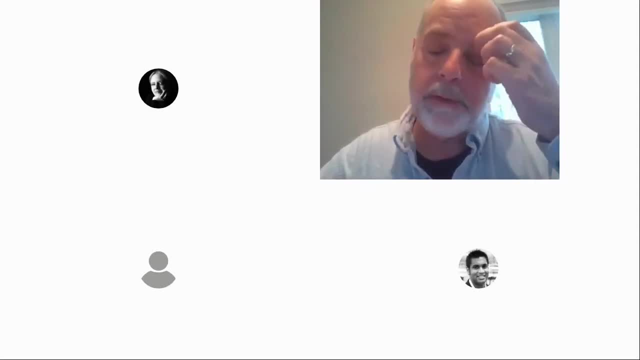 issues with some of the lines in terms of the array data, the copy number variation that we observed. they were all pretty well characterized to begin with so they were all charitably normal. so there were some subtle problems that were detected in the in the other cell lines and only one of the 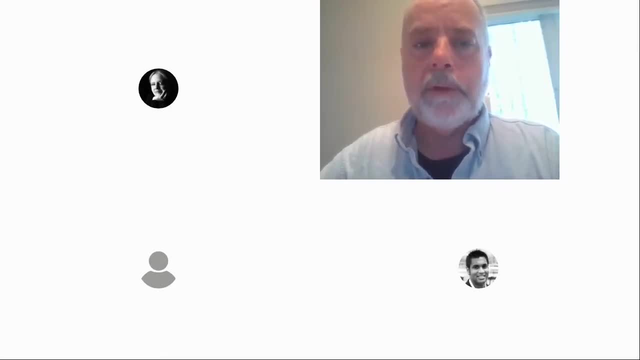 cell lines that we tested met all of the criteria, and that was the call of 2.1 cells that we're now using for for for the first year of production. so yes, there are differences that you find, even between well characterized, normal IPS cell lines. okay, I think we're one last question and then I 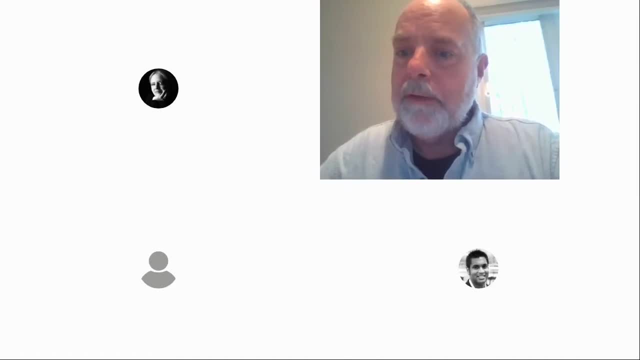 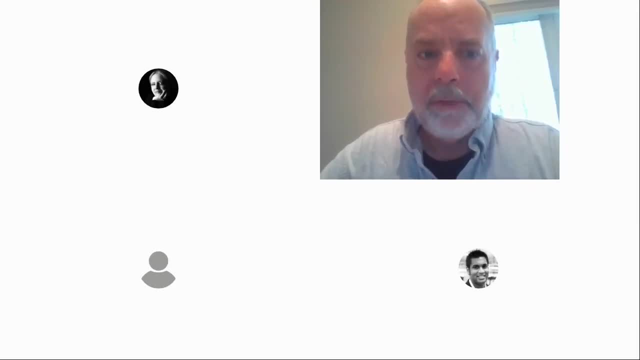 we could use base editors for this, but at we could use base editors for this, but at the moment we don't have recombinant, the moment we don't have recombinant, the moment we don't have recombinant protein base editing technology, we don't. 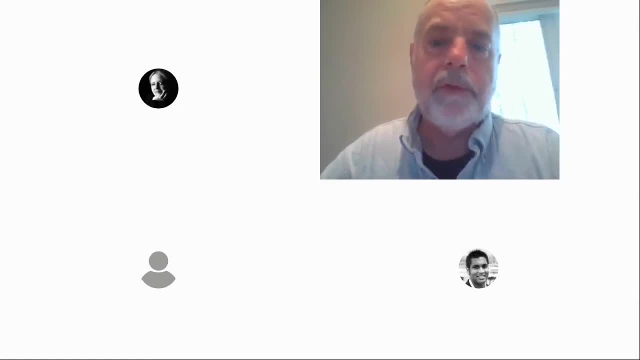 protein base editing technology. we don't protein base editing technology. we don't have access to recombinant protein. we have access to recombinant protein. we have access to recombinant protein. we might be able to use mRNA. it's something. might be able to use mRNA. it's something. 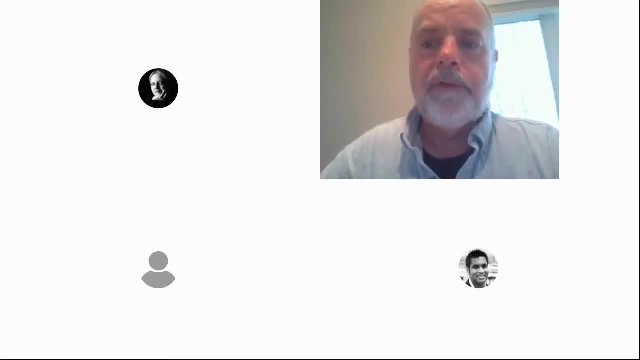 might be able to use mRNA. it's something that we are continuing to keep an eye on. that we are continuing to keep an eye on that. we are continuing to keep an eye on, because it could be even safer way to. because it could be even safer way to. 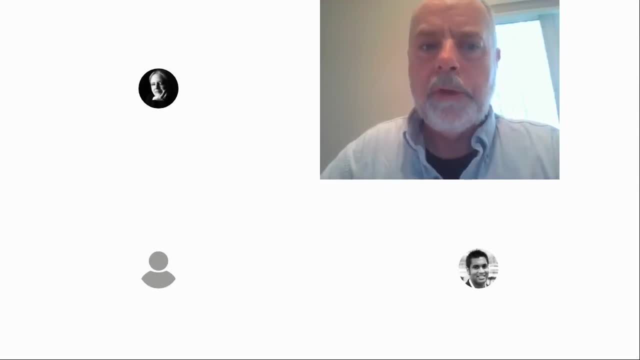 because it could be even safer way to introduce a single nucleotide changes. introduce a single nucleotide changes. introduce a single nucleotide changes into cells without having to worry about into cells, without having to worry about into cells, without having to worry about the effects of making double-stranded. 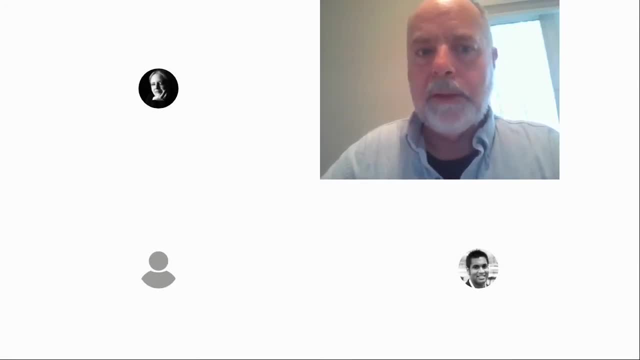 the effects of making double-stranded, the effects of making double-stranded breaks, I would say though that for some breaks, I would say though that for some breaks, I would say though that for some of the other leels that we want to make, of the other leels that we want to make, 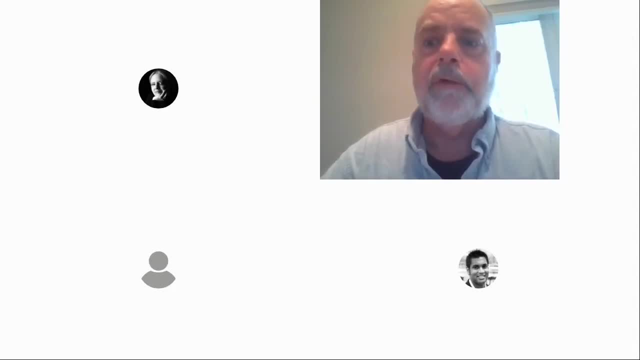 of the other leels that we want to make, like knock-in of halo tags and so on. we like knock-in of halo tags and so on. we like knock-in of halo tags and so on. we can't use base editors, so I think for. can't use base editors, so I think for. 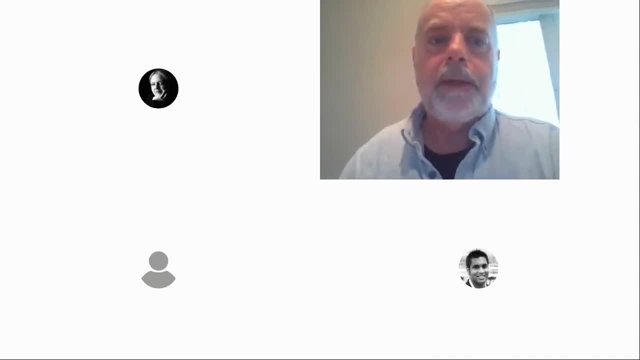 can't use base editors. so I think for those applications, we will stick with those applications. we will stick with those applications. we will stick with the cast 9 endonuclease technology. okay, the cast 9 endonuclease technology. okay, the cast 9 endonuclease technology, okay. so let me now turn it over to Chris. 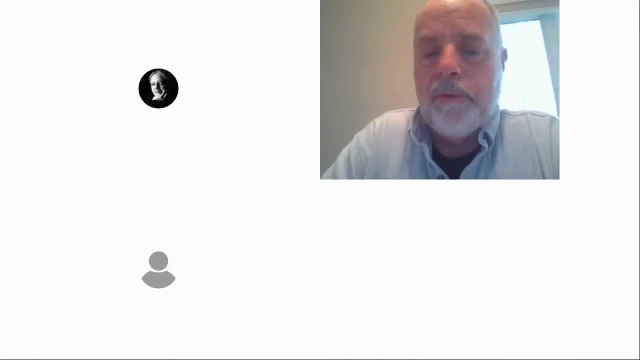 so let me now turn it over to Chris. so let me now turn it over to Chris. Saha Chris is an associate professor at Saha. Chris is an associate professor at Saha Chris is an associate professor at the University of Wisconsin in Madison. the University of Wisconsin in Madison. 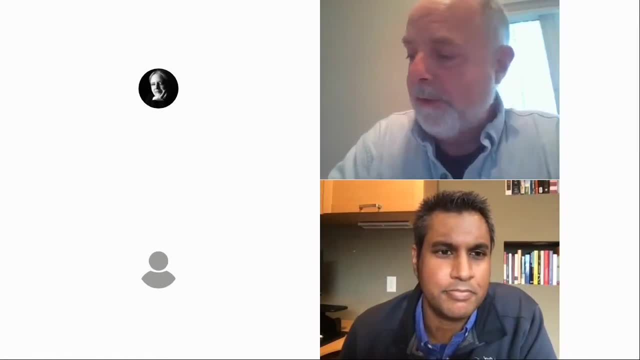 the University of Wisconsin in Madison and he's going to tell us a very and he's going to tell us a very and he's going to tell us a very interesting story about how we can use interesting story about how we can use interesting story about how we can use patient-derived IPS cells for for. 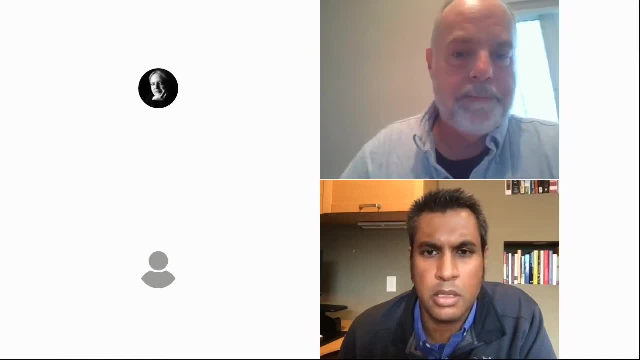 patient-derived IPS cells for for. patient-derived IPS cells for for therapeutics: Chris, over to you all. therapeutics, Chris, over to you all. therapeutics, Chris, over to you all. right, first of all, it's fantastic to be right. first of all, it's fantastic to be. 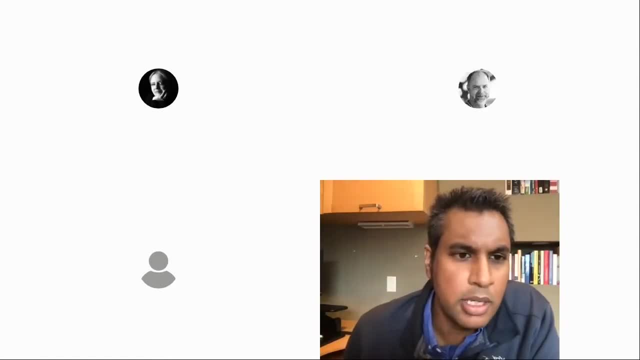 right, first of all, it's fantastic to be here. that was a really exciting story here. that was a really exciting story here. that was a really exciting story that we just heard and I think, well, my, that we just heard, and I think, well, my, that we just heard, and I think, well, my lab is building upon that. so I'm, I'm. 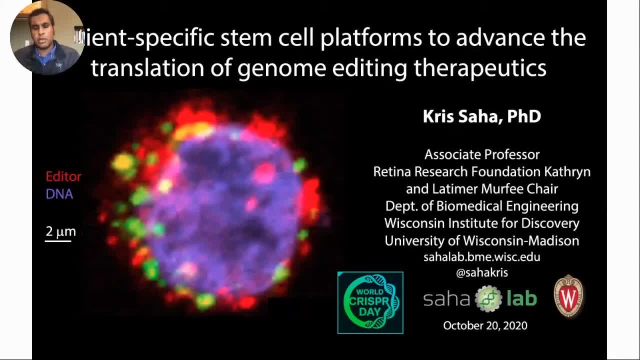 lab is building upon that, so I'm, I'm- lab is building upon that, so I'm, I'm here in Madison Wisconsin and would like here in Madison Wisconsin, and would like here in Madison Wisconsin and would like to tell you about how we're using, to tell you about how we're using. 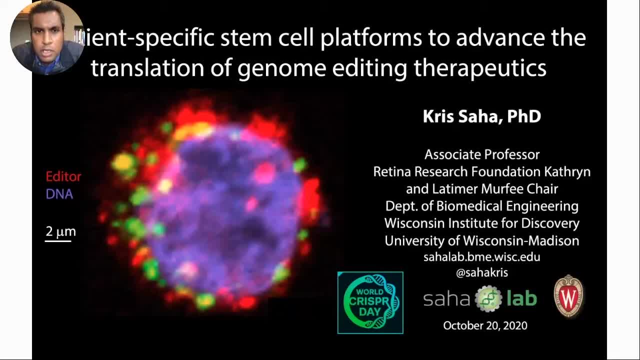 to tell you about how we're using patient-specific cell lines- IPS lines to patient-specific cell lines, IPS lines to patient-specific cell lines, IPS lines to make functional tissues to test genome. make functional tissues to test genome. make functional tissues to test genome, editors and potential candidate genome. 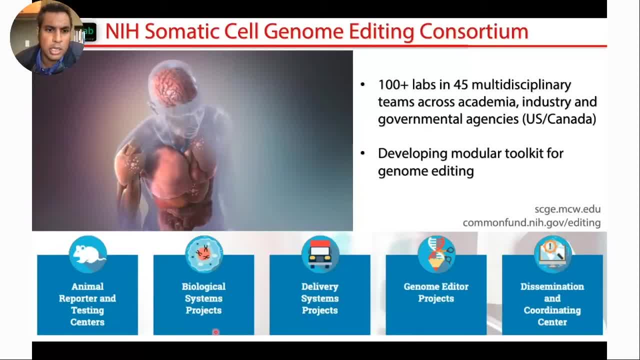 editors and potential candidate genome editors and potential candidate genome editing therapeutics and some of this editing therapeutics and some of this editing therapeutics and some of this work is really inspired by a larger work is really inspired by a larger work is really inspired by a larger consortium that I'm helping to lead is 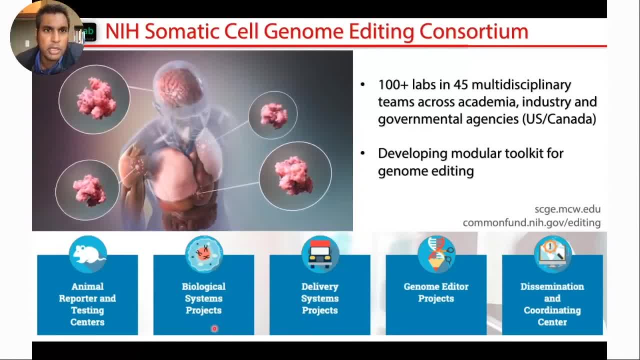 consortium that I'm helping to lead is consortium that I'm helping to lead is funded in the US by the National, funded in the US by the National, funded in the US by the National Institutes of Health, and it's called the Institutes of Health and it's called the. 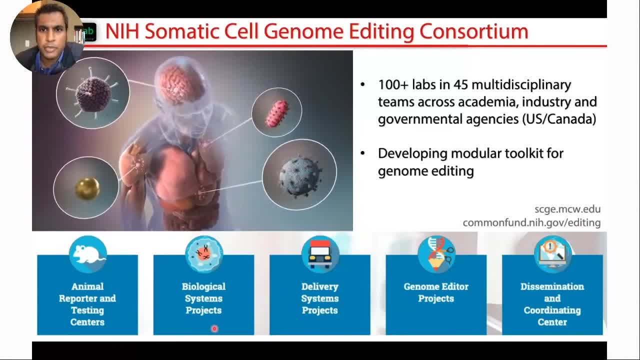 Institutes of Health and it's called the somatic cell genome editing consortium, somatic cell genome editing consortium, somatic cell genome editing consortium. it's fairly large effort that is trying. it's fairly large effort that is trying. it's fairly large effort that is trying to develop a modular toolkit such that 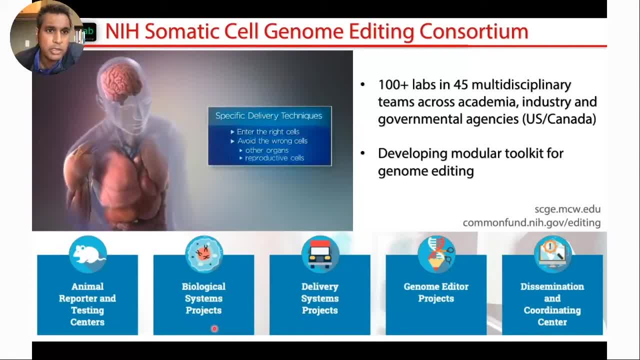 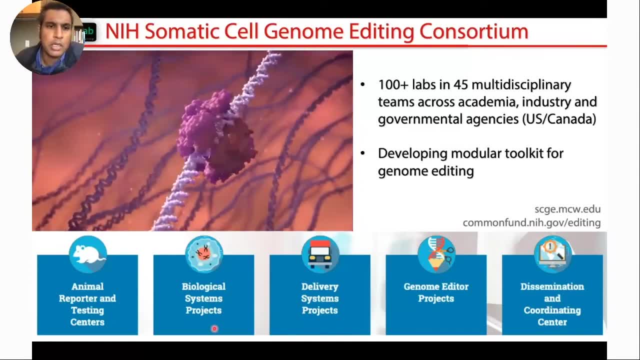 to develop a modular toolkit such that to develop a modular toolkit such that you can deliver editors into the body to you can deliver editors into the body to you can deliver editors into the body to directly edit endogenous alleles, that directly edit endogenous alleles, that directly edit endogenous alleles. that may be problematic and so the kind of 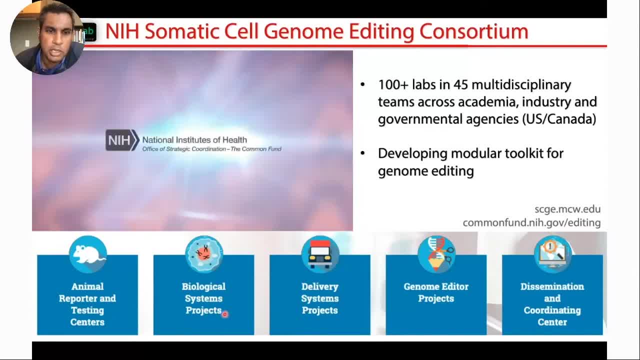 may be problematic and so the kind of may be problematic and so the kind of major initiatives are shown at. the major initiatives are shown at. the major initiatives are shown at the bottom here and the video is kind of bottom here. and the video is kind of bottom here and the video is kind of going through different areas of 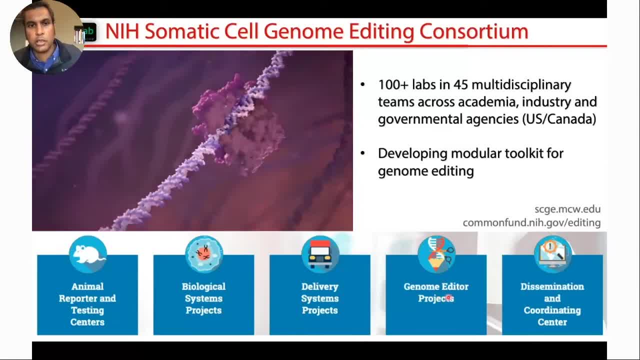 going through different areas of going through different areas of emphasis. so certainly we're emphasis, so certainly we're emphasis, so certainly we're working on new editors, base editors, working on new editors, base editors, working on new editors, base editors, mitochondrial editors, to kind of mitochondrial editors, to kind of. 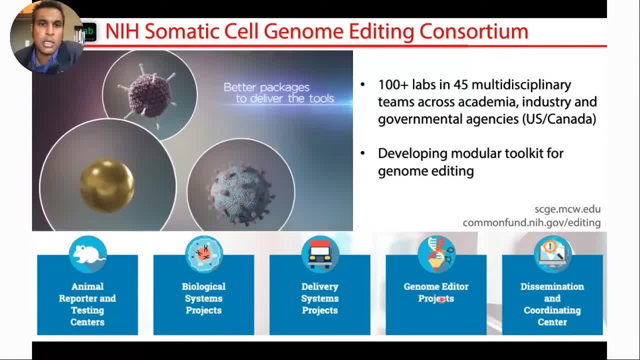 mitochondrial editors to kind of diversify the types of edits that we can. diversify the types of edits that we can diversify the types of edits that we can make both DNA, RNA and other nucleic. make both DNA RNA and other nucleic. make both DNA, RNA and other nucleic acids in the cell. what I'll be focusing 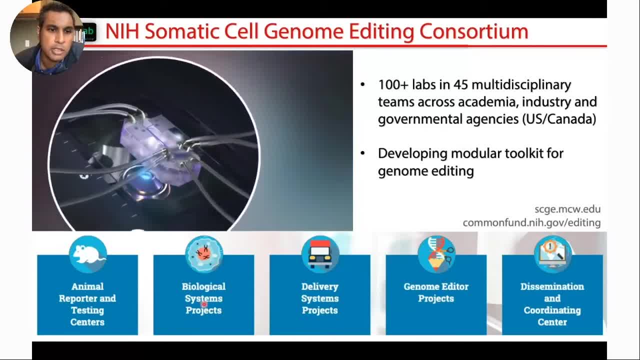 acids in the cell. what I'll be focusing: acids in the cell. what I'll be focusing on here is what you see in the video on here is what you see in the video on. here is what you see in the video, which is new biological systems, namely: 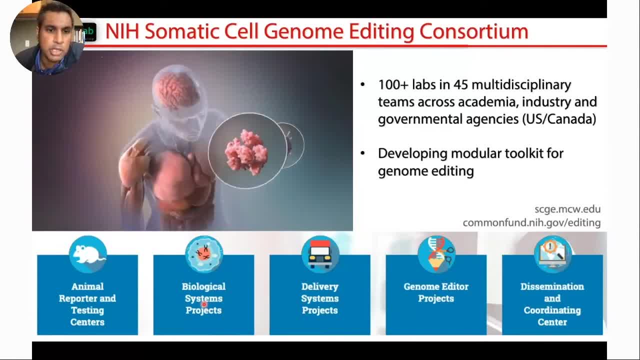 which is new biological systems, namely which is new biological systems, namely human biological systems that we can, human biological systems that we can, human biological systems that we can engineer using stem cell bioengineering, engineer using stem cell bioengineering, engineer using stem cell bioengineering, and a number of the projects use human 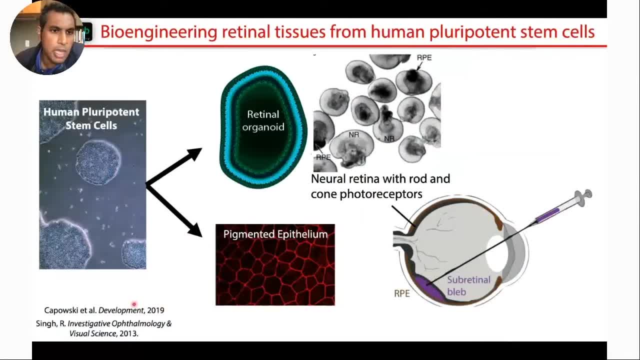 and a number of the projects use human and a number of the projects use human pluripotent stem cells. that you just pluripotent stem cells, that you just pluripotent stem cells. that you just heard about as essentially the raw, heard about as essentially the raw. 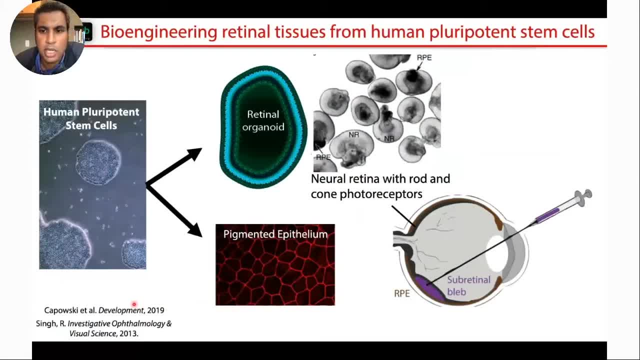 heard about as essentially the raw substrate to engineer various tissues, substrate to engineer various tissues, substrate to engineer various tissues. and today I'll give you a focus story. and today I'll give you a focus story. and today I'll give you a focus story about tissues of the eye and with our 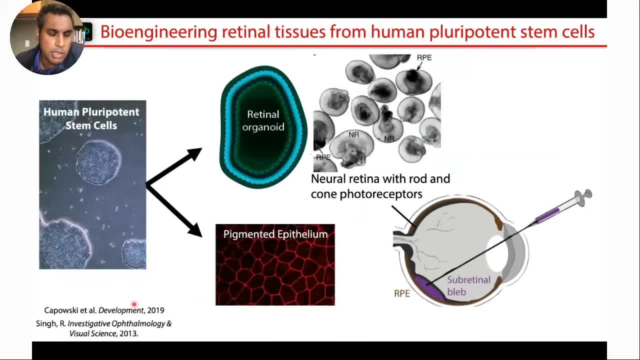 about tissues of the eye and with our about tissues of the eye and with our team here at Wisconsin, namely David Gans team here at Wisconsin, namely David Gans team here at Wisconsin, namely David Gans lab, who's pioneered some of the lab, who's pioneered some of the 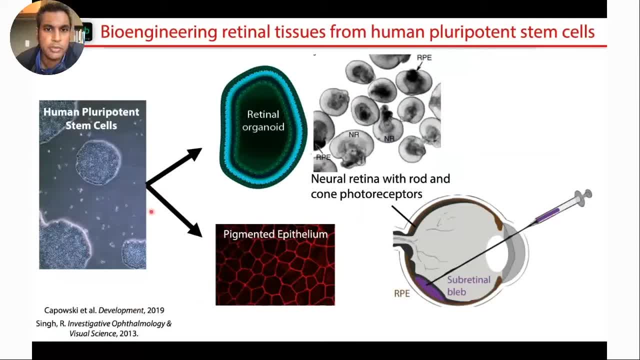 lab who's pioneered some of the differentiation methods of going from differentiation methods of going from differentiation methods of going from stem cells into various tissues of the stem cells, into various tissues of the stem cells, into various tissues of the eye, namely the pigmented epithelial layer. 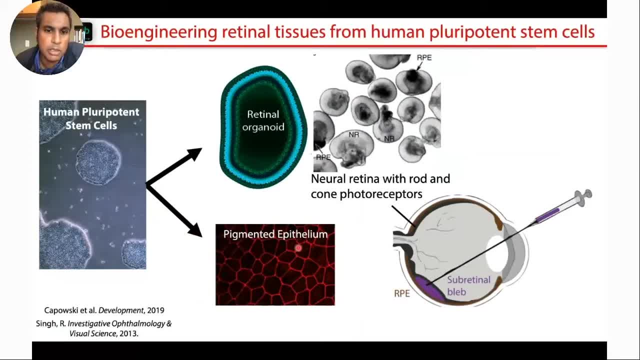 eye, namely the pigmented epithelial layer. eye, namely the pigmented epithelial layer. retinal pigmented epithelium- that I'll be. retinal pigmented epithelium. that I'll be. retinal pigmented epithelium. that I'll be mostly talking about today, but we also 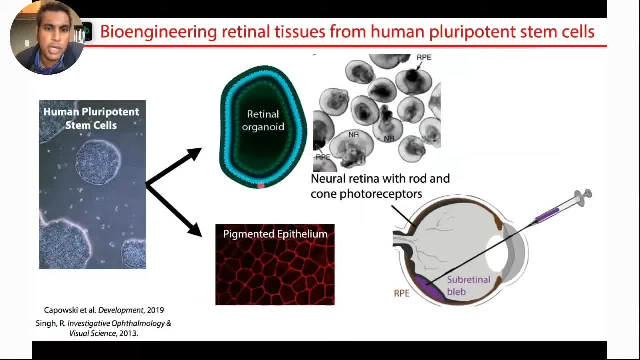 mostly talking about today. but we also mostly talking about today. but we also have projects that are in 3d retinal, have projects that are in 3d retinal, have projects that are in 3d retinal- organoids that have photoreceptors as. 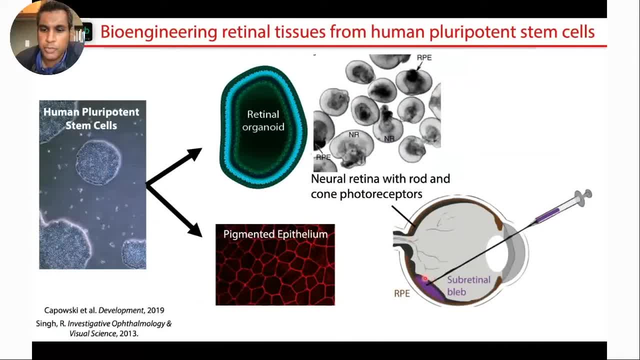 organoids that have photoreceptors as organoids that have photoreceptors as kind of the inner retina here. so that's kind of the inner retina here. so that's kind of the inner retina here. so that's shown in by my laser pointer in this. 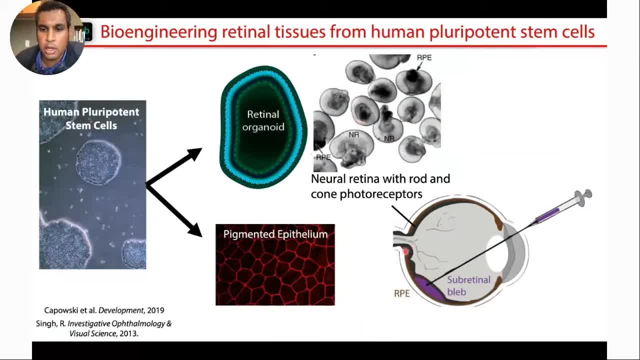 shown in by my laser pointer in this, shown in by my laser pointer in this black area. that would be for the retinal black area, that would be for the retinal black area, that would be for the retinal organoid, the RPE. the epithelial is in. 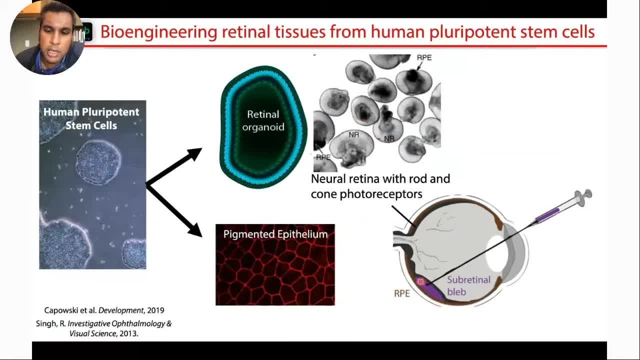 organoid, the RPE, the epithelial is in organoid, the RPE, the epithelial is in the back and, clinically, this layer, the, the back. and clinically, this layer, the, the back. and clinically, this layer, the epithelia as well as the photoreceptors. epithelia as well as the photoreceptors. 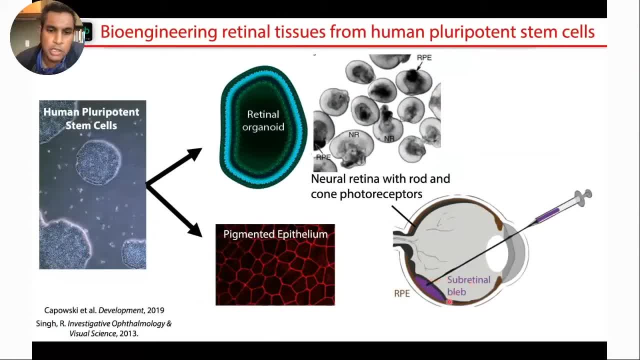 epithelia, as well as the photoreceptors, are accessible through a sub retinal, are accessible through a sub retinal, are accessible through a sub retinal injection, and so any test, this product injection, and so any test, this product injection, and so any test, this product is delivered that way and- and there's a 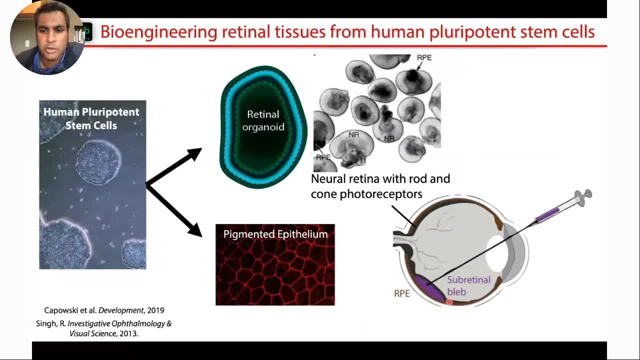 is delivered that way and and there's a is delivered that way and and there's a quite a bit of excitement in the field, quite a bit of excitement in the field, quite a bit of excitement in the field of delivering many other types of, of delivering many other types of. 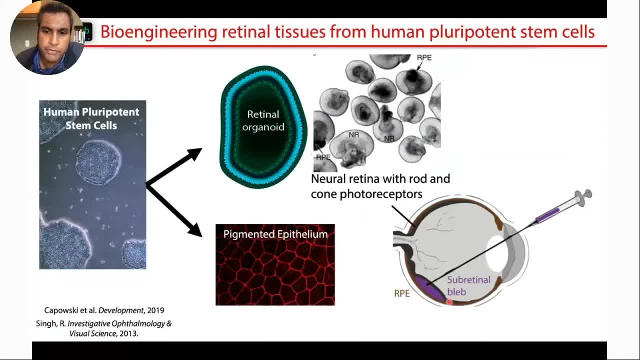 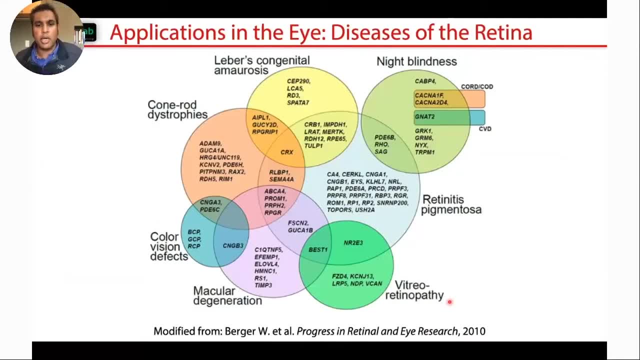 of delivering many other types of editors into the sub retinal space, this editors into the sub retinal space, this editors into the sub retinal space. this can be done fairly easily by trained, can be done fairly easily by trained can be done fairly easily by trained surgeons. so the eye from my point of 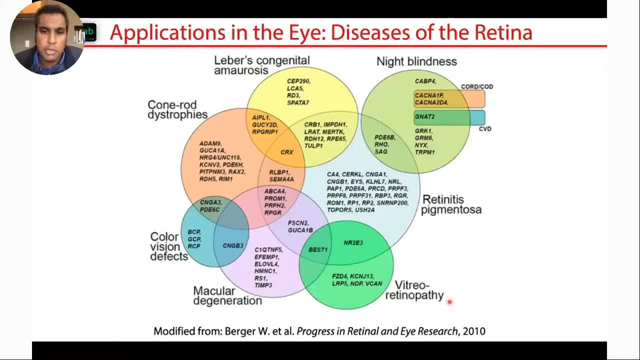 surgeons. so the eye from my point of surgeons, so the eye from my point of view, is a very exciting place to do. view is a very exciting place to do. view is a very exciting place to do. genome editing, uh, namely because uh, genome editing, uh, namely because uh. 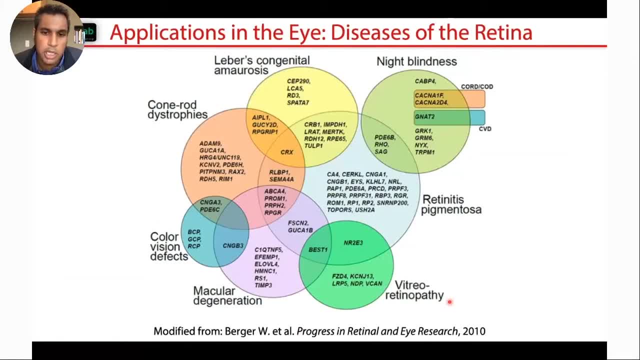 genome editing, uh, namely because, uh, there's a lot of need out there and the there's a lot of need out there and the there's a lot of need out there, and the genetics and of various genetics and of various genetics and of various disorders are quite diverse. so this: 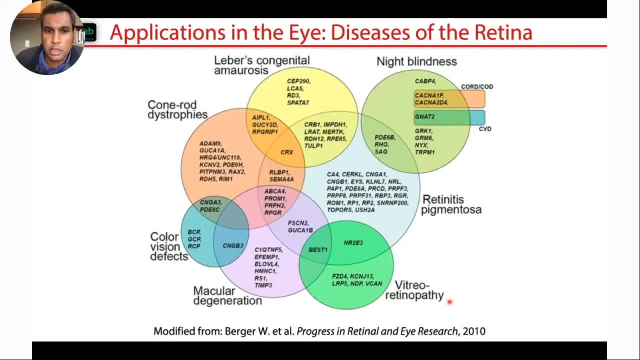 disorders are quite diverse. so this disorders are quite diverse. so this venn diagram, venn diagram, venn diagram: it shows that the genes that have been. it shows that the genes that have been. it shows that the genes that have been identified, identified, identified. that was about 10 years ago, for. 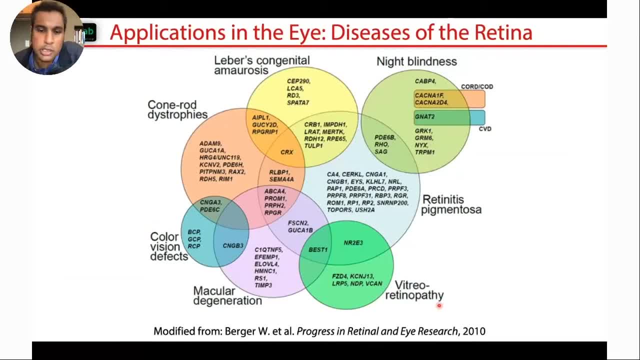 that was about 10 years ago. for that was about 10 years ago for for a number of different visual, for a number of different visual, for a number of different visual disorders, and this list has just disorders, and this list has just disorders, and this list has just increased um every year. i'll be focusing 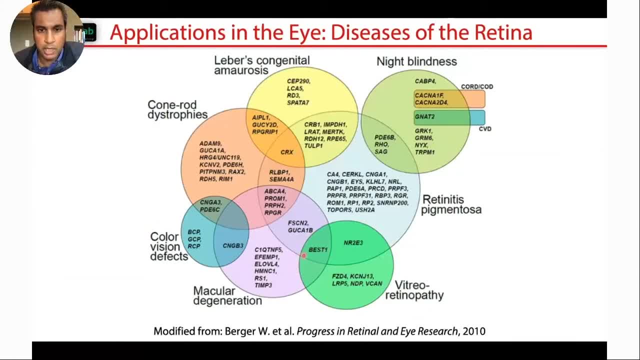 increased um every year. i'll be focusing- increased um every year. i'll be focusing on this one gene, on this one gene, on this one gene that leads to um macular degeneration, that leads to um macular degeneration that leads to um macular degeneration as and um problems in vision, called best. 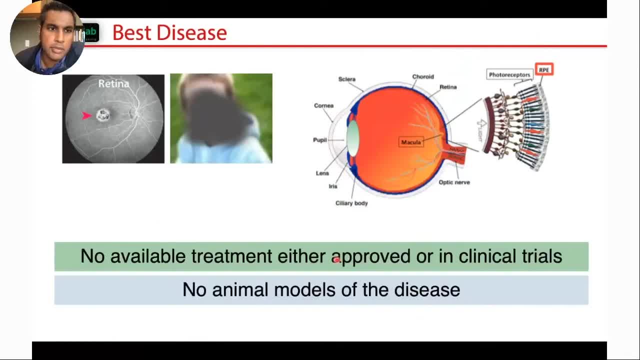 as and um problems in vision called best as and um problems in vision called best one one. one best disease is uh one where uh central best disease is uh one where uh central best disease is uh one where uh central vision, as you can see here, this is what. 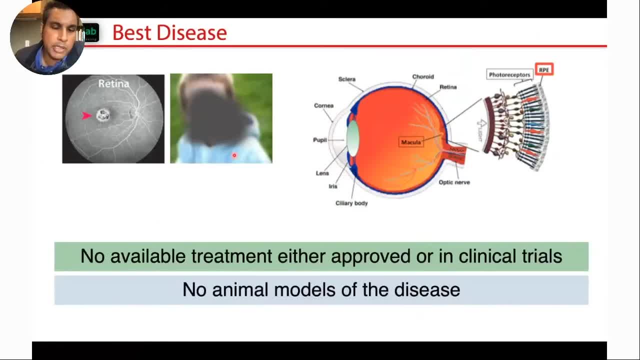 vision, as you can see here. this is what vision. as you can see here. this is what: um patients, uh, who have best disease, um patients, uh, who have best disease, um patients, uh, who have best disease, would see they would lose central vision. would see they would lose central vision. 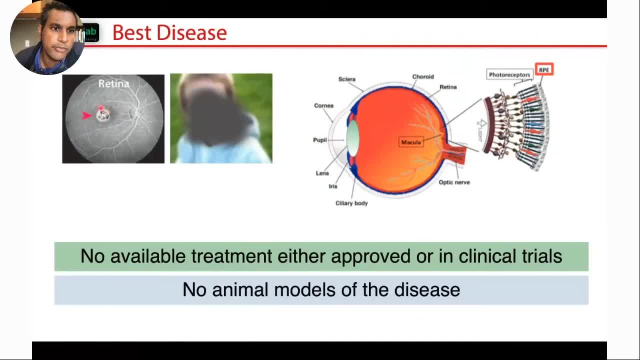 would see, they would lose central vision. you can see kind of build up uh abnormal. you can see kind of build up uh abnormal. you can see kind of build up uh abnormal build up of build up, of build up of material here in the back of the eye and 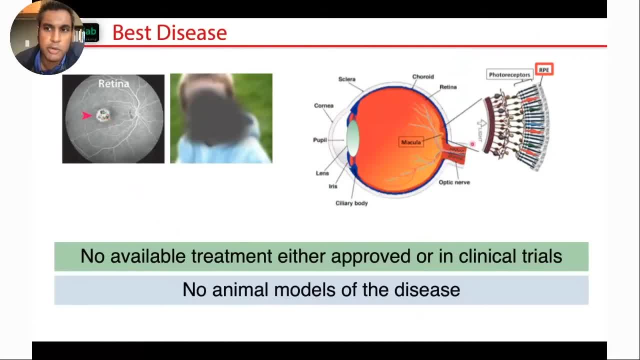 material here in the back of the eye and material here in the back of the eye, and again, that's again, that's again. that's largely because this best one gene is, largely because this best one gene is, largely because this best one gene is overexpressed in that epithelial layer. 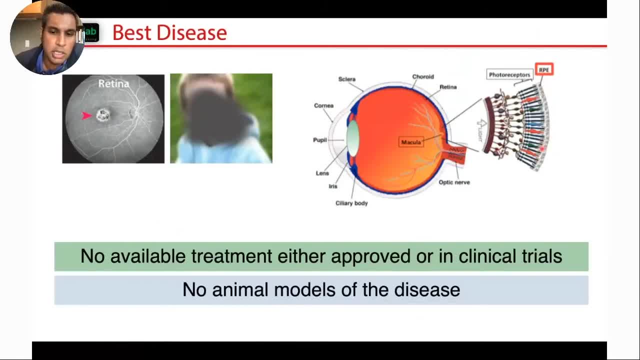 overexpressed in that epithelial layer, overexpressed in that epithelial layer. that i'll talk about that. i'll talk about that. i'll talk about the challenge here is, and is that there? the challenge here is, and is that there? the challenge here is, and is that there are no treatments for this disease. but 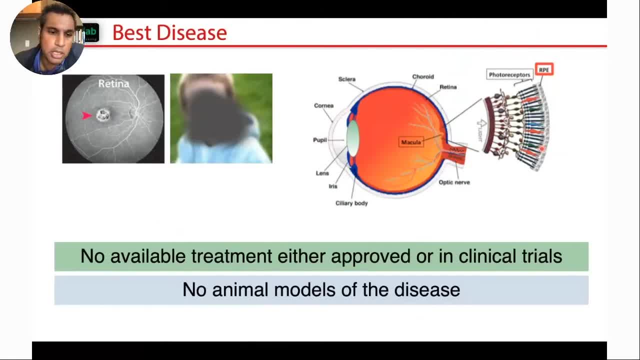 are no treatments for this disease, but are no treatments for this disease, but also also also for kind of pre-clinical and early stage. for kind of pre-clinical and early stage, for kind of pre-clinical and early stage work. there's no very good animal models. 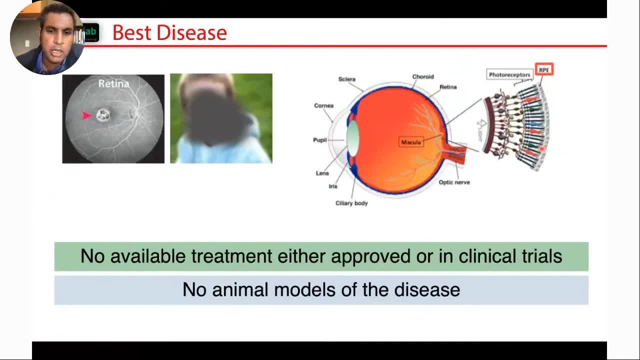 work. there's no very good animal models work. there's no very good animal models of the disease that really recapitulate of the disease, that really recapitulate of the disease, that really recapitulate what the patients are, what the patients are, what the patients are progressing through and what clinicians 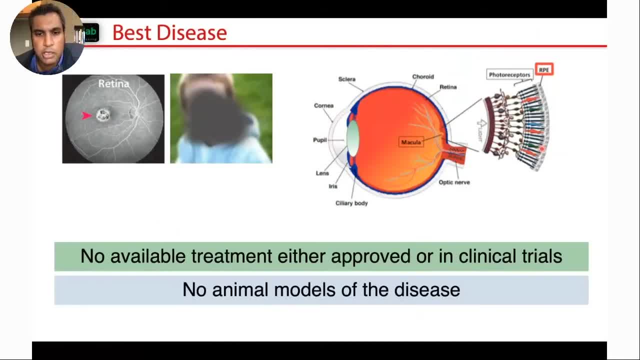 progressing through and what clinicians progressing through and what clinicians are seeing are seeing, are seeing, and so this and so this, and so this motivates the use of using human motivates, the use of using human motivates, the use of using human stem cells, stem cells, stem cells as a model system, and so best one is a. 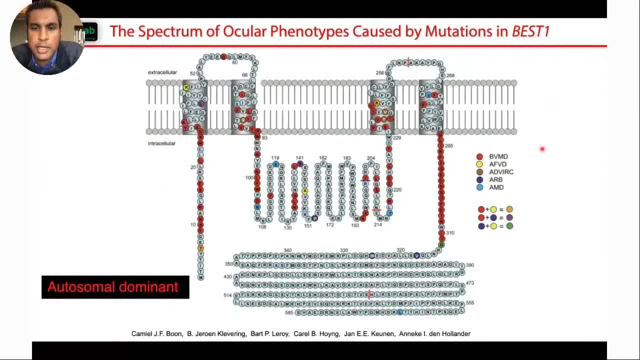 as a model system, and so best one is a as a model system, and so best one is a. transmembrane, transmembrane, transmembrane protein. it encodes for this um protein. it encodes for this um protein. it encodes for this um, you know, fairly large protein that has 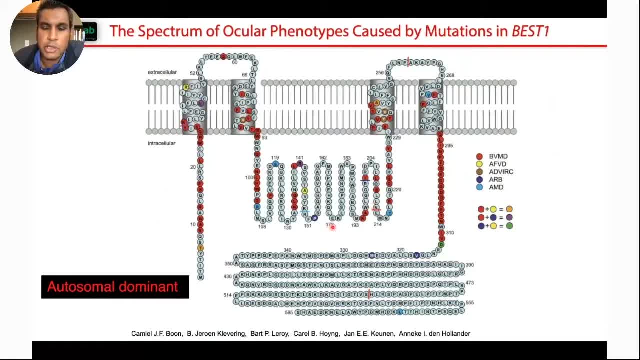 you know, fairly large protein that has, you know, fairly large protein that has several domains, and i'll be several domains and i'll be several domains and i'll be focusing in on some of the red, focusing in on some of the red, focusing in on some of the red mutations that are shown here in this. 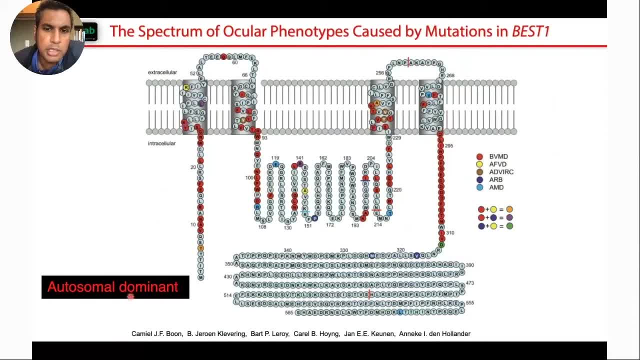 mutations that are shown here in this, mutations that are shown here in this, in this schematic, that have been in this schematic, that have been in this schematic, that have been autosomal dominant mutations, so one autosomal dominant mutations, so one autosomal dominant mutations. so one copy will lead to disease. 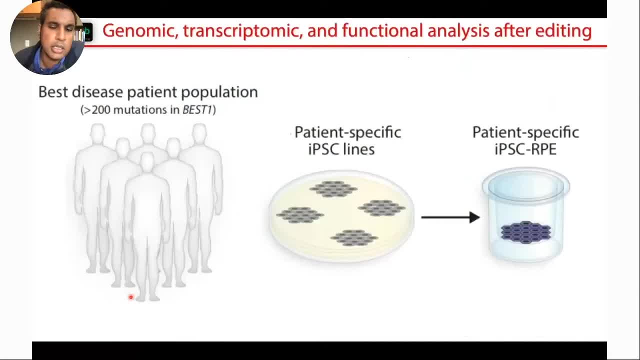 copy will lead to disease. copy will lead to disease and, in this scenario, what we've done is- and in this scenario, what we've done is, and in this scenario, what we've done is: taken, taken, taken. a number of patients generated ips lines. a number of patients generated ips lines. 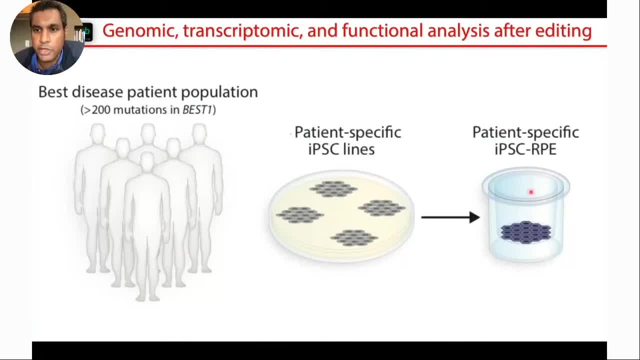 a number of patients generated ips lines through reprogramming from their blood, through reprogramming from their blood, through reprogramming from their blood or skin, or skin or skin, and then differentiated them into rpe and then differentiated them into rpe, and then differentiated them into rpe. what we focused on is 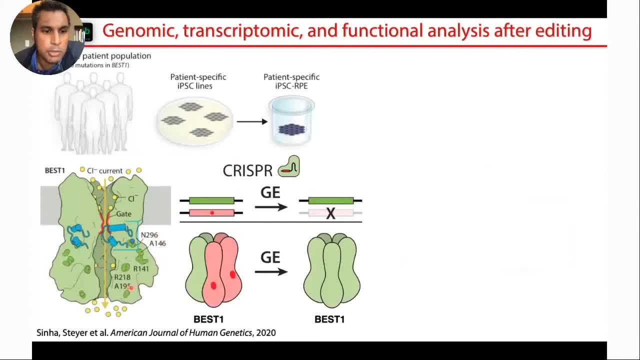 what we focused on is. what we focused on is patients that have patients that have patients that have these particular mutations in these particular mutations, in these particular mutations in important areas of this, important areas of this, important areas of this channel. so best one encodes a channel, so best one encodes a. 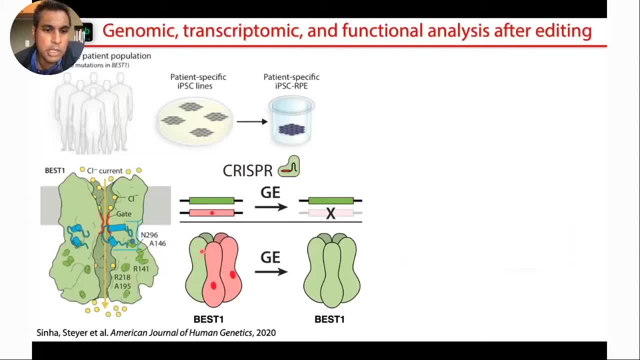 channel. so best one encodes a multimer, multimer, multimer. so there's a homopentameric channel, so there's a homopentameric channel. so there's a homopentameric channel, meaning that there's, meaning that there's. 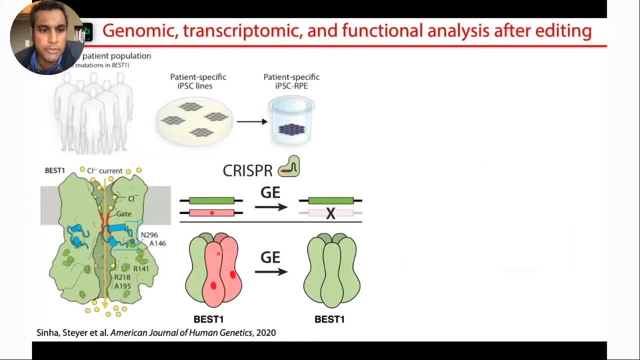 meaning that there's five proteins that come together, really, five proteins that come together, really, five proteins that come together really in this type of orientation, in this type of orientation, in this type of orientation according to the crystal structure that, according to the crystal structure that, according to the crystal structure that was recently. 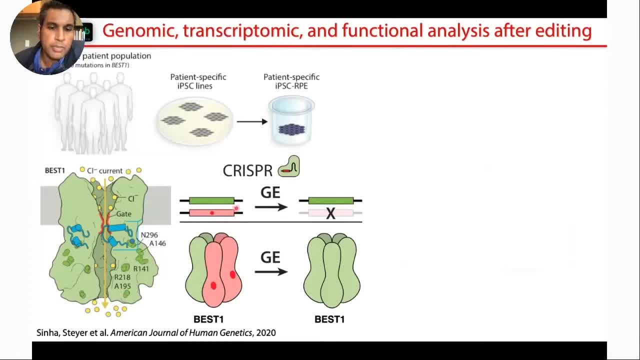 solved and dominant, solved and dominant, solved and dominant. patients with the dominant form of the patients, with the dominant form of the patients, with the dominant form of the disease, have disease, have disease, have one problematic mutant copy, one problematic mutant copy, one problematic mutant copy. and the goal of our crispr technique is: 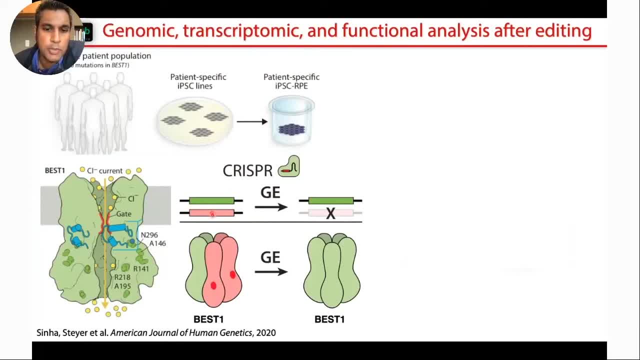 and the goal of our crispr technique is: and the goal of our crispr technique is to specifically cut and disrupt the. to specifically cut and disrupt the. to specifically cut and disrupt the mutant copy. mutant copy. mutant copy such that the the remaining untouched in, such that the the remaining untouched in. 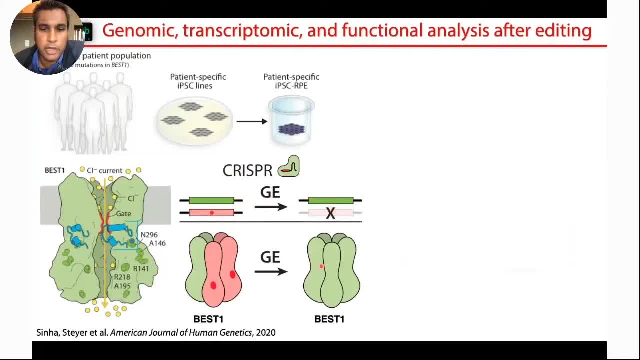 such that the the remaining untouched, in theory, wild type copy would take over theory. wild type copy would take over theory. wild type copy would take over and essentially flood this homopentameric and essentially flood this homopentameric and essentially flood this homopentameric channel. 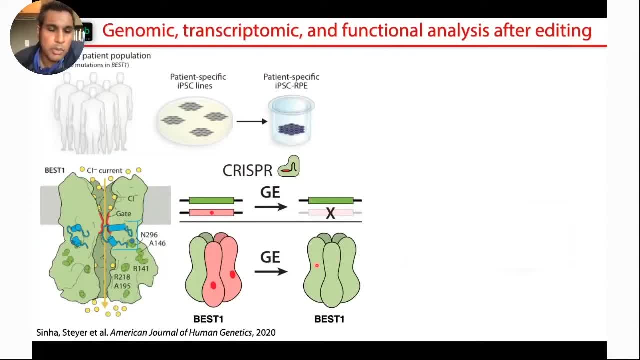 channel, channel into all wild type forms, into all wild type forms, into all wild type forms, and what we learned really, and what we learned really, and what we learned really, is that it does matter, which is that it does matter, which is that it does matter, which particular edit. 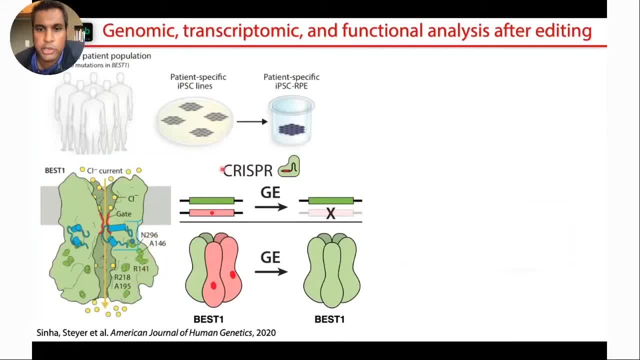 particular edit, particular edit: the patient has, and so i'll go through the patient has, and so i'll go through the patient has, and so i'll go through that data in the next few slides, that data in the next few slides, that data in the next few slides, um what we chose to use as our candidate. 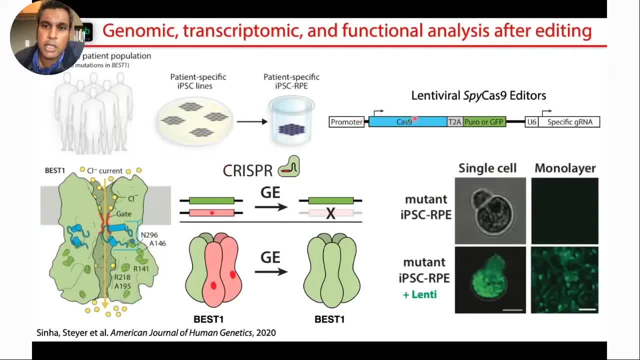 um, what we chose to use as our candidate. um, what we chose to use as our candidate- gene therapy- here is to gene therapy, here is to gene therapy, here is to drive spy cas9, drive spy cas9, drive spy cas9 and have a 2a with a gfp in in many of 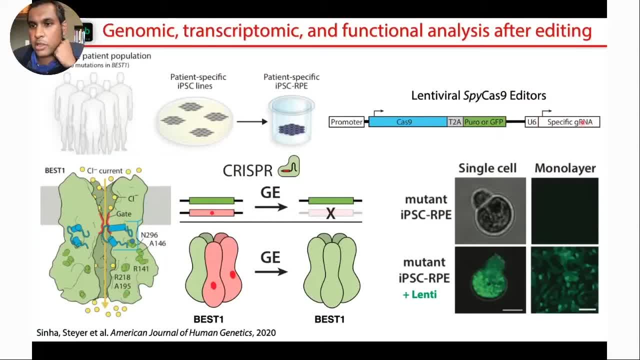 and have a 2a with a gfp in in many of, and have a 2a with a gfp in in many of these studies, these studies, these studies and a separate promoter that drives the and a separate promoter that drives the and a separate promoter that drives the mutant allele. specific guide rna. to cut. 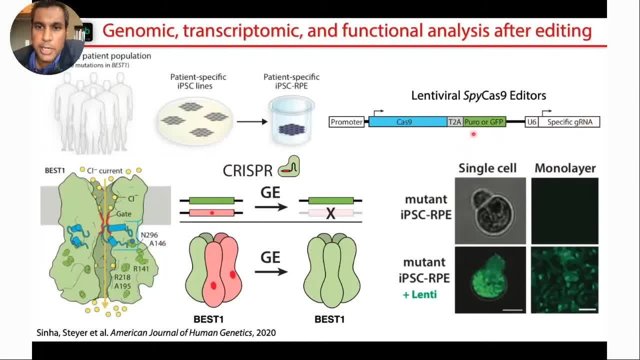 mutant allele: specific guide rna to cut mutant allele- specific guide rna- to cut this mutant allele, this mutant allele, this mutant allele, and we get very good transduction and we get very good transduction and we get very good transduction of these human rpe layers. 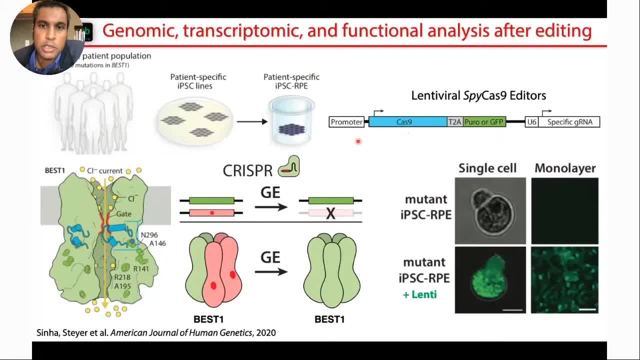 of these human rpe layers, of these human rpe layers, and the promoter here is driven by the and the promoter here is driven by the and the promoter here is driven by the endogenous best one promoter, so we have endogenous best one promoter, so we have. 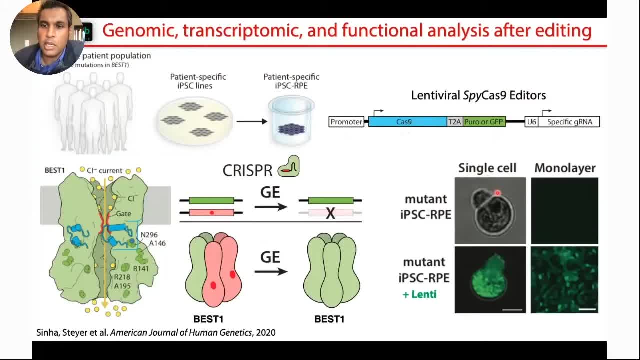 endogenous, best one promoter. so we have cell type, specific expression of our cell type, specific expression of our cell type, specific expression of our editor, editor, editor and some of the studies that we can do and some of the studies that we can do and some of the studies that we can do in rpe is both single cell we can patch. 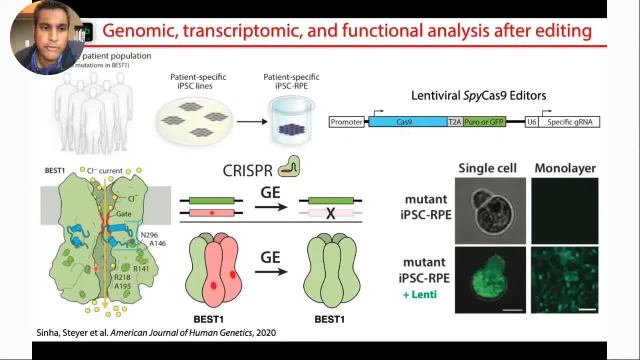 in rpe is both single cell we can patch. in rpe is both single cell, we can patch. clamp- a single cell. look for clamp- a single cell. look for clamp- a single cell. look for current flow through there and that current flow through there and that current flow through there and that would be a chloride current flow. 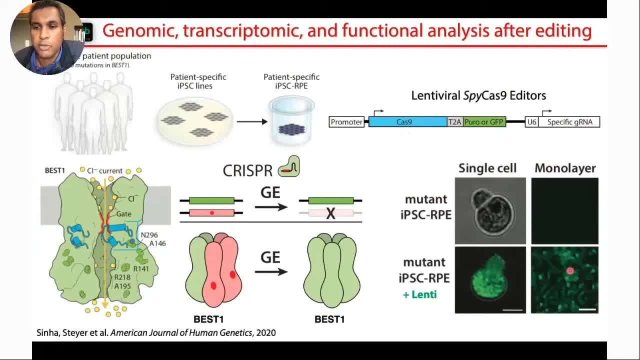 would be a chloride current flow would be a chloride current flow. or we could take a whole kind of, or we could take a whole kind of, or we could take a whole kind of monolayer and look for whether it monolayer and look for whether it. 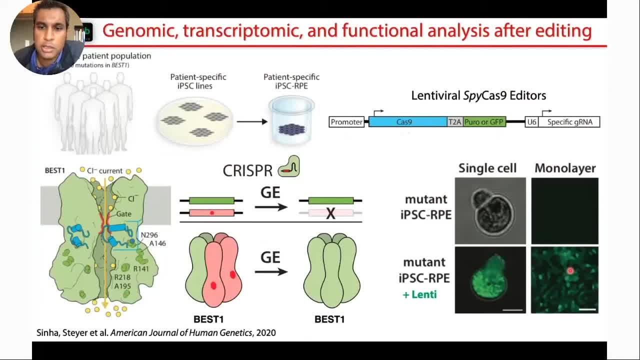 monolayer and look for whether it degrades some of the photoreceptor outer, degrades some of the photoreceptor outer, degrades some of the photoreceptor outer segments that segments, that segments that they naturally do inside the eye, they naturally do inside the eye. 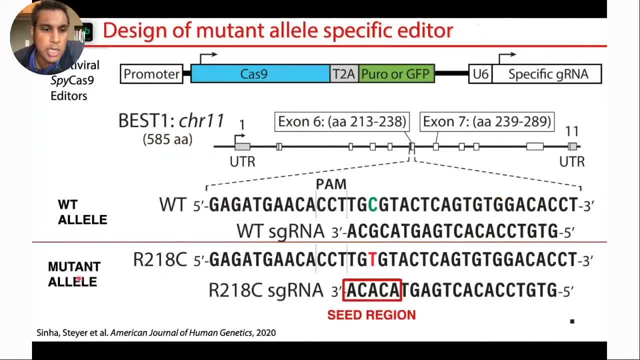 they naturally do inside the eye. and so this is one example for, and so this is one example for, and so this is one example for one specific patient that has this, one specific patient that has this, one specific patient that has this mutant allele r218c. mutant allele r218c. 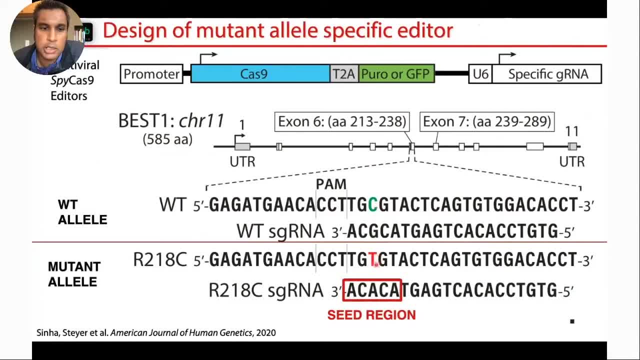 mutant allele r218c. that single base change is that single base change is that single base change is c to t here, and so what we do is we c to t here, and so what we do is we c to t here, and so what we do is we design our guide. 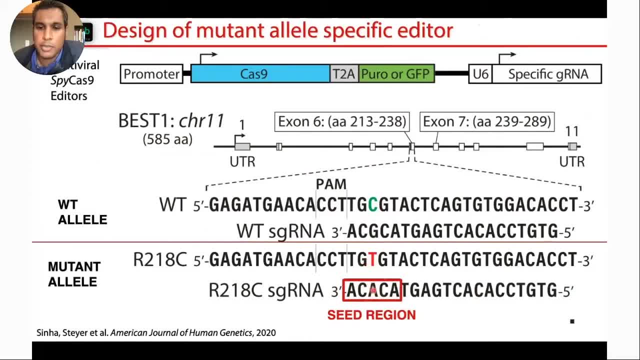 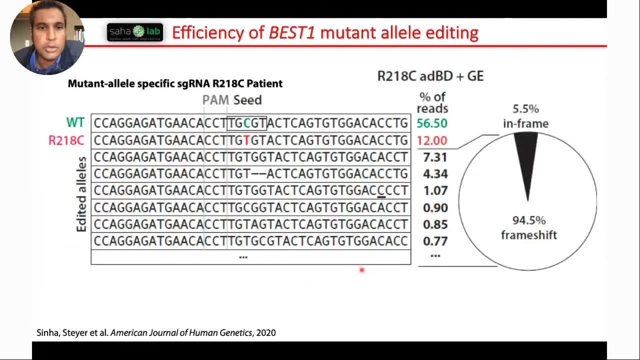 design our guide, design our guide to be specific to the mutant allele, to be specific to the mutant allele, to be specific to the mutant allele such that it will specifically cut this, such that it will specifically cut this, such that it will specifically cut this allele. and so, when we do this, um, we and and we. 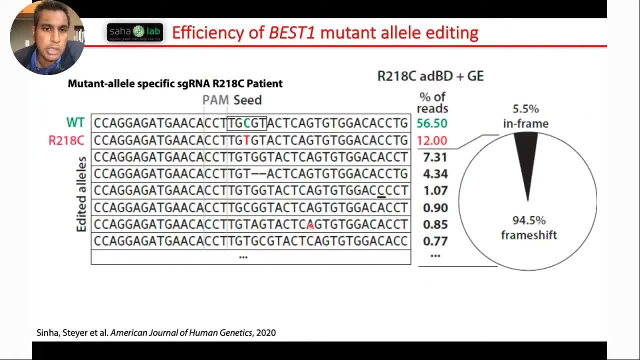 and so when we do this, um, we and, and we, and so when we do this, um, we and, and we take out the cells extract genomic dna, take out the cells extract genomic dna, take out the cells extract genomic dna and sequence it through, and sequence it through. 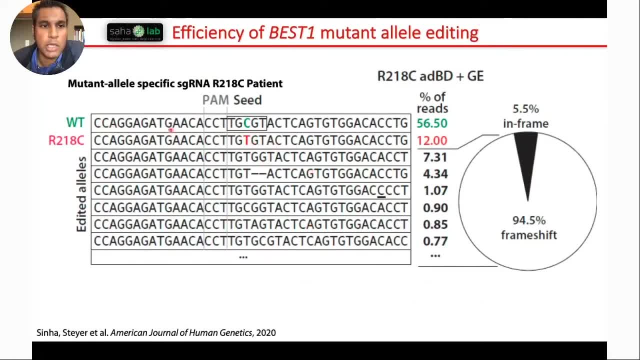 and sequence it through lumina, deep sequencers, lumina, deep sequencers, lumina, deep sequencers. we get our wild type alleles showing up. we get our wild type alleles showing up. we get our wild type alleles showing up as our most common read, as our most common read. 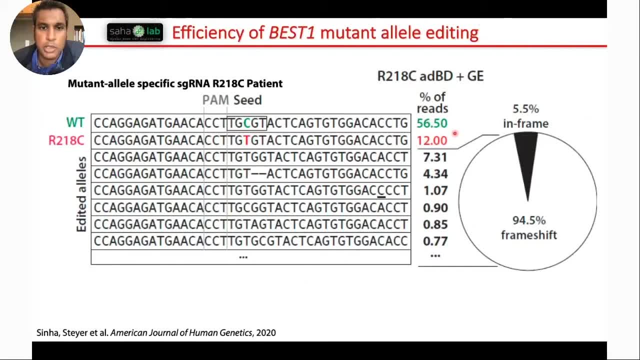 as our most common read and that's approximately 50 of our, and that's approximately 50 of our, and that's approximately 50 of our reads which is reads which is reads which is good, uh and good, uh and good, uh. and the next most common is the untouched. 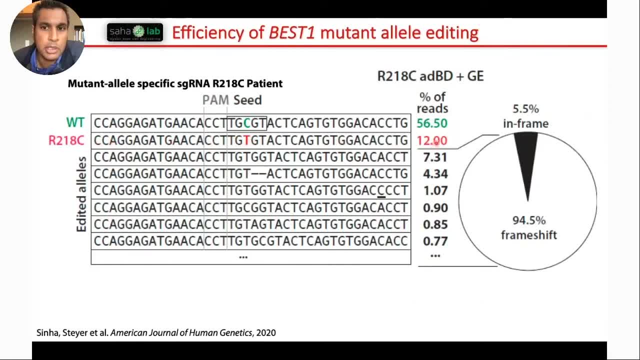 the next most common is the untouched. the next most common is the untouched mutant allele, which is 12, mutant allele, which is 12. mutant allele, which is 12. so we haven't completely eliminated it, so we haven't completely eliminated it, so we haven't completely eliminated it. but then you can start to see. 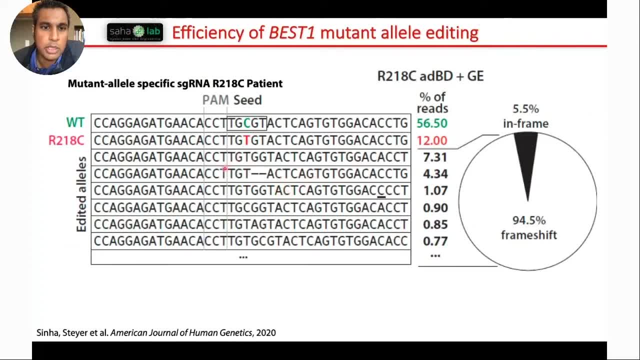 but then you can start to see. but then you can start to see, um, some of the uh, um, some of the uh, um, some of the uh, the the mutant alleles that come out. so the the mutant alleles that come out. so the the mutant alleles that come out. so here's a two base pair deletion. 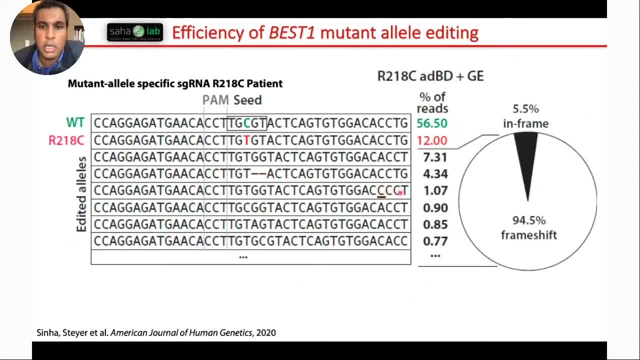 here's a two base pair deletion. here's a two base pair deletion: um, there's a uh insertion here. um, there's a uh insertion here. um, there's a uh insertion here, and so there's there's a number of, and so there's there's a number of. 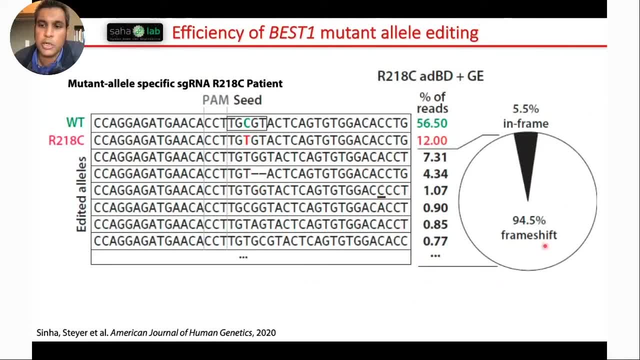 and so there's, there's, there's a number of indels here that indels here, that indels here that, on the whole, end up uh generating 94, on the whole end up uh generating 94, on the whole end up uh generating 94 frameshift. 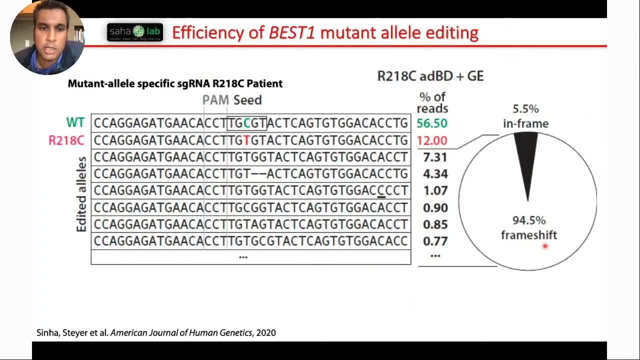 frameshift. frameshift and frame shifts are important because and frame shifts are important because and frame shifts are important because those trigger nonsense, mediated decay, those trigger nonsense, mediated decay, those trigger nonsense, mediated decay, and the specificity is high, and so we. and the specificity is high, and so we. 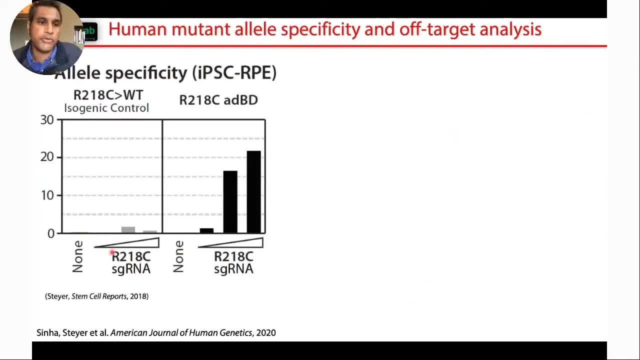 and the specificity is high, and so we can um, can um, can um. we have an isogenic control that we've. we have an isogenic control that we've. we have an isogenic control that we've generated using methods generated using methods. generated using methods similar to what we just heard in the. 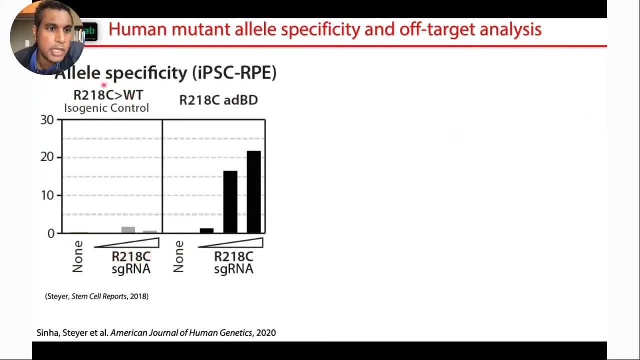 similar to what we just heard in the, similar to what we just heard in the first talk. first talk, first talk where we've, where we've, where we've, corrected that r218c back to the wild, corrected that r218c back to the wild, corrected that r218c back to the wild type in the ips cell state. 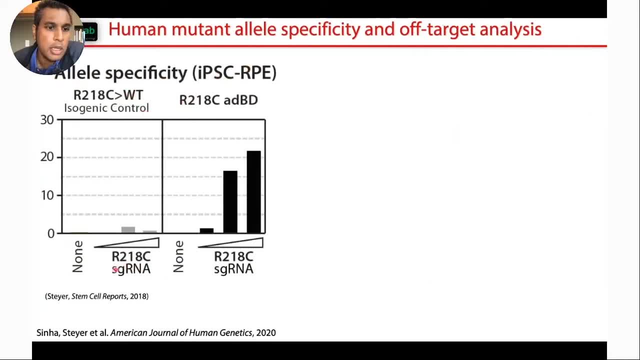 type in the ips cell state, type in the ips cell state and then differentiated them to rpe and then differentiated them to rpe and then differentiated them to rpe. when we apply the mutant specific allele, when we apply the mutant specific allele, when we apply the mutant specific allele editor, we see: 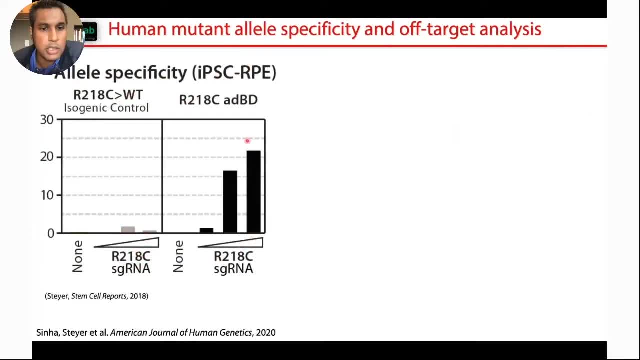 editor. we see editor. we see some cutting, but not as much and not some cutting, but not as much, and not some cutting, but not as much, and not as much as you would see in the actual, as much as you would see in the actual, as much as you would see in the actual mutant specific. 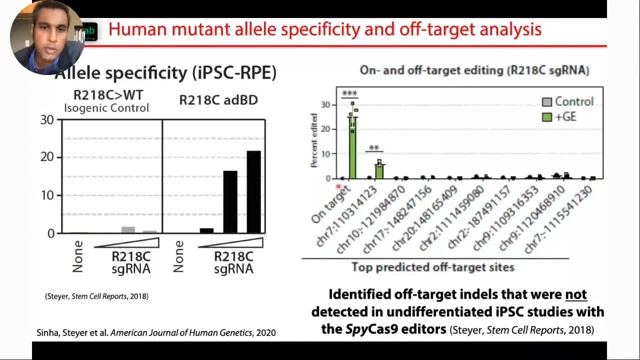 mutant specific, mutant specific informatic techniques, the top off informatic techniques, the top off informatic techniques. the top off target site is actually the wild type target site, is actually the wild type target site, is actually the wild type allele. so it's actually, it's a bit. 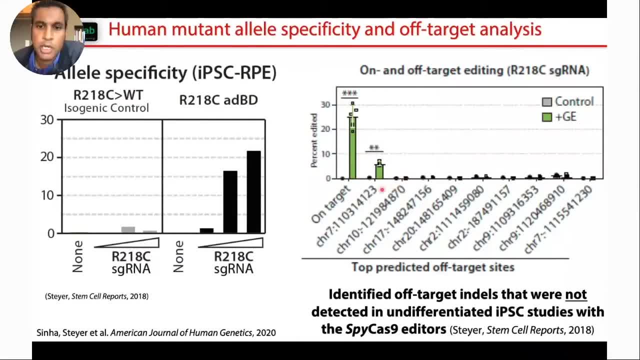 allele, so it's actually it's a bit allele, so it's actually it's a bit confusing there, and we get confusing there, and we get confusing there and we get some cutting, but we also identify some cutting, but we also identify some cutting, but we also identify some cutting at one. 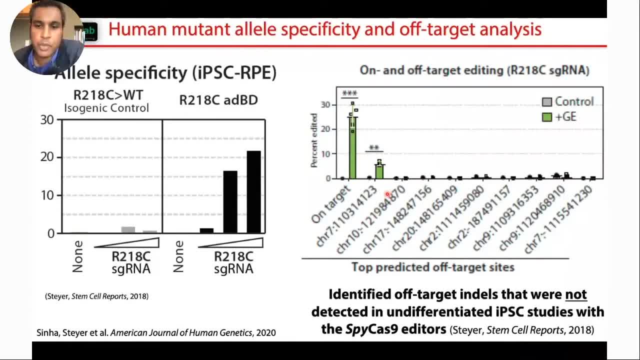 some cutting at one, some cutting at one place in chromosome seven, that place in chromosome seven, that place in chromosome seven that we actually only saw when we used. we actually only saw when we used. we actually only saw when we used rpe differentiated cells. we did not see. 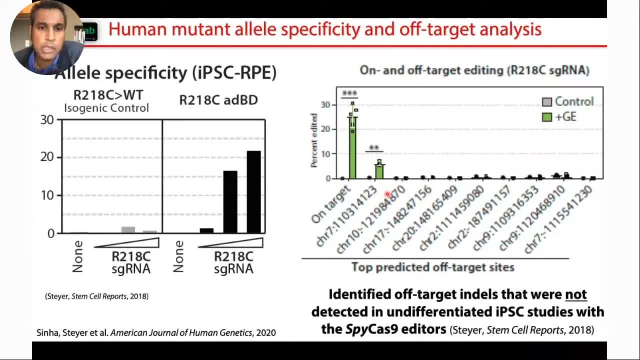 rpe differentiated cells. we did not see rpe differentiated cells. we did not see that when we applied the um, a similar that when we applied the um, a similar that when we applied the um, a similar editing technique on ips cells. so editing technique on ips cells. so 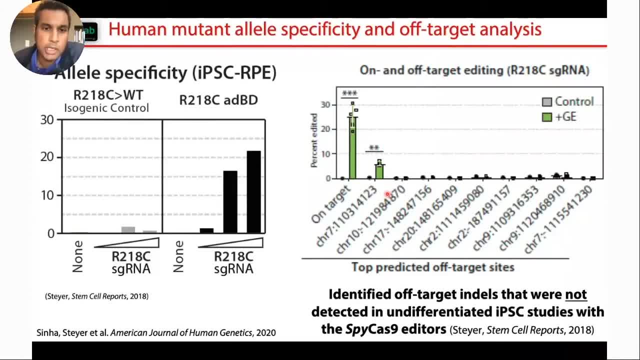 editing technique on ips cells. so there's some value. i think of there's some value. i think of there's some value, i think of using the differentiated cell type, to using the differentiated cell type, to using the differentiated cell type to identify off-target, identify off-target. 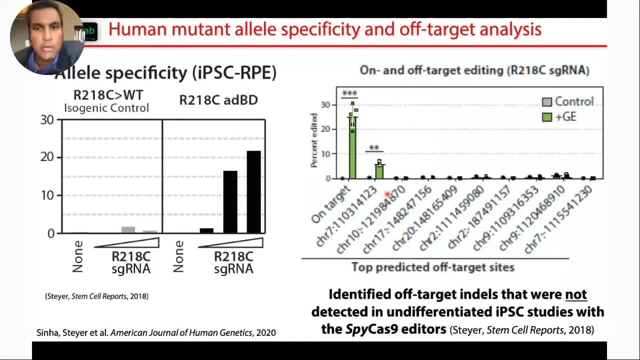 identify off-target, potential off-target modifications, potential off-target modifications, potential off-target modifications. and overall, when we looked at all of our and overall, when we looked at all of our and overall, when we looked at all of our strategies for the different patients, strategies for the different patients. 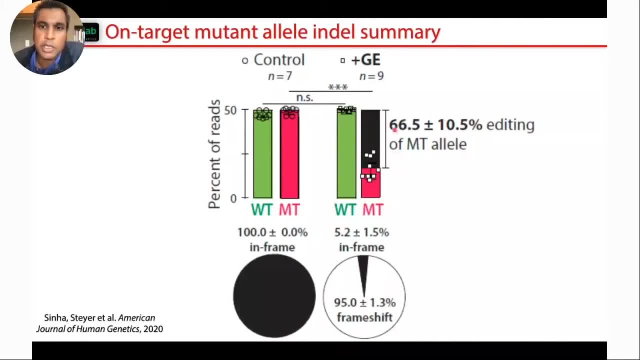 strategies for the different patients: uh the mutant allele specific strategy. uh the mutant allele specific strategy. uh the mutant allele specific strategy ended up disrupting the mutant allele. in ended up disrupting the mutant allele. in ended up disrupting the mutant allele in about 70, about 70, about 70 at about 70, 66, you know plus or minus 10. 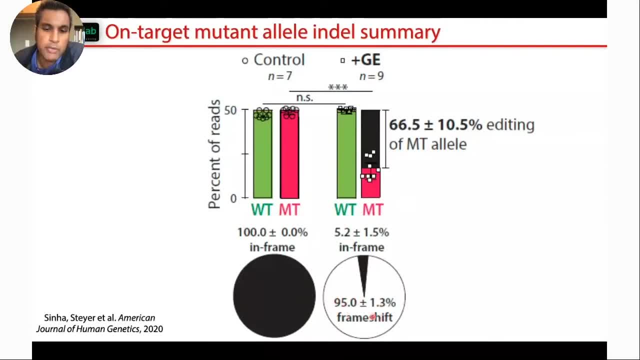 at about 70- 66, you know plus or minus 10 at about 70: 66, you know plus or minus 10 here here, here, um, and they all gave remarkably high um and they all gave remarkably high um and they all gave remarkably high levels of. 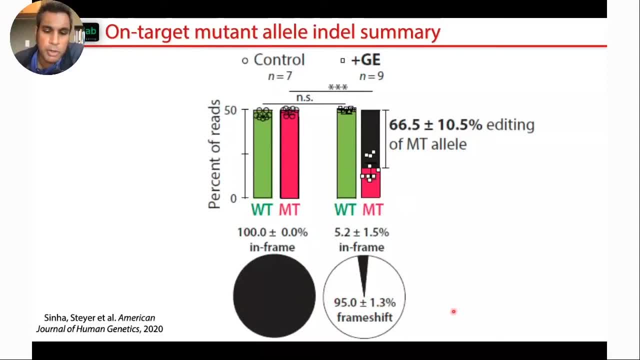 levels of levels of frame shifts and i think that might have frame shifts and i think that might have frame shifts and i think that might have to do with dna repair processes in the to do with dna repair processes in the to do with dna repair processes in the rpe specifically, that are largely a 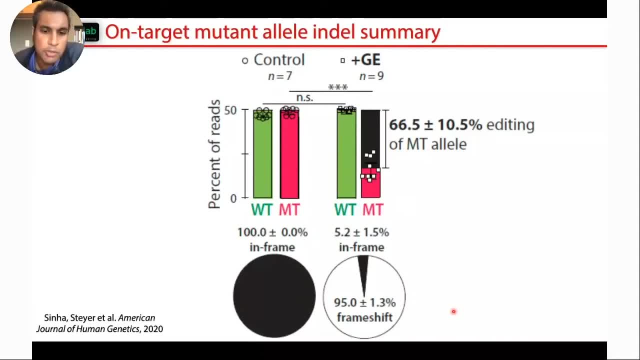 rpe, specifically, that are largely a rpe, specifically, that are largely a non-dividing cell, that non-dividing cell that ends up having a plus one, ends up having a plus one, ends up having a plus one. mutation spectrum in terms of insert. mutation spectrum in terms of insert. 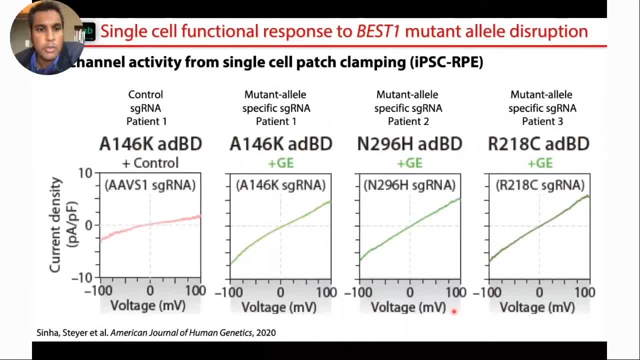 mutation spectrum in terms of insert, insertion of bases, insertion of bases, insertion of bases. when we do functional tests on single. when we do functional tests on single, when we do functional tests on single cells, we see a rescue. whenever we do the cells, we see a rescue whenever we do the. 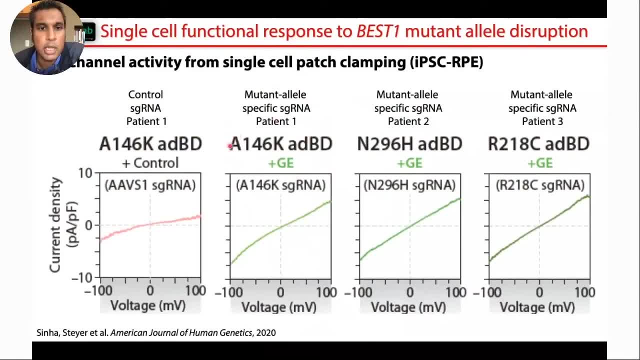 cells. we see a rescue whenever we do the mutant allele specific editor. mutant allele specific editor. mutant allele specific editor. so this is uh one of the patients a146k. so this is uh one of the patients a146k. so this is uh one of the patients a146k, uh 218c. 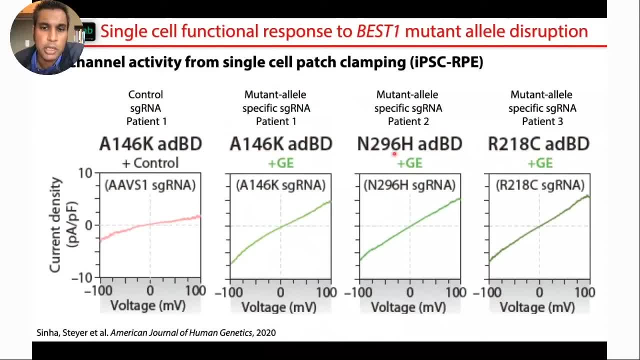 uh 218c, uh 218c on the far right is what i uh focused on. on the far right is what i uh focused on. on the far right is what i uh focused on um, and they all seem to increase the um and they all seem to increase the. 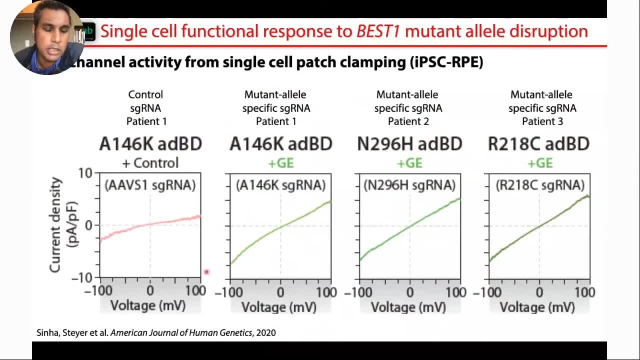 um, and they all seem to increase the current here, which is uh represented by current here, which is uh represented by current here, which is uh represented by a diagonal line in this current density, a diagonal line in this current density, a diagonal line in this current density, voltage plot. 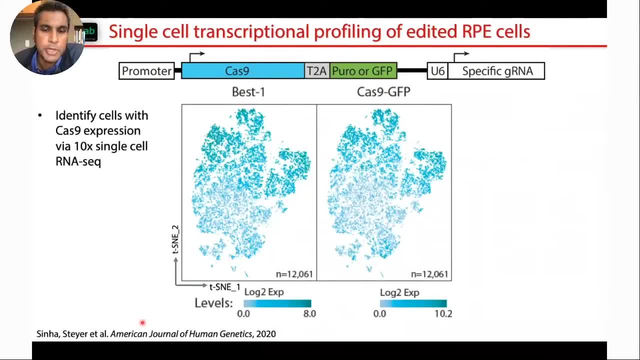 and one level further we looked for, and one level further we looked for, and one level further we looked for transcriptional perturbations in these transcriptional perturbations, in these transcriptional perturbations in these specific cell types. so what we could do, specific cell types, so what we could do. 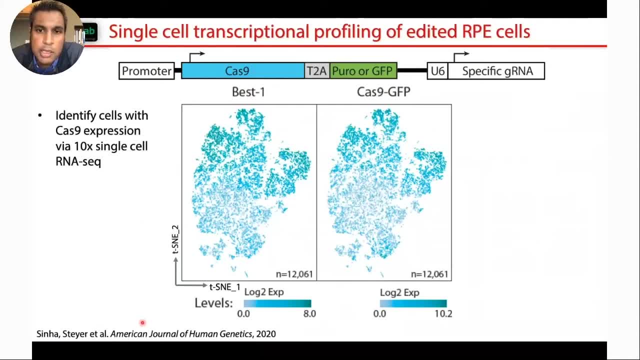 specific cell types. so what we could do using 10x single cell rna seek is to using 10x single cell rna seek is to using 10x single cell rna seek is to track cells that actually have, track cells that actually have. 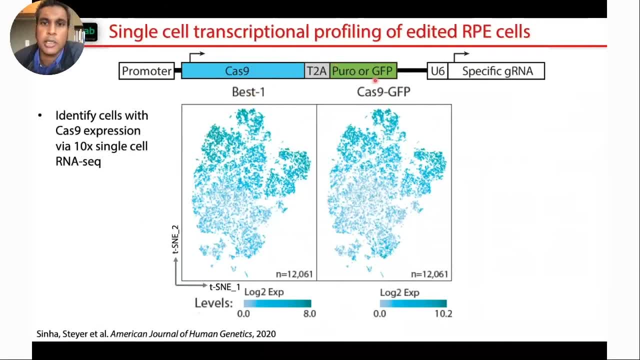 track cells that actually have transcripts arising from our transcripts, arising from our transcripts arising from our lentiviral construct, lentiviral construct, lentiviral construct, and as expected that the and as expected that the and as expected that the expression level of our, expression level of our, 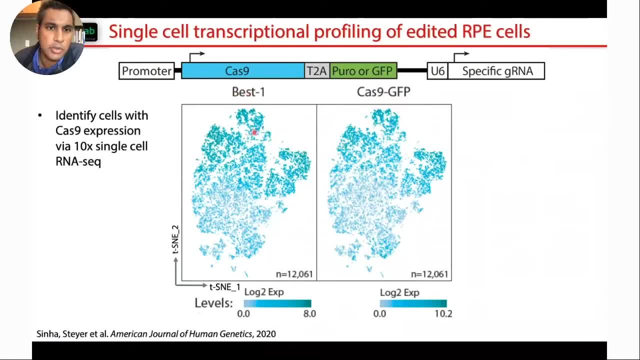 expression level of our cas9 gfp is. this is similar to what cas9 gfp is. this is similar to what cas9 gfp is. this is similar to what is um endogenously being driven. uh is um endogenously being driven. uh is um endogenously being driven. uh. best one using the best one. promoter. 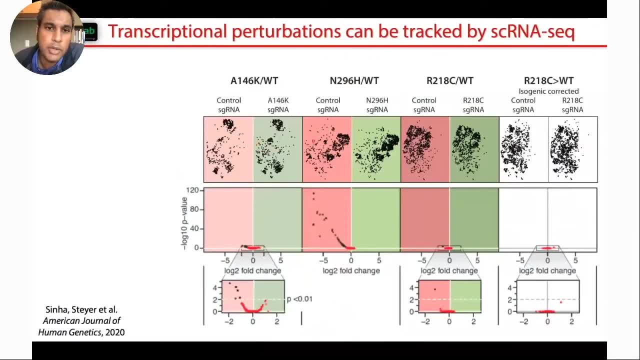 best one using the best one promoter. best one using the best one promoter. what we looked at in more detail was to. what we looked at in more detail was to. what we looked at in more detail was to see whether there was any abnormal. see whether there was any abnormal. 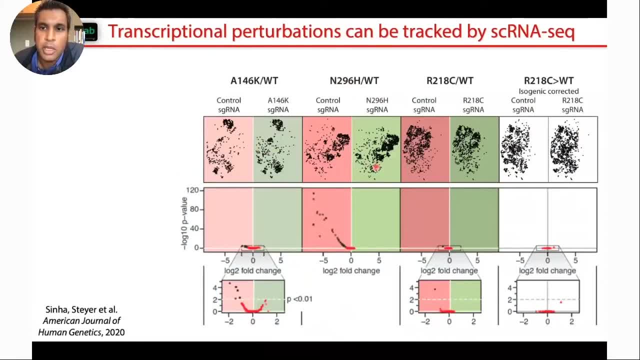 see whether there was any abnormal gene expression whenever we delivered gene expression, whenever we delivered gene expression, whenever we delivered our editor, our editor, our editor and what this plot is is a lot of, and what this plot is is a lot of, and what this plot is is a lot of different samples, but 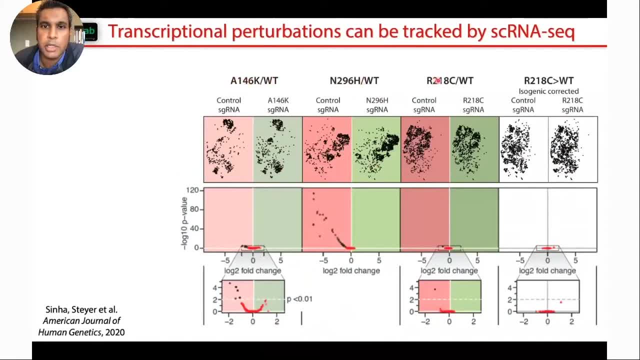 different samples, but different samples. but there are three different patient lines, there are three different patient lines, there are three different patient lines from the domino allele, from the domino allele, from the domino allele. mutation shown here: one, two, three and mutation shown here: one, two, three and. 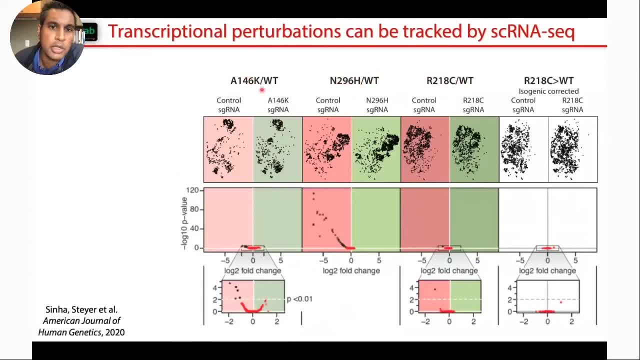 mutation shown here: one, two, three, and in each of those lines we've delivered. in each of those lines we've delivered. in each of those lines we've delivered an editor that was targeted against a, an editor that was targeted against a, an editor that was targeted against a mutant allele. 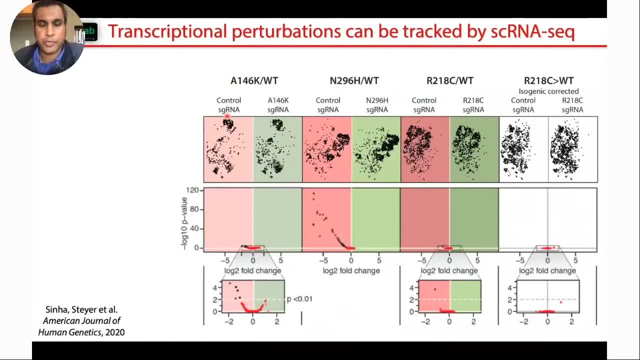 mutant allele. mutant allele or a control region that's that's not, or a control region that's that's not, or a control region that's that's not. coding in the cell, and so coding in the cell, and so coding in the cell. and so, uh, these are umap projections. 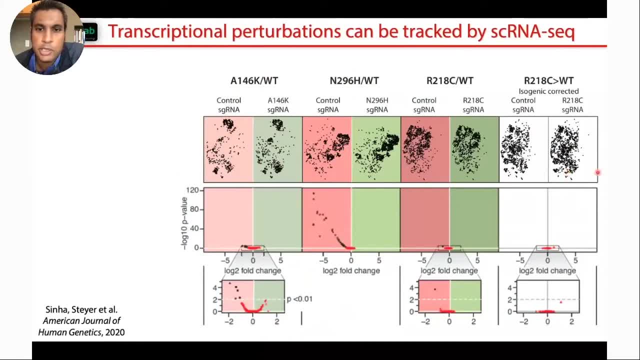 uh, these are umap projections. uh, these are umap projections of the 10x data and largely they're very of the 10x data and largely they're very of the 10x data and largely they're very similar, similar, similar and when we look at differentially, 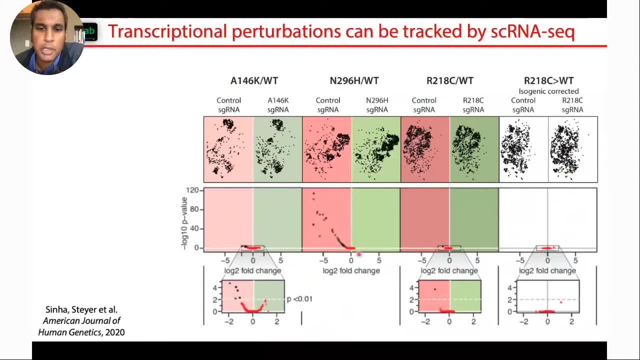 and when we look at differentially and when we look at differentially, expressed genes, expressed genes, expressed genes: there's very few that pop up on the. there's very few that pop up on the. there's very few that pop up on the whole, except for this one sample where 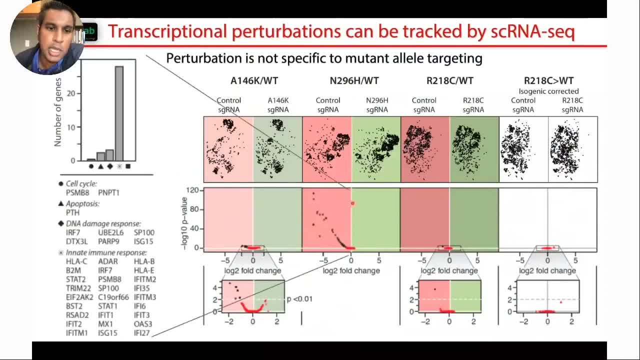 whole, except for this one sample, where, whole, except for this one sample, where we see quite a bit of, we see quite a bit of. we see quite a bit of genes that came up, genes that came up, genes that came up significantly different in this case, in significantly different, in this case, in 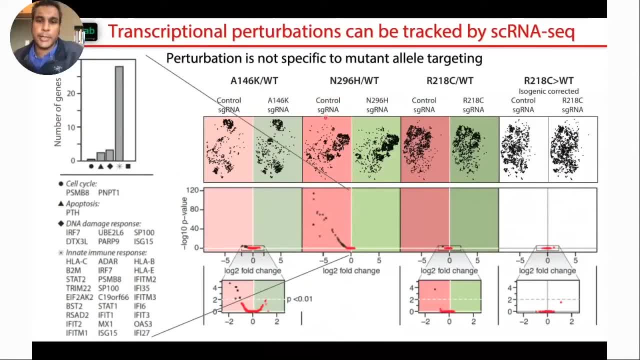 significantly different in this case, in the control, the control, the control targeted targeted targeted with the control targeted editor, with the control targeted editor, with the control targeted editor, and a lot of that had to do with stress and a lot of that had to do with stress and a lot of that had to do with stress response and innate immune response. so 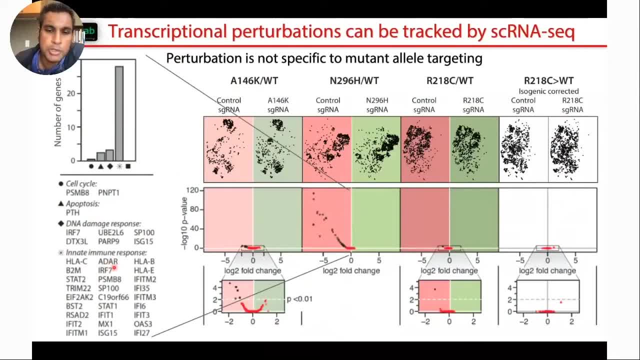 response and innate immune response. so response and innate immune response. so this, this could be a story uh related this. this could be a story uh related this. this could be a story uh related to transcriptional changes, from just to transcriptional changes, from just to transcriptional changes, from just simple transduction and dna damage. 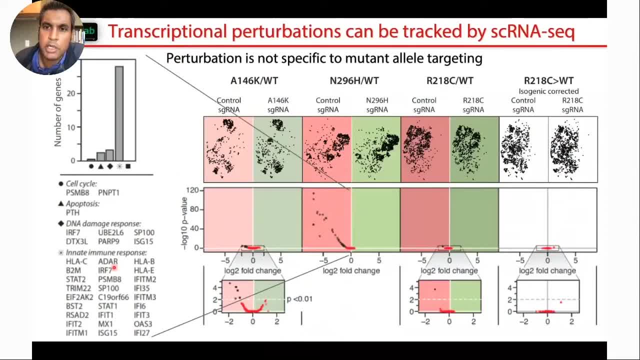 simple transduction and dna damage. simple transduction and dna damage, um, but we're we're looking more into um, but we're we're looking more into um, but we're we're looking more into this, but on the old the, the actual going this, but on the old the, the actual going. 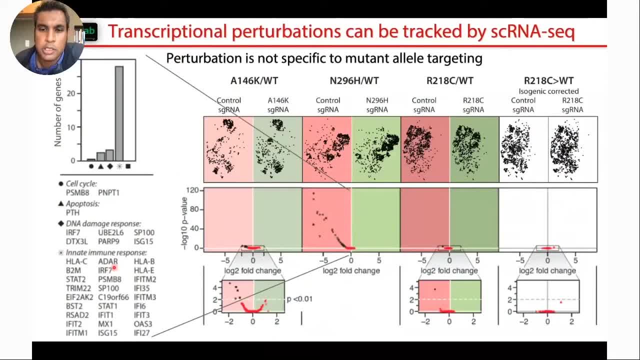 this, but on the old the, the actual going after the mutant allele didn't seem to after the mutant allele didn't seem to. after the mutant allele didn't seem to trigger any trigger, any trigger, any consistent changes across their samples, consistent changes across their samples, consistent changes across their samples. and so i'll stop there and and say that. 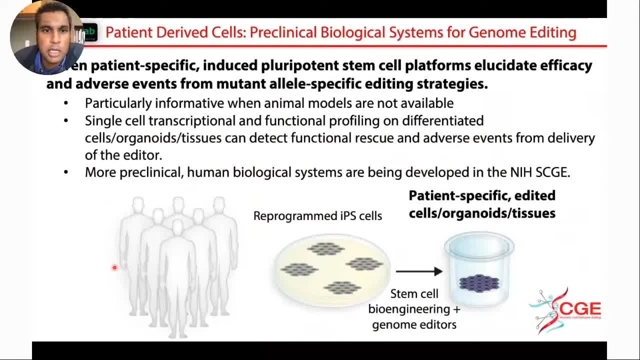 and so i'll stop there and and say that. and so i'll stop there and and say that we- we we had seven patient specific ips lines. it had seven patient specific ips lines. it had seven patient specific ips lines. it helped us, helped us, helped us find information. 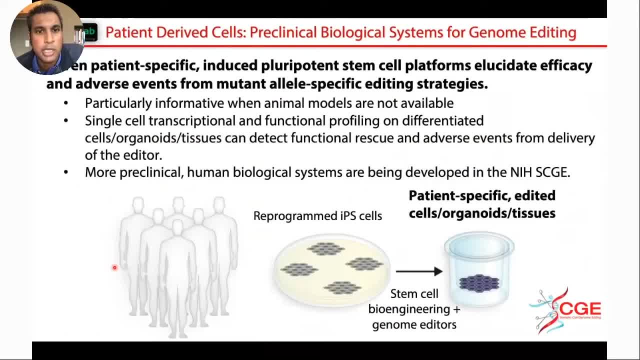 find information. find information in a case where there's no good animal, in a case where there's no good animal, in a case where there's no good animal model. and it gave us model, and it gave us model and it gave us functional information of how cells in 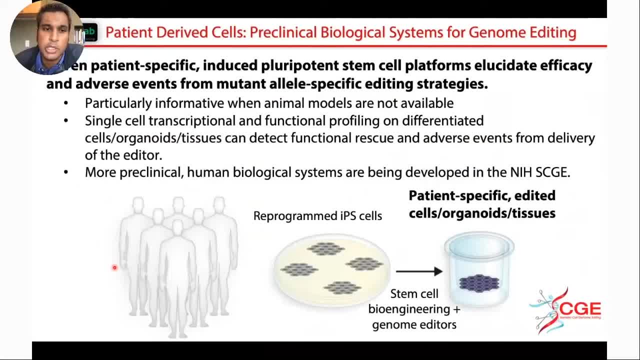 functional information of how cells in functional information, of how cells in this specific cell type would respond to this specific cell type, would respond to this specific cell type, would respond to a particular crispr therapeutic strategy, a particular crispr therapeutic strategy, a particular crispr therapeutic strategy, and i think this is 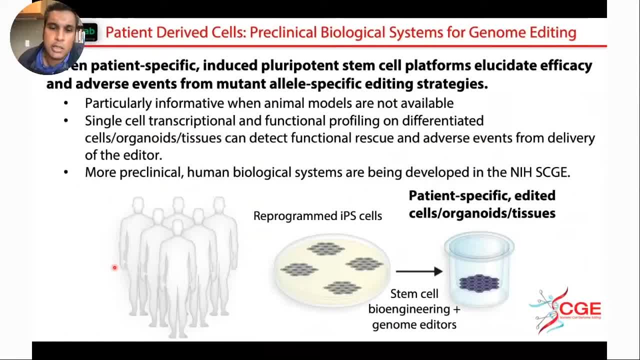 and i think this is, and i think this is a type of techniques that will be a type of techniques that will be a type of techniques that will be scaled up through the scaled up through the scaled up through the somatic cell genome editing consortium. somatic cell genome editing consortium. 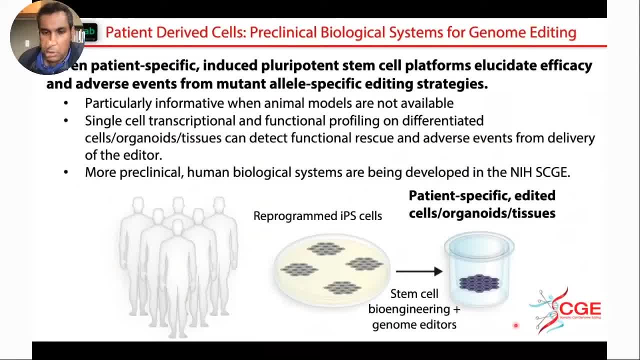 somatic cell genome editing consortium that i mentioned, that i mentioned. that i mentioned, as well as many others in the field, as well as many others in the field, as well as many others in the field. before i sign off, i was i wanted to. before i sign off, i was i wanted to. 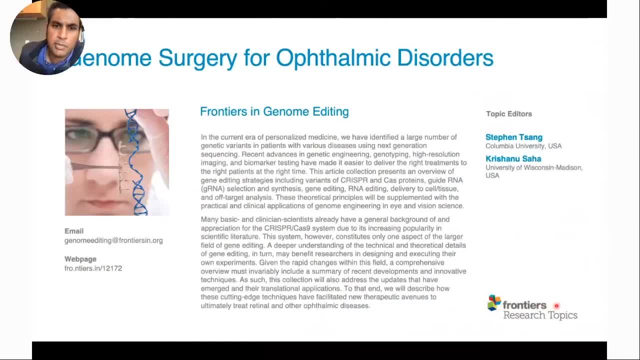 before i sign off, i was. i wanted to highlight this uh special issue. that highlight this uh special issue. that highlight this uh special issue that we're taking uh papers for uh. so we're taking uh papers for uh, so we're taking uh papers for uh. so steven saying at columbia and i are 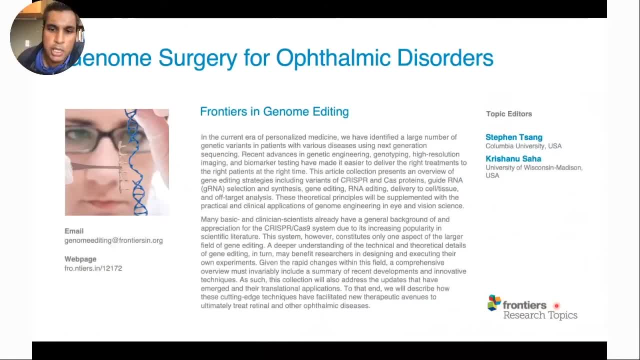 steven saying at columbia and i are steven saying at columbia and i are guest editing this, guest editing this, guest editing this. if you have similar stories in the eye, if you have similar stories in the eye, if you have similar stories in the eye on genome editing. and, lastly, there's a 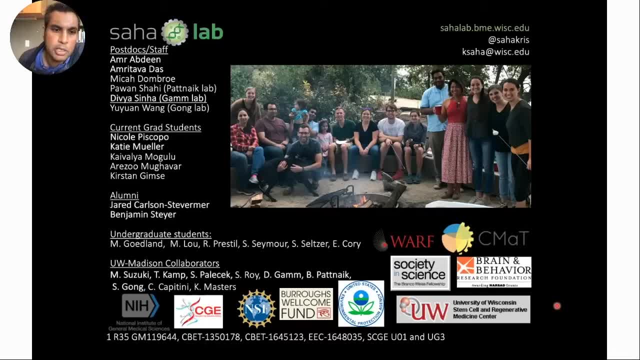 on genome editing and, lastly, there's a on genome editing and, lastly, there's a lot of, lot of great people in the lab that contributed great people in the lab that contributed great people in the lab that contributed to this, namely uh ben stair, who recently 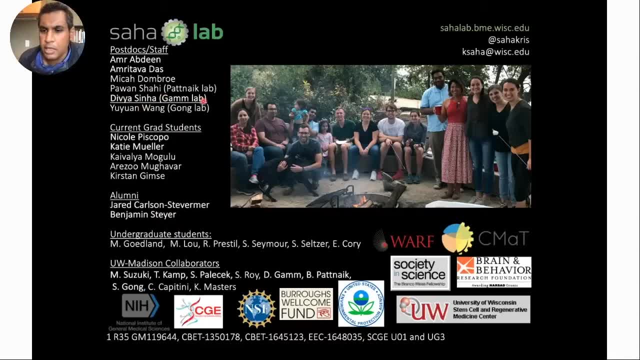 to this, namely uh ben stair. who recently to this? namely uh ben stair, who recently graduated, and dubia sinha graduated. and dubia sinha graduated. and dubia sinha in the gam lab. with that, i'll take uh. in the gam lab. with that, i'll take uh. 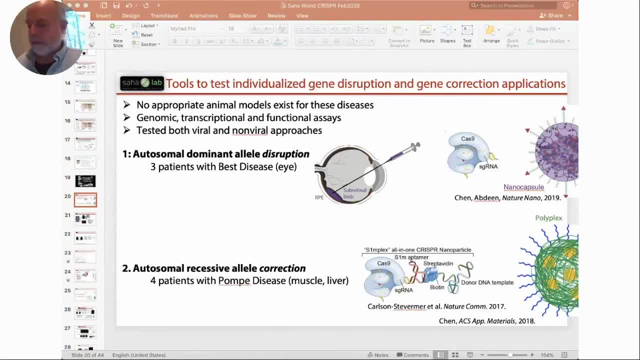 in the gam lab. with that, i'll take uh questions, questions, questions. thank you, chris. thank you, chris. thank you, chris, for a nice talk. so i'm looking at the for a nice talk. so i'm looking at the for a nice talk. so i'm looking at the q a. 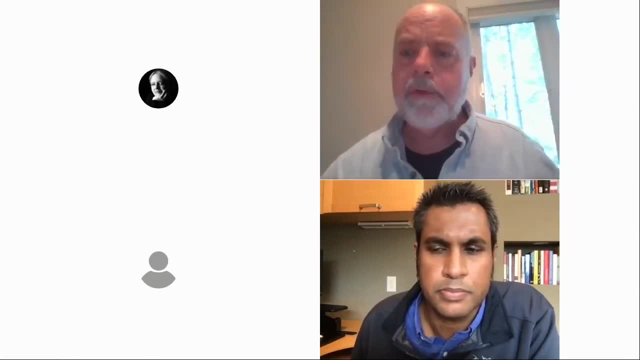 q a, q a. i don't see any questions. i don't see any questions. i don't see any questions specifically for you at this time. you, specifically for you at this time. you, i don't see any questions specifically for you at this time. you may get some later. 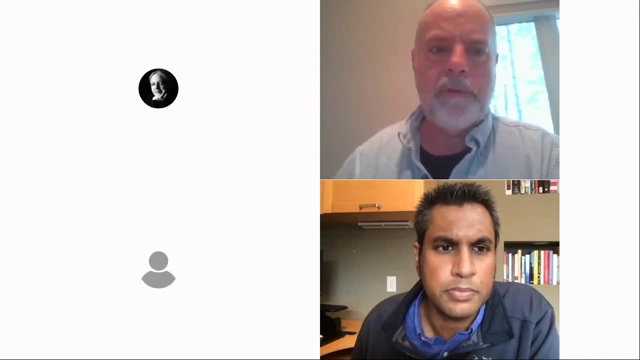 may get some later. may get some later after the talk, and you can answer those after the talk and you can answer those after the talk. and you can answer those um at your leisure, um at your leisure, um at your leisure. so i think we'll move on to our next. 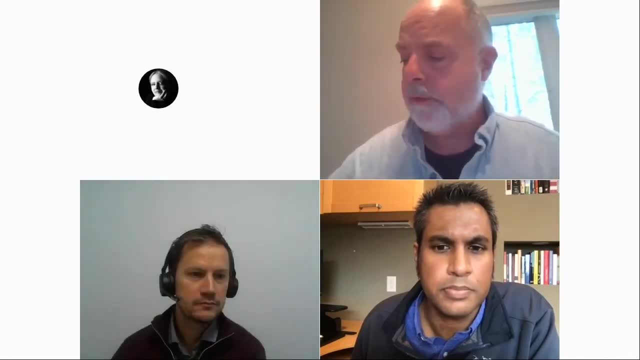 so i think we'll move on to our next. so i think we'll move on to our next speaker, rasmus bach. speaker rasmus bach. speaker rasmus bach, who is an associate professor at uh. who is an associate professor at uh. who is an associate professor at uh aarhus, i hope i'm pronouncing that right. 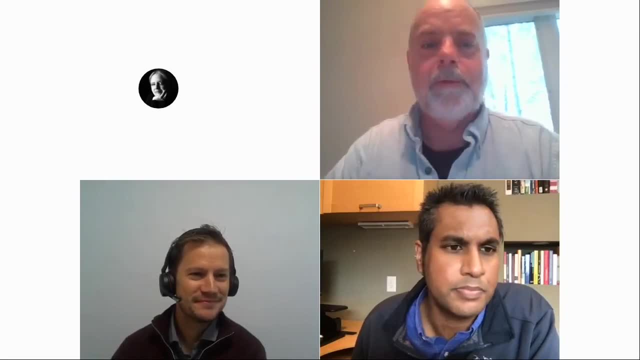 aarhus- i hope i'm pronouncing that right. aarhus, i hope i'm pronouncing that right- aarhus university and aarhus university and aarhus university and denmark, so denmark, so denmark. so a guest from europe, a speaker from europe, a guest from europe, a speaker from europe. 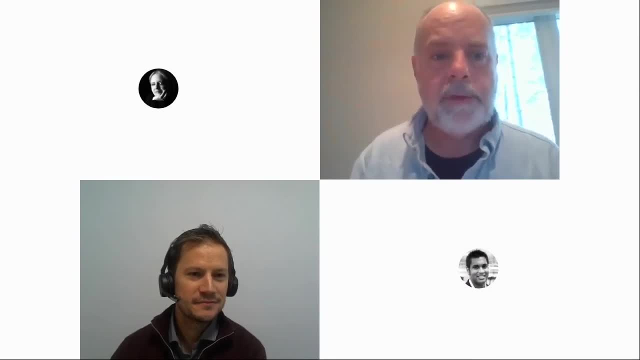 a guest from europe, a speaker from europe, and he's going to tell us about his, and he's going to tell us about his and he's going to tell us about his experiences with crispr. experiences with crispr, experiences with crispr, interference in crispr, activation in. 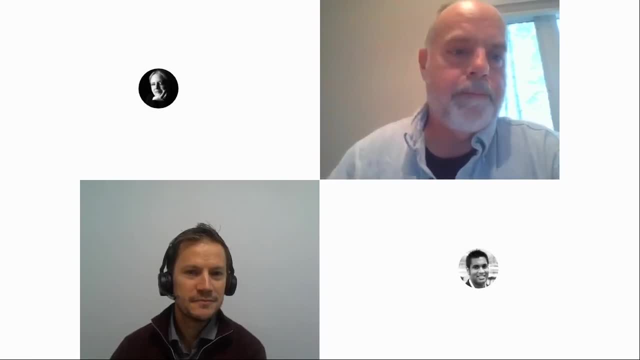 interference in crisper activation in interference in crisper activation in human uh hematopoietic stem cells. great, thank you, bill. great thank you, bill. great thank you, bill. so i'll be talking about crispr. so i'll be talking about crispr. so i'll be talking about crispr activation and crispr inhibition, and 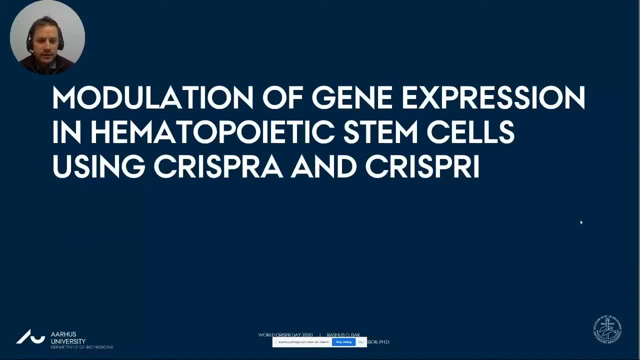 activation and crisper inhibition. and activation and crisper inhibition, and mainly focusing on hematopoietic stem, mainly focusing on hematopoietic stem, mainly focusing on hematopoietic stem cells, but also in in different i'll be- cells, but also in in different i'll be. 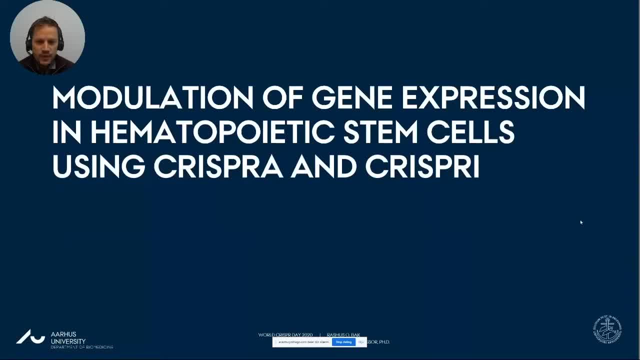 cells, but also in in different. i'll be presenting data from different cell, presenting data from different cell, presenting data from different cell lines in general lines, in general lines in general. i have single disclosure to make, but the. i have single disclosure to make, but the. i have single disclosure to make, but the work i'll be presenting is. 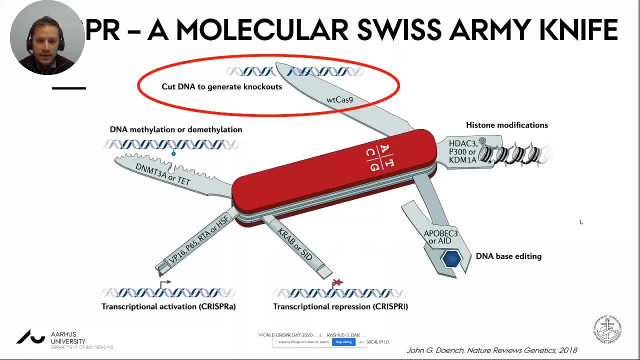 work i'll be presenting is work i'll be presenting is completely from my academic lab, completely from my academic lab, completely from my academic lab. so, as you're probably all aware of, so, as you're probably all aware of, so, as you're probably all aware of, crisper by now is a molecular swiss. 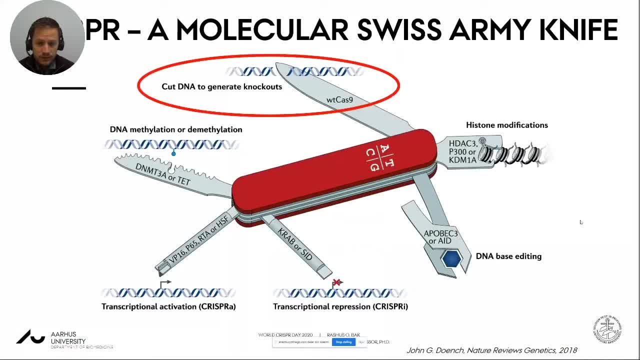 crisper by now is a molecular swiss crisper by now is a molecular swiss army knife. there are so many purposes, army knife. there are so many purposes, army knife. there are so many purposes that you can use this tool for but the that you can use this tool for but the. 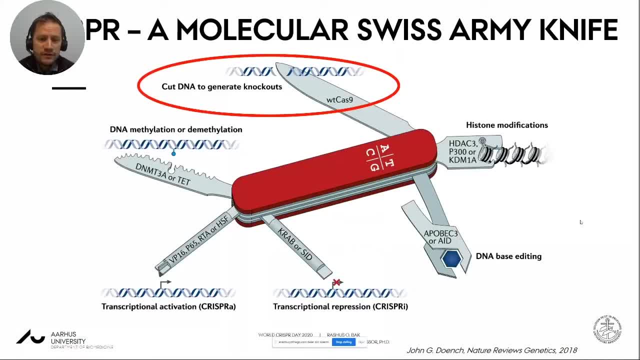 that you can use this tool for, but the, the translational, the translational, the translational. focus of this, focus of this, focus of this tool, is mainly using the function of tool, is mainly using the function of tool, is mainly using the function of generating knockouts or knock-ins. 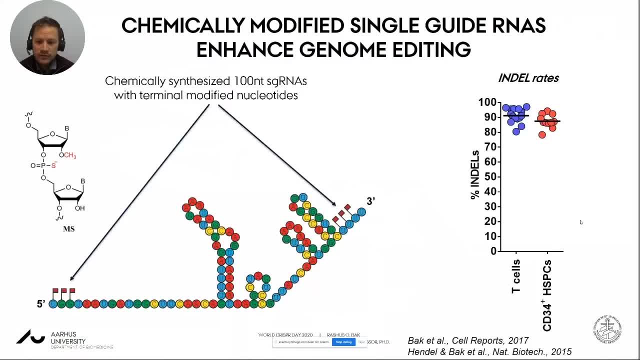 generating knockouts or knock-ins, generating knockouts or knock-ins, and just and just and just to recapitulate from where i'm coming, to recapitulate from where i'm coming, to recapitulate from where i'm coming from: we published. from, we published. 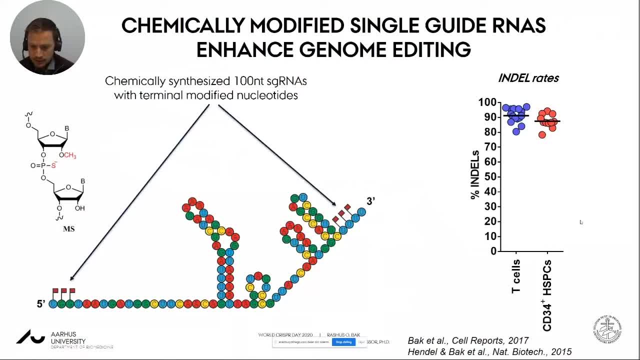 from. we published some work during my postdoc. this is some work during my postdoc. this is some work during my postdoc. this is published in 2015 together with a published in 2015, together with a published in 2015 together with a previous colleague of mine, il hendel. 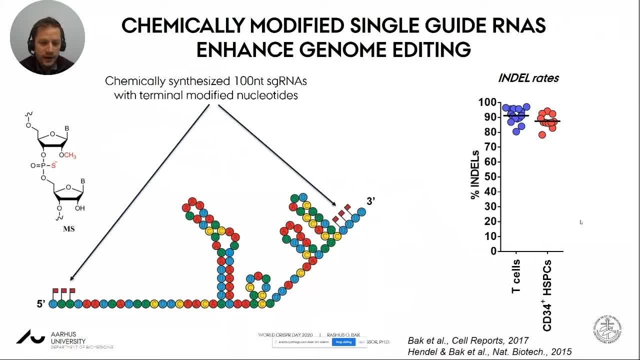 previous colleague of mine, il hendel. previous colleague of mine, il hendel. where we, where we, where we showed that these chemically modified, showed that these chemically modified showed that these chemically modified guide rnas that are protected in both guide rnas that are protected in both. 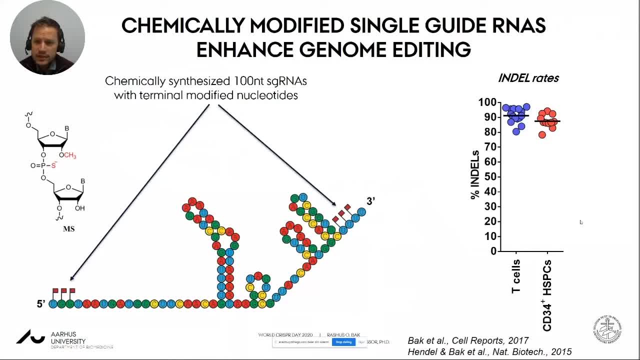 guide rnas that are protected in both ends- ends. ends- can yield very high levels of gene. can yield very high levels of gene. can yield very high levels of gene editing rates, particularly in primary editing rates, particularly in primary editing rates, particularly in primary cells such as t cells and hematopoietic. 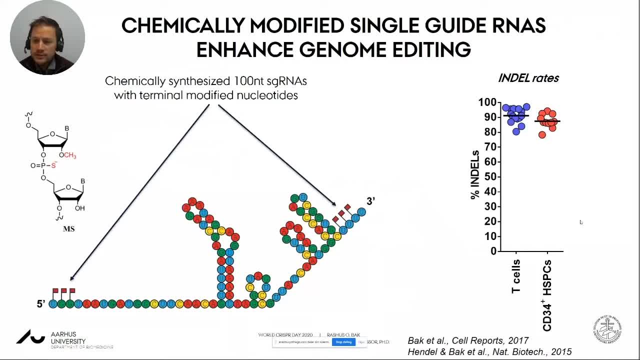 cells, such as t cells, and hematopoietic cells, such as t cells and hematopoietic stem cells. so here is shown data on the stem cells. so here is shown data on the stem cells. so here is shown data on the right right right, getting up to 90- 95 percent of indels. getting up to 90- 95 percent of indels, getting up to 90- 95 percent of indels in these two cell types, in these two cell types, in these two cell types, and we also showed that we could edit and we also showed that we could edit. 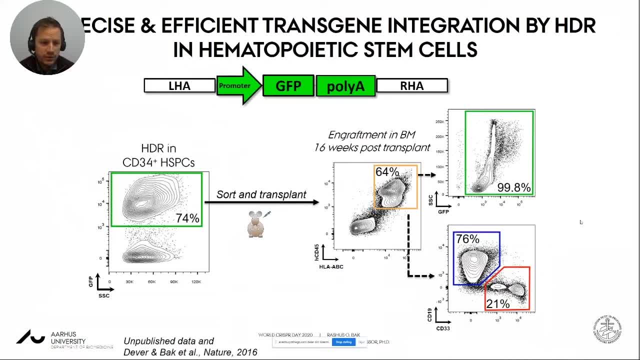 and we also showed that we could edit, edit hematopoietic stem cells. doing edit hematopoietic stem cells. doing edit hematopoietic stem cells. doing targeted knock-in here. targeted knock-in here. targeted knock-in here. showing gfp reported gene knock-in into. 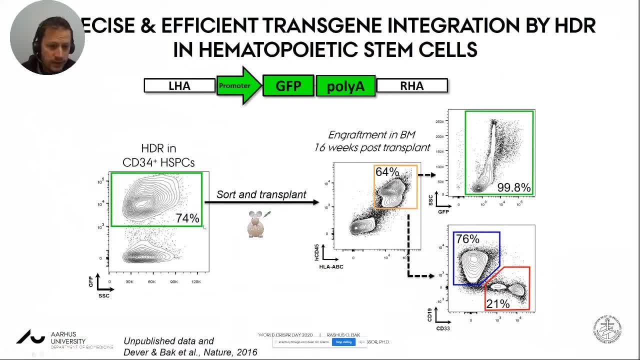 showing gfp reported gene knock-in into. showing gfp reported gene knock-in into hematopoietic stem cells, in this case hematopoietic stem cells, in this case hematopoietic stem cells, in this case getting high rates and this particular getting high rates and this particular. 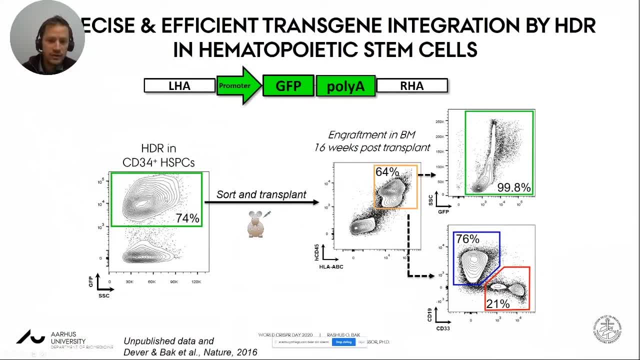 getting high rates and this particular donor of 74, donor of 74, donor of 74 target integration, we can sort out all target integration. we can sort out all target integration. we can sort out all these green, these green, these green stem and progenitor cells, transplant them. 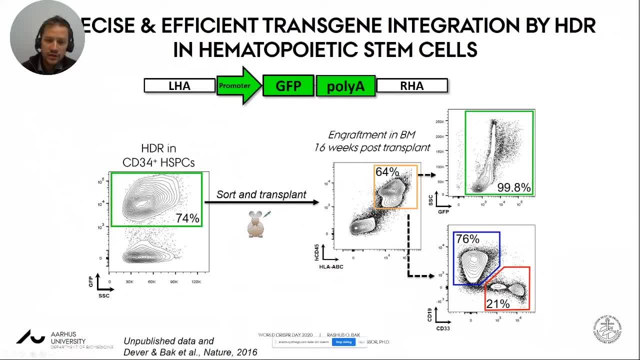 stem and progenitor cells, transplant them. stem and progenitor cells, transplant them into an immunodeficient mouse, into an immunodeficient mouse, into an immunodeficient mouse. and after four months in a mouse, we can, and after four months in a mouse, we can, and after four months in a mouse we can see that there is human chimerism in the. 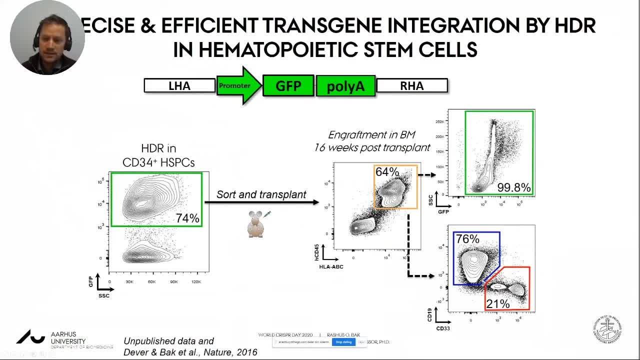 see that there is human chimerism in the see, that there is human chimerism in the bone marrow, and all the cells are still bone marrow and all the cells are still bone marrow and all the cells are still green and the cells still give rise to. 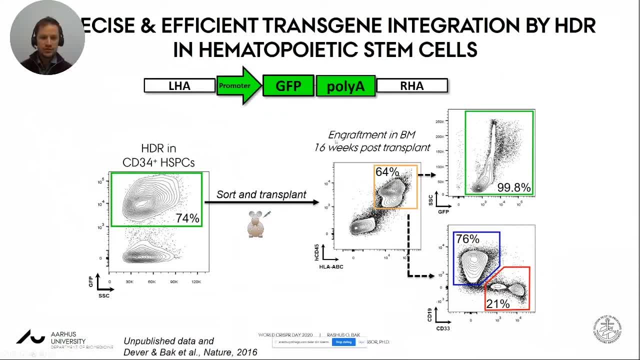 green and the cells still give rise to green and the cells still give rise to multi-lineage repopulation, multi-lineage repopulation, multi-lineage repopulation. so, just showing that this system is very so, just showing that this system is very so, just showing that this system is very potent with the chemically modified 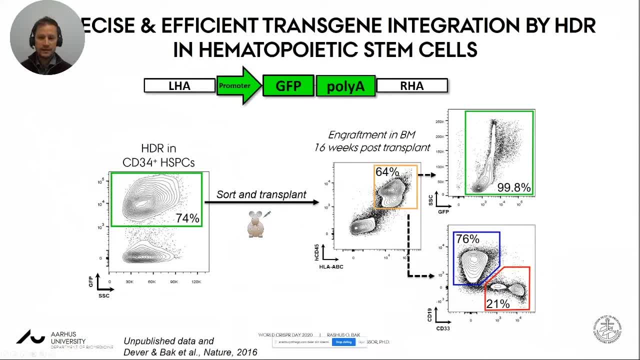 potent with the chemically modified? potent with the chemically modified guide rnas in a highly clinical setting, guide rnas in a highly clinical setting, guide rnas in a highly clinical setting. and this is exactly what. and this is exactly what, and this is exactly what matt portia showed some data from in a. 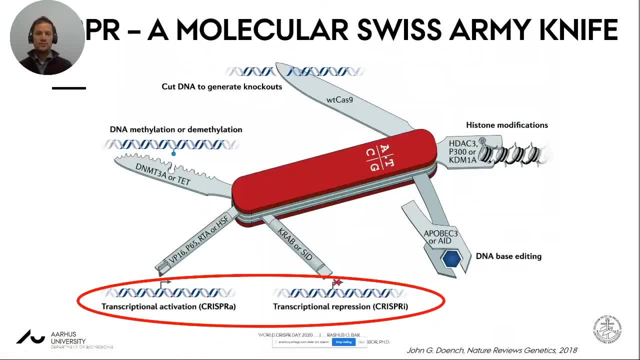 matt portia showed some data from in a. matt portia showed some data from in a previous session, previous session, previous session. so coming back to the swiss army knife, so coming back to the swiss army knife. so coming back to the swiss army knife, we've now turned our focus on 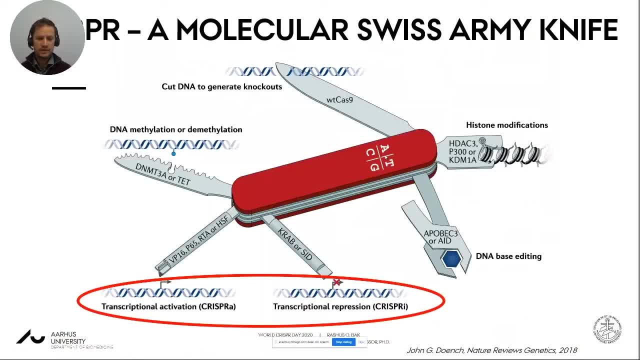 we've now turned our focus on. we've now turned our focus on on some of the other derived technologies, on some of the other derived technologies, on some of the other derived technologies: mainly the crispr activation and crispr, mainly the crispr activation and crispr. 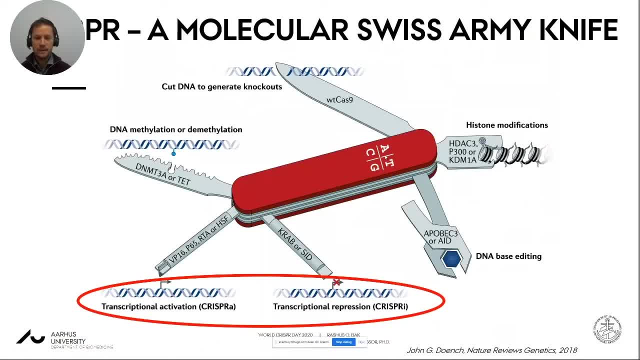 mainly the crispr activation and crispr inhibition, inhibition, inhibition or repression interference technologies, if, or repression interference technologies, if, or repression interference technologies, if you will, you will, you will trying to apply some of the same, trying to apply some of the same, trying to apply some of the same principles to this. 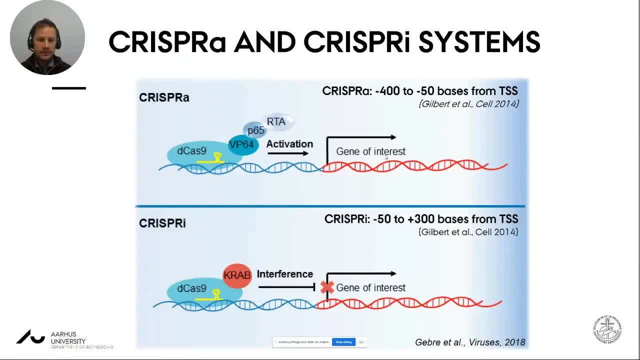 principles to this, principles to this, and it's these tools are very, very and it's these tools are very, very and it's these tools are very, very simple, simple, simple. you deactivate the catalytic function of you deactivate the catalytic function of you deactivate the catalytic function of a domain or several domains, that it will. 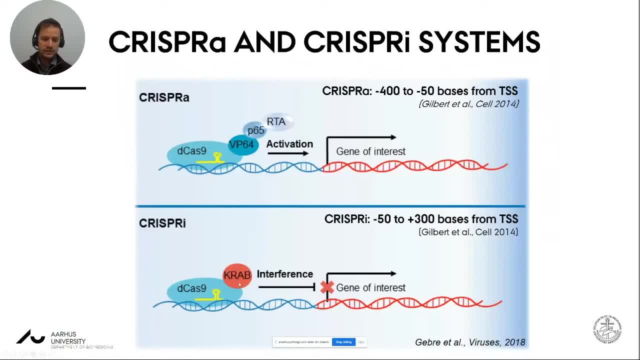 a domain or several domains that it will. a domain or several domains that it will facilitate activation, or it can be facilitate activation, or it can be facilitate activation, or it can be a transcriptionally interfering domain, a transcriptionally interfering domain, a transcriptionally interfering domain, and then you target. 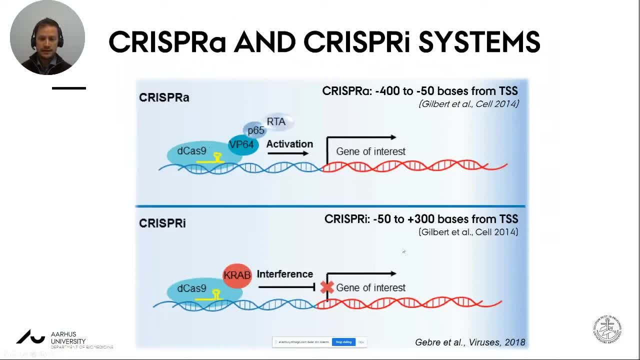 and then you target, and then you target this, uh, these complexes to this, uh, these complexes to this, uh, these complexes to a site close to the transcriptional start, a site close to the transcriptional start, a site close to the transcriptional start side. here is sort of 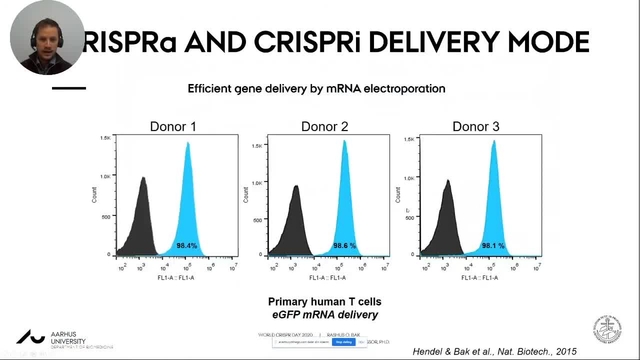 side. here is sort of side. here is sort of the rules that we have stuck to and and and to, to to get high rates, or at least hope to get get high rates, or at least hope to get get high rates or at least hope to get high rates in some of the primary cells. 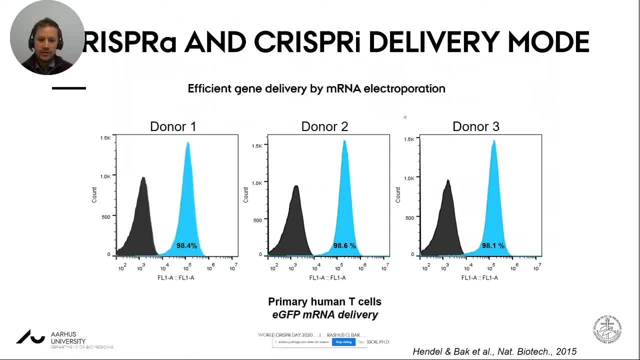 high rates in some of the primary cells, high rates in some of the primary cells, that can be very difficult to that can be very difficult, to that can be very difficult to deliver genetic material to return our deliver genetic material, to return our deliver genetic material. to return our attention to also some previous data. 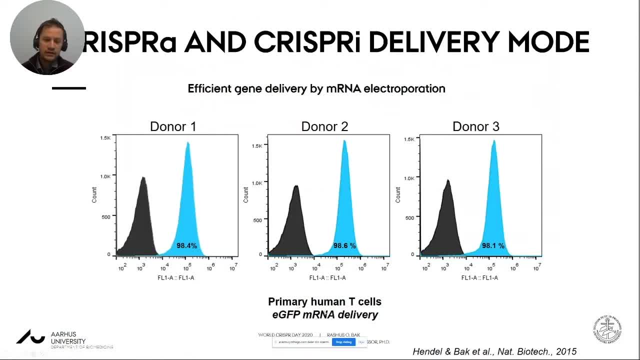 attention to also some previous data. attention to also some previous data here showing that in primary human t here. showing that in primary human t here, showing that in primary human t cells we can get very high delivery of cells. we can get very high delivery of cells. we can get very high delivery of messenger rna to these cells. so almost 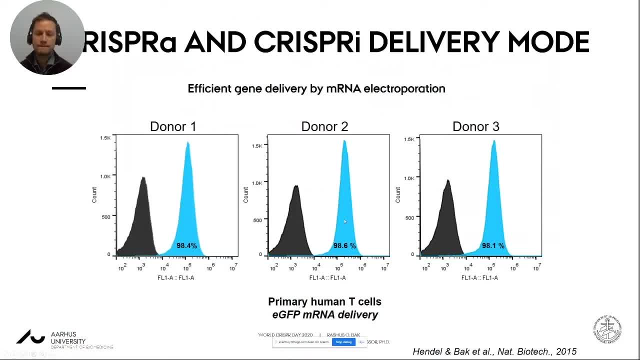 messenger rna to these cells. so almost messenger rna to these cells. so almost all the cells are transfected and all the cells are transfected and all the cells are transfected and expressing high levels of the trans, expressing high levels of the trans, expressing high levels of the trans gene. 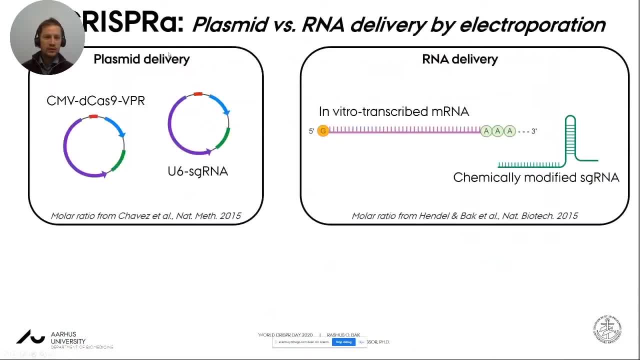 so initially i'll just focus on crisper. so initially i'll just focus on crisper. so initially i'll just focus on crisper. activation and what activation and what activation and what many studies have used, as either many studies have used as either many studies have used as either plasmid delivery for this system or 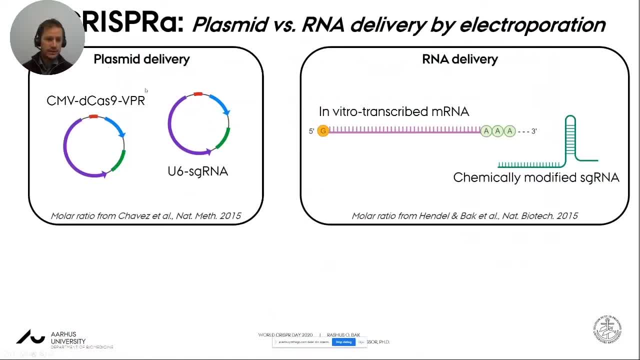 plasmid delivery for this system, or plasmid delivery for this system. or lentiviral delivery of m for. for lentiviral delivery of m for. for lentiviral delivery of m for, for example, library screens, example library screens, example library screens. so we wanted to compare an rna delivery. 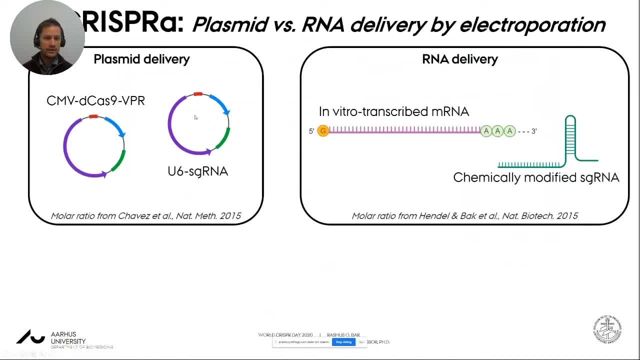 so we wanted to compare an rna delivery. so we wanted to compare an rna delivery strategy to a plasma delivery strategy, to a plasma delivery strategy to a plasma delivery strategy. so the plasma strategy is strategy, so the plasma strategy is strategy. so the plasma strategy is a two-part system, two plasmids or it. 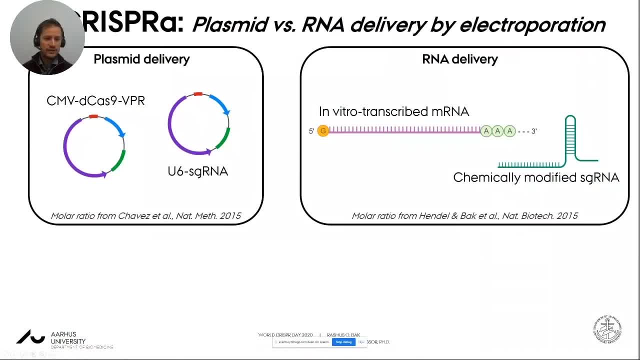 a two-part system, two plasmids, or it a two-part system, two plasmids, or it might be several plasmids. because in might be several plasmids? because in might be several plasmids? because in most settings we're using four guide. 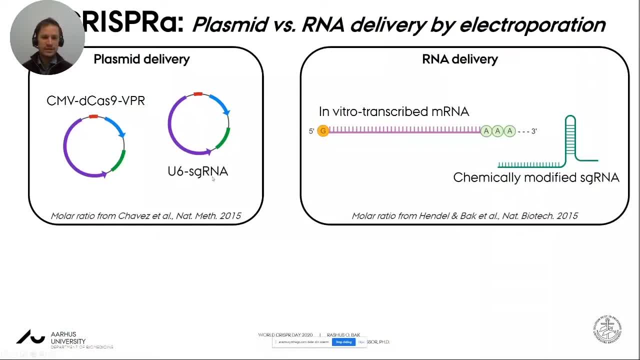 most settings. we're using four guide most settings. we're using four guide RNAs targeting the same RNAs targeting the same RNAs targeting the same locus or the same site in the promoter locus or the same site in the promoter locus or the same site in the promoter. just before the transcription start. 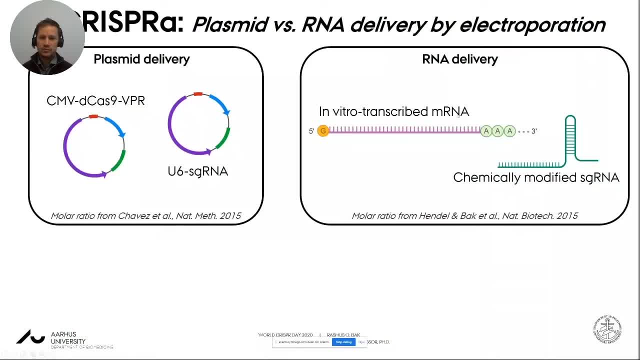 just before the transcription start. just before the transcription start side: and and for the rna delivery side, and and for the rna delivery side and and for the rna delivery system. we're making in vitro transcribed system. we're making in vitro transcribed system, we're making in vitro transcribed messenger RNA and co-delivering that. 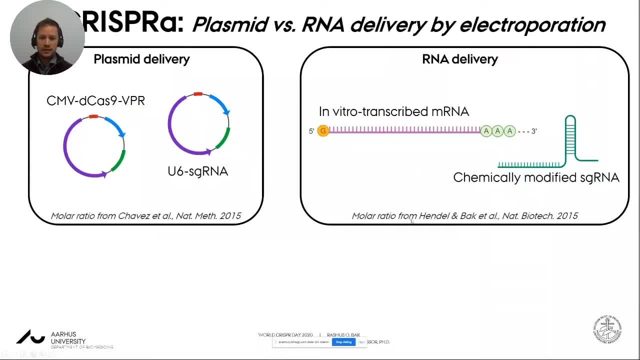 messenger RNA and co-delivering that messenger RNA and co-delivering that with chemically modified guide RNAs, with chemically modified guide RNAs, with chemically modified guide RNAs. looking at some molar ratios that we. looking at some molar ratios that we. 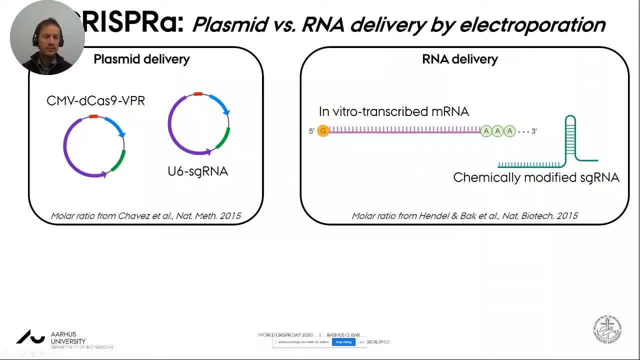 looking at some molar ratios that we previously devised and these smaller, previously devised. and these smaller, previously devised. and these smaller ratios were also devised from a previous ratios were also devised from a previous ratios were also devised from a previous publication, publication, publication, um, um, um. so this is the 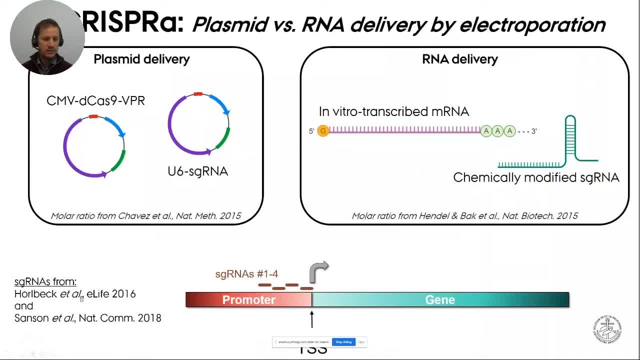 so this is the. so this is the basic setup. the guide RNA design is basic setup. the guide RNA design is basic setup. the guide RNA design is from previous publications, where they from previous publications, where they from previous publications where they designed highly optimized, designed, highly optimized, designed, highly optimized libraries for CRISPR activation and also. 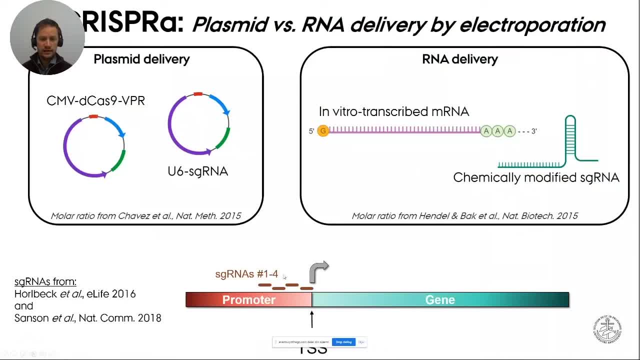 libraries for CRISPR activation and also libraries for CRISPR activation. and also interference, and this is the general interference and this is the general interference and this is the general concept of tiling, concept of tiling, concept of tiling mainly for guide RNAs right around the 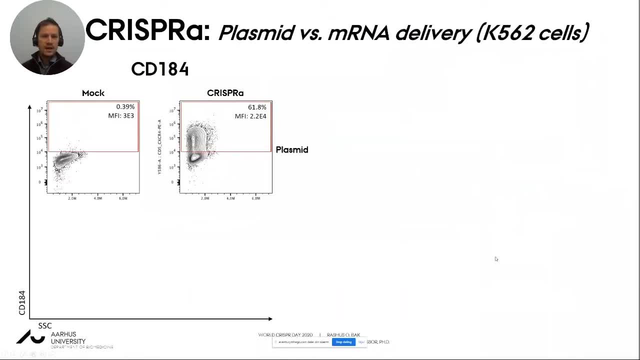 mainly for guide RNAs right around the mainly for guide RNAs right around the promoter region, at the transcriptional promoter region, at the transcriptional promoter region, at the transcriptional start site, start site, start site, and we focused on and we focused on and we focused on proteins or genes that are expressed. 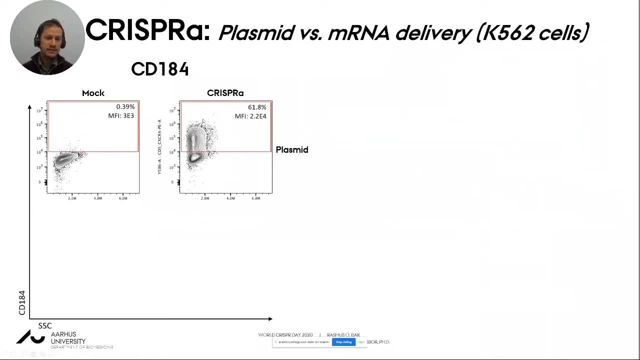 proteins or genes that are expressed. proteins or genes that are expressed on the surface of the, on the surface of the, on the surface of the cells. that we can analyze this by flow cells. that we can analyze this by flow cells. that we can analyze this by flow cytometry, thereby having a single cell. 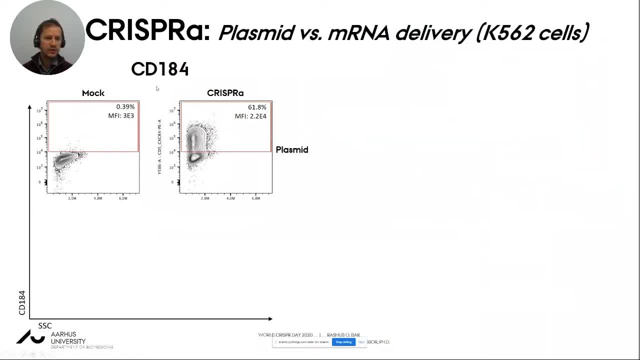 cytometry, thereby having a single cell cytometry, thereby having a single cell resolution, and this is experiment resolution. and this is experiment resolution and this is experiment targeting cd184 cxcr4, targeting cd184 cxcr4, targeting cd184 cxcr4 protein. using the plasmid system, we can. 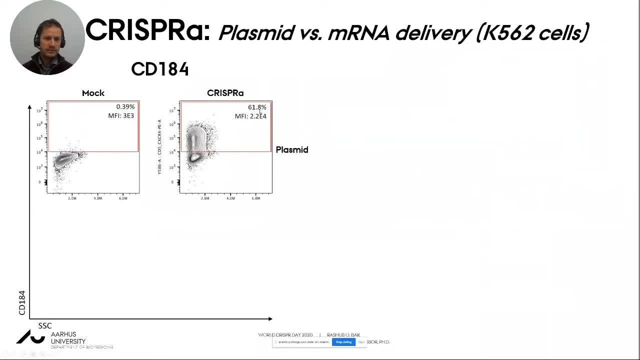 protein using the plasmid system. we can protein using the plasmid system. we can see that we get nice up regulation with see that we get nice up regulation with. see that we get nice up regulation with a, a, a: 62 percent of the cells now expressing a. 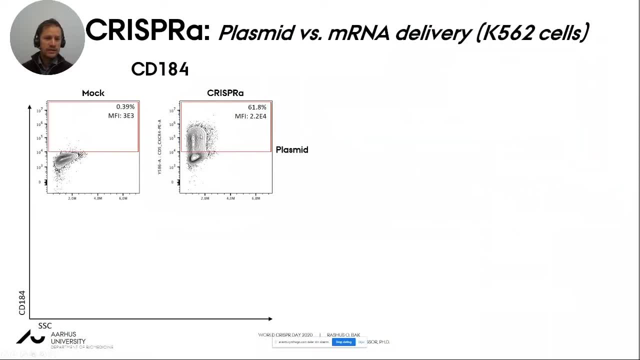 62 percent of the cells now expressing a 62 percent of the cells now expressing a gene that was previously completely gene that was previously completely gene that was previously completely suppressed, suppressed, suppressed. you also notice here that, for you see, you also notice here that for you see a highly heterogeneous population of 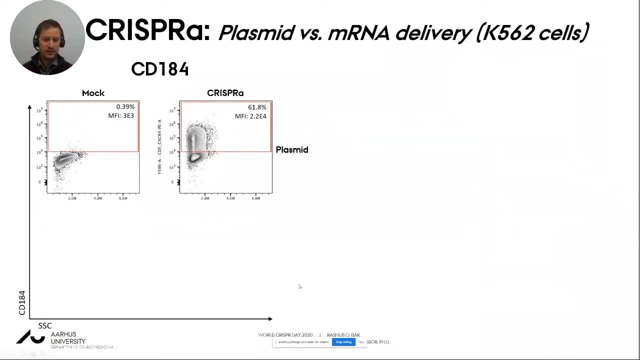 a highly heterogeneous population of a highly heterogeneous population of cells that express this gene. so when we cells that express this gene, so when we cells that express this gene, so when we instead delivered, and this is all instead delivered, and this is all instead delivered, and this is all delivery by electroporation, when we 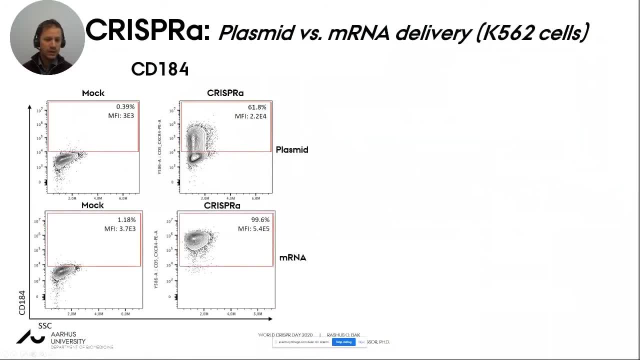 delivery by electroporation. when we delivery by electroporation, when we deliver it using an all rna system, you deliver it using an all rna system. you deliver it using an all rna system. you can see that, can see that, can see that we're getting really homogeneous levels. 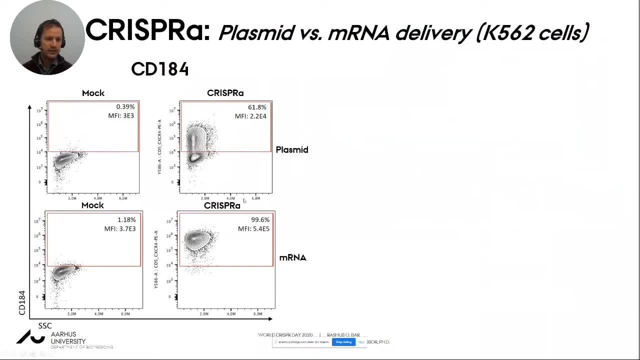 we're getting really homogeneous levels. we're getting really homogeneous levels of activation here and also a bit higher of activation here, and also a bit higher of activation here and also a bit higher, at least on average, than the plasmid, at least on average, than the plasmid. 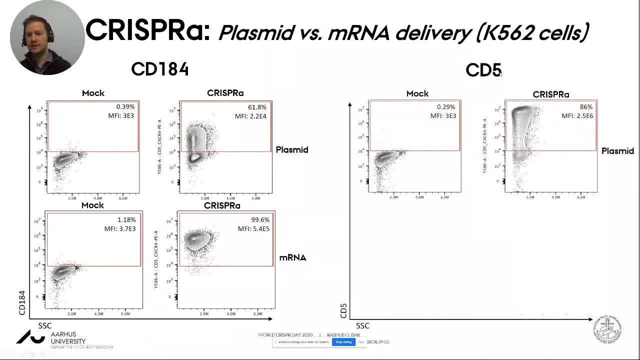 at least on average than the plasmid based system. this is for cxcr4 as i based system. this is for cxcr4 as i based system. this is for cxcr4 as i mentioned. targeting cd5 crispr activation mentioned targeting cd5 crispr activation. 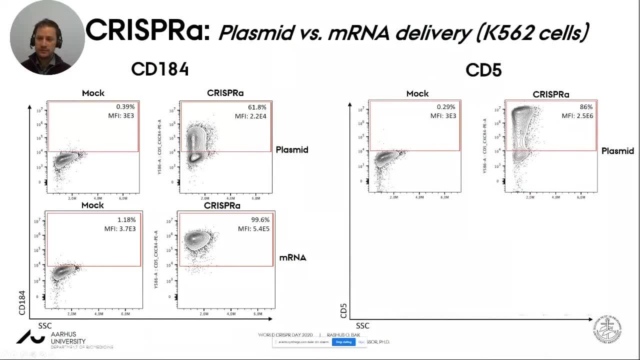 mentioned targeting cd5 crispr. activation by plasmid delivery works a little. by plasmid delivery works a little by plasmid delivery works a little better. 86 percent of the cells are better. 86 percent of the cells are better. 86 percent of the cells are positive, but again heterogeneously. 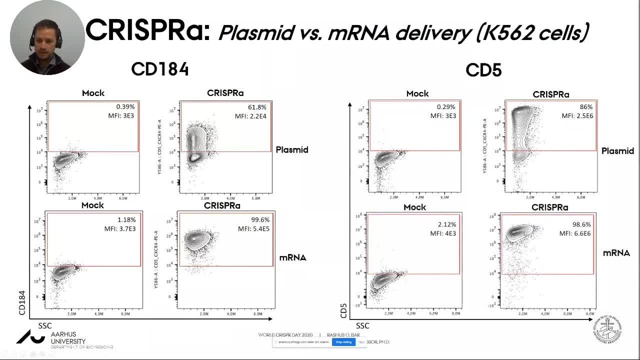 positive, but again heterogeneously positive, but again heterogeneously upregulated, upregulated, upregulated for the messenger RNA system. it looks for the messenger RNA system. it looks for the messenger RNA system. it looks much more homogeneous, much more homogeneous, much more homogeneous. so this was a quite striking difference. 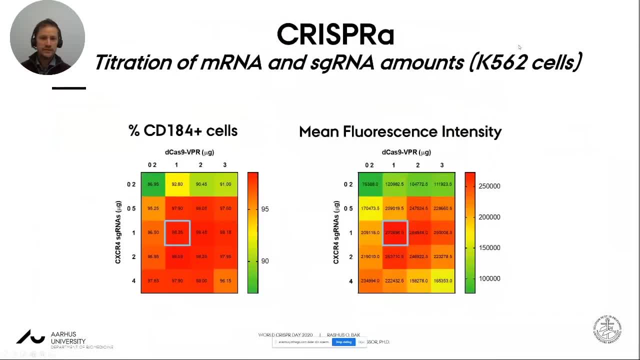 so this was a quite striking difference. so this was a quite striking difference and looked very promising. this is in and looked very promising. this is in and looked very promising. this is in: k562 cells, which i- i should emphasize, k562 cells, which i- i should emphasize. 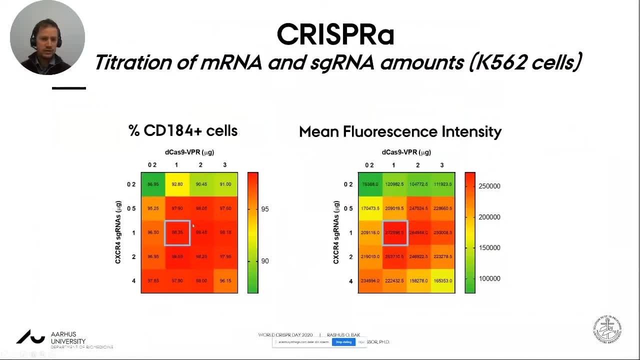 k562 cells, which i, i should emphasize- we also wanted to make sure that, for we also wanted to make sure that, for we also wanted to make sure that, for this application of the crispr system, we, this application of the crispr system, we, this application of the crispr system, we were still at an optimal, uh, at optimal. 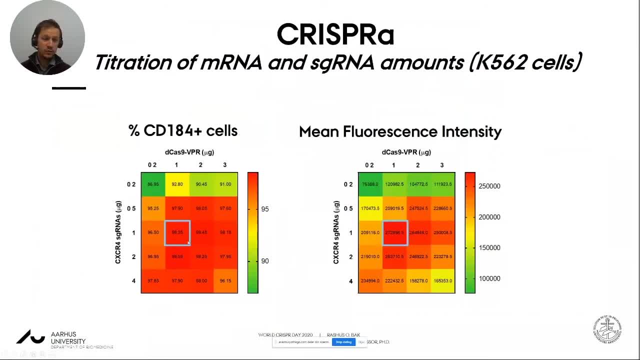 were still at an optimal uh, at optimal, were still at an optimal uh, at optimal levels of the guide RNAs and the and the levels of the guide RNAs and the and the levels of the guide RNAs and the and the messenger RNA. and we were in fact 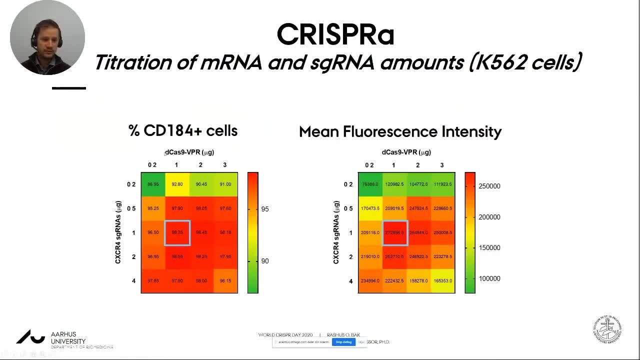 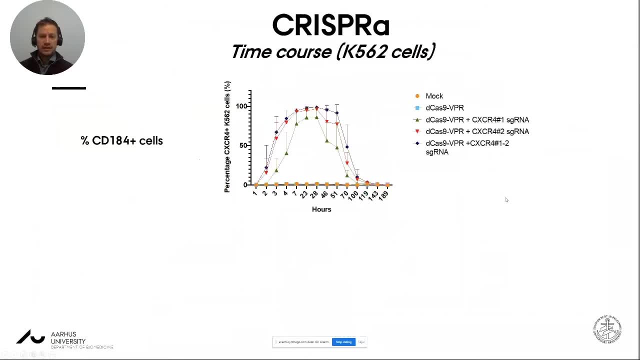 messenger RNA and we were in fact, messenger RNA and we were in fact hitting just the sweet spot of hitting just the sweet spot of hitting just the sweet spot of numerical scale, numerical scale, numerical scale. we get really high levels of, we get really high levels of, we get really high levels of operation very fast within four hours. 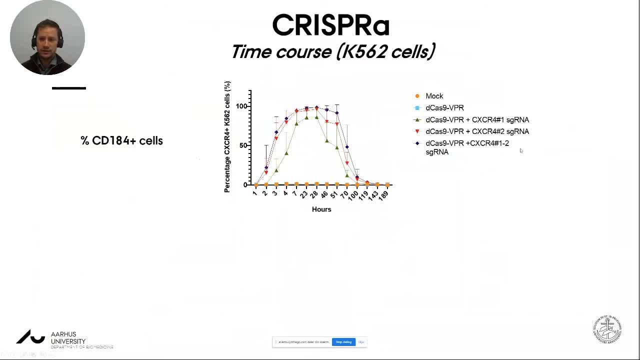 operation very fast within four hours. operation very fast within four hours. you get almost high full. you get almost high full. you get almost high full. upregulation: this is using either one upregulation. this is using either one upregulation. this is using either one guide: RNA targeting cxcr4, a different. 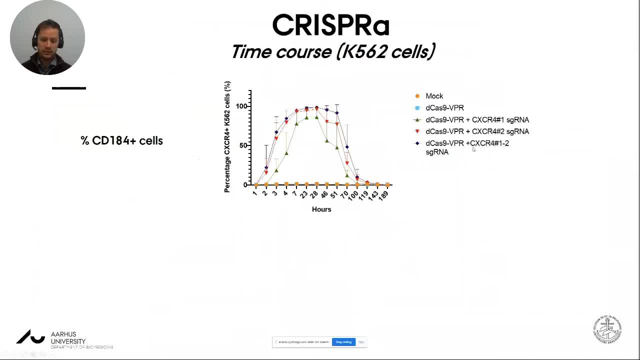 guide RNA targeting cxcr4. a different guide RNA targeting cxcr4, a different guide RNA or the two guide RNAs- guide RNA or the two guide RNAs guide RNA or the two guide RNAs combined. so this is not a four guide combined. so this is not a four guide. 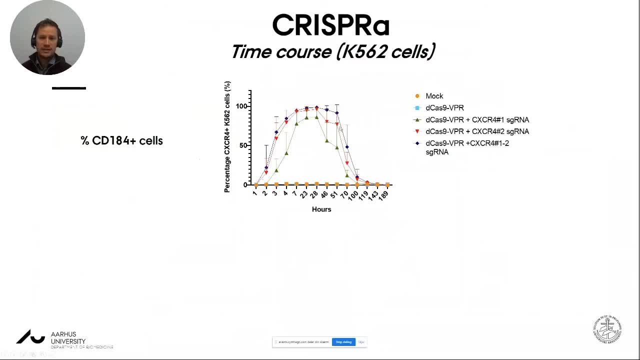 combined. so this is not a four guide RNA system but only a two guide RNA RNA system, but only a two guide RNA RNA system, but only a two guide RNA system. and you can see that the guide system and you can see that the guide system and you can see that the guide RNA2 gives almost the same up. 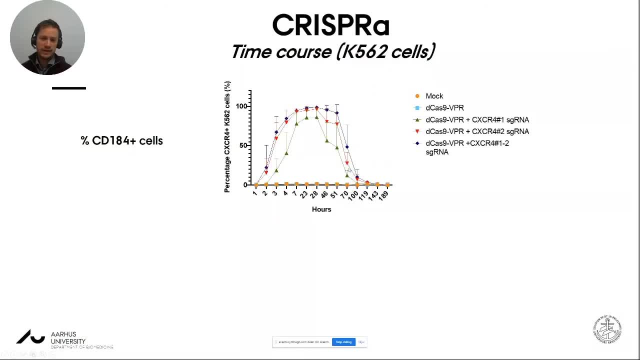 RNA2 gives almost the same up. RNA2 gives almost the same up. regulation as both of them combined. regulation as both of them combined. regulation as both of them combined, and it wears off, and it wears off, and it wears off after about four days. if you look at the 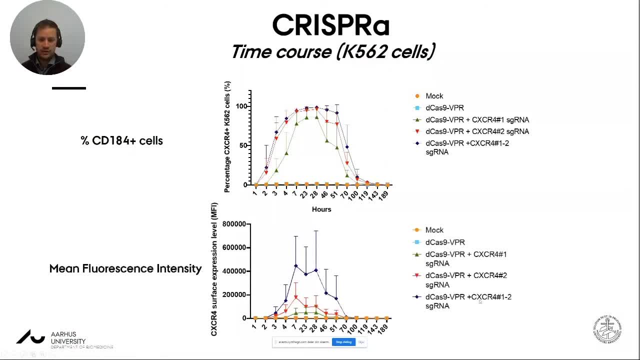 after about four days. if you look at the after about four days. if you look at the mean for essence intensity- mean for essence intensity, mean for essence intensity- you'll see a higher difference between, you'll see a higher difference between. you'll see a higher difference between the. 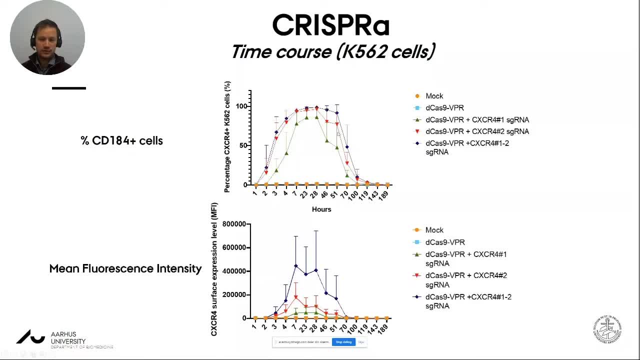 the, the commentatorial guide RNA and and the commentatorial guide RNA and and the commentatorial guide RNA and and the guide RNA2. that was very guide RNA2, that was very guide. RNA2. that was very high degree of operation by only high degree of operation by only. 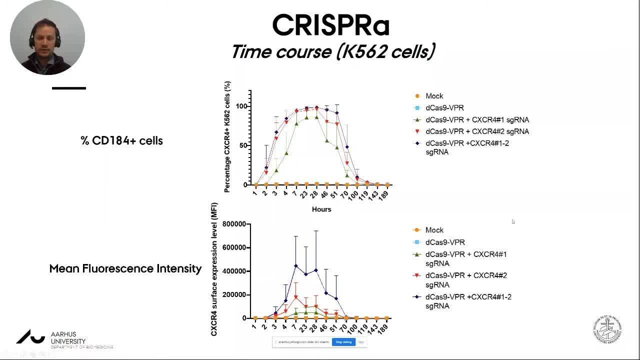 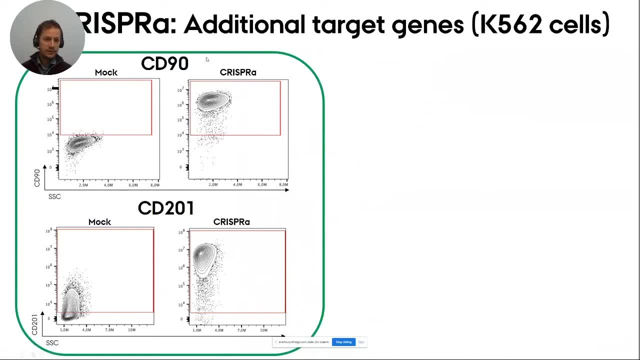 high degree of operation by only including a single guide RNA or a including a single guide RNA or a including a single guide RNA or a less potent guide RNA. less potent guide RNA. less potent guide RNA. so we turned, so we turned, so we turned towards several targets that were still 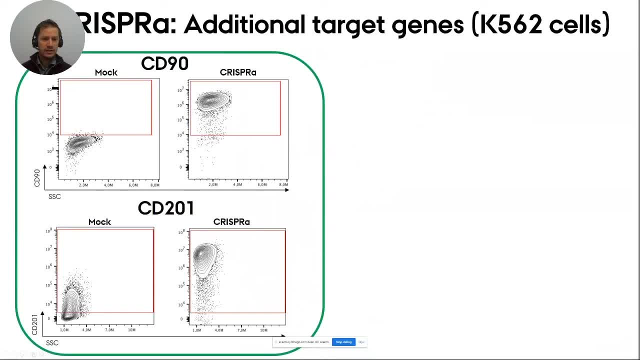 towards several targets that were still towards several targets that were still expressed on the surface of the cells, expressed on the surface of the cells, expressed on the surface of the cells. this is data from cd90 up regulation, and this is data from cd90 up regulation, and 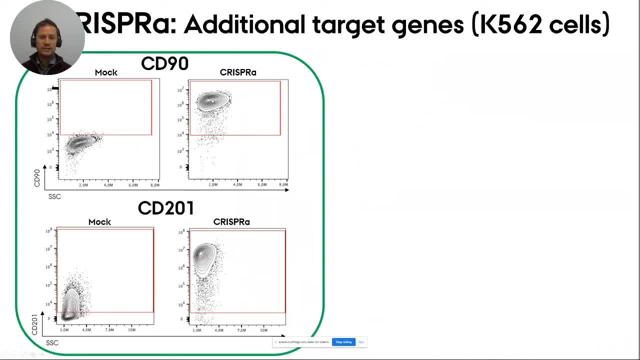 this is data from cd90 up regulation and cd201, cd201, cd201- again seeing really potent up regulation, again seeing really potent up regulation, again seeing really potent up regulation of these two genes, of these two genes, of these two genes. but we also observed genes that were 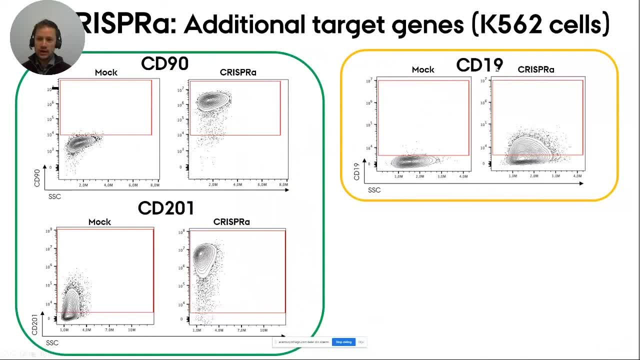 but we also observed genes that were. but we also observed genes that were more difficult to up regulate. this is more difficult to up regulate. this is more difficult to up regulate. this is using four guides targeting the promoter. using four guides targeting the promoter. using four guides targeting the promoter of cd19. 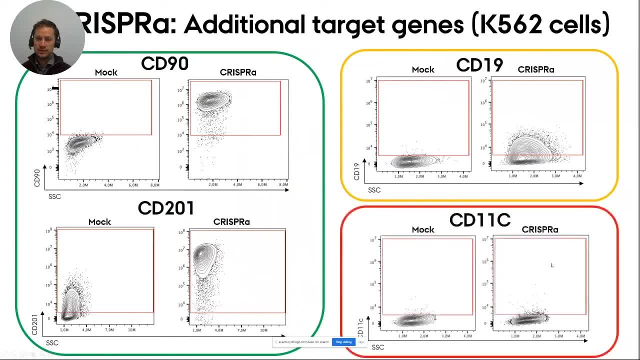 of cd19, of cd19, where we only see a suboptimal up, where we only see a suboptimal up, where we only see a suboptimal up. regulation, and we also regulation, and we also regulation, and we also noticed genes that didn't display any. 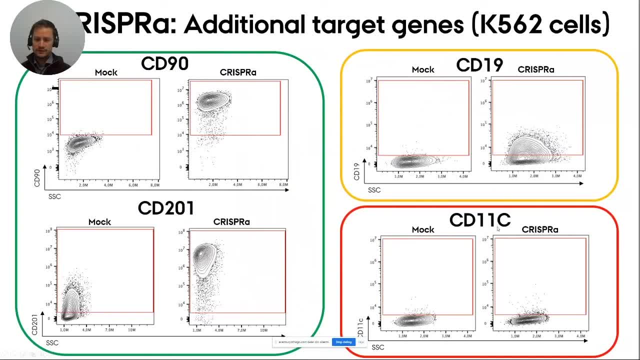 noticed genes that didn't display any noticed genes that didn't display any up regulation at all up regulation at all up regulation at all. so that was a bit of a surprise to us. so that was a bit of a surprise to us. so that was a bit of a surprise to us. and why this didn't work. it could be the. 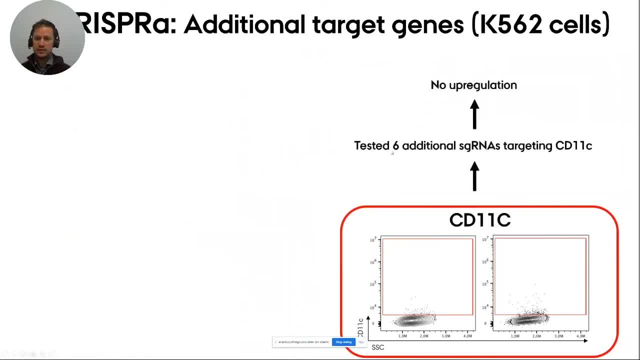 and why this didn't work. it could be the and why this didn't work. it could be the four guides that we had chosen for this, four guides that we had chosen for this, four guides that we had chosen for this particular gene. so we screened six particular gene, so we screened six. 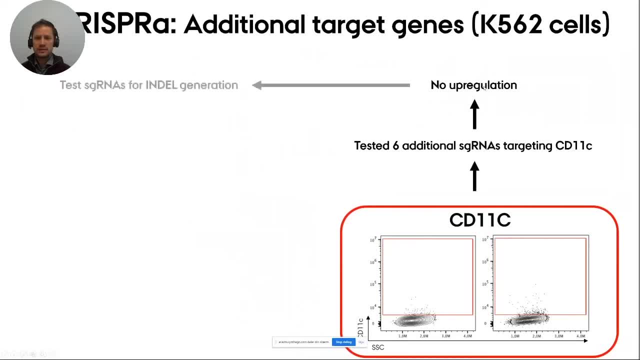 particular gene. so we screened six additional guide rnas around the same additional guide rnas around the same additional guide rnas around the same site. still didn't see any up regulation site. still didn't see any up regulation site. still didn't see any up regulation. so we tested all 10 guide rnas to see if. 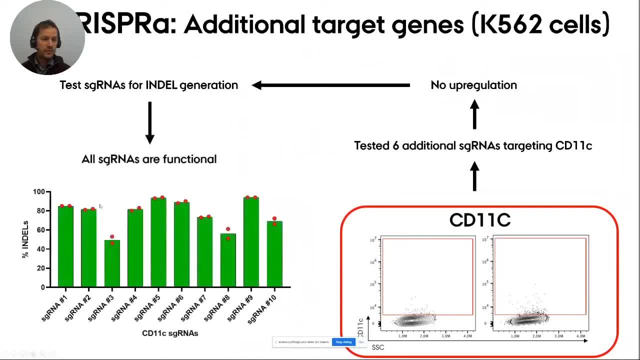 so we tested all 10 guide rnas to see. if so, we tested all 10 guide rnas to see if they were functional. just for they were functional, just for they were functional, just for generating indels in the genome and in generating indels in the genome. and in fact they were all functional. 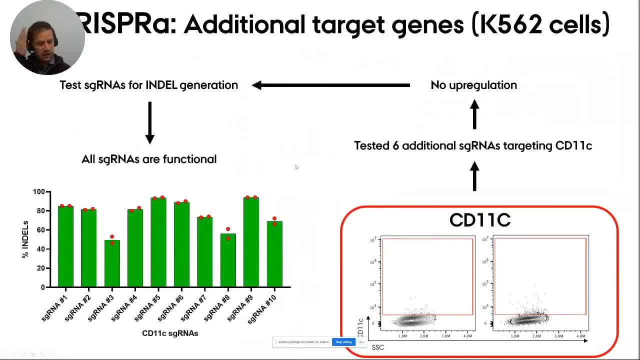 fact, they were all functional. fact, they were all functional. so that's where we are now with this gene. so that's where we are now with this gene. so that's where we are now with this gene. we, we can't seem to up regulate it. we, we can't seem to up regulate it. 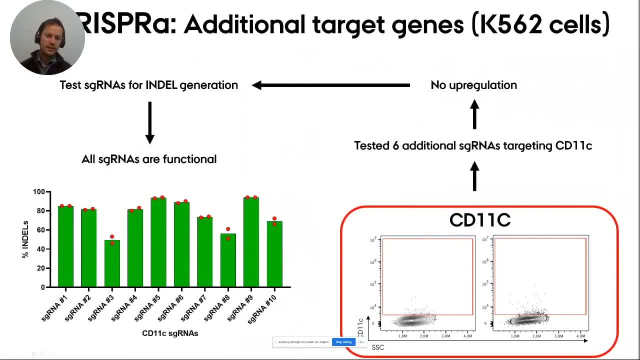 we, we can't seem to up regulate it- and and of course, thoughts, and, and of course, thoughts and, and of course thoughts would go towards the epigenetic state of, would go towards the epigenetic state of, would go towards the epigenetic state of this gene that might influence. 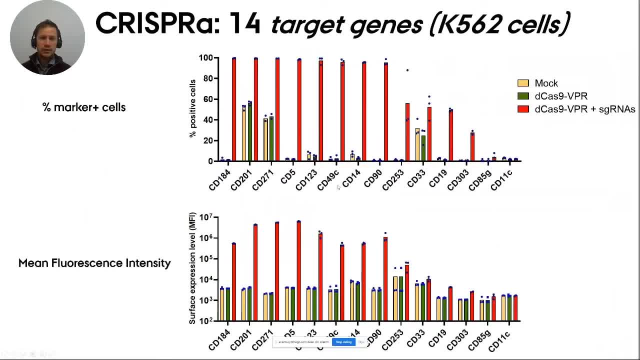 this gene that might influence this gene that might influence this. so this is just this. so this is just this. so this is just showing all 14 target genes, that we showing all 14 target genes, that we showing all 14 target genes that we screen in k562 cells. we see high up. 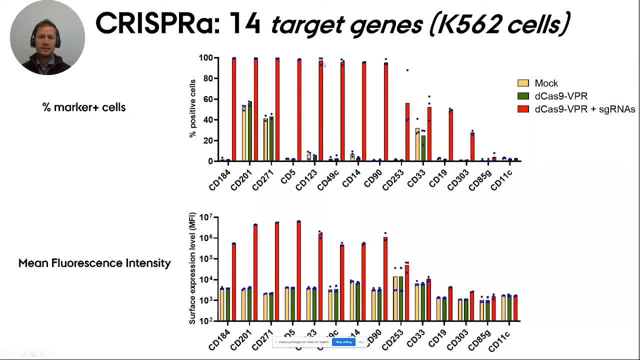 screen in k562 cells we see high up regulation for six. i believe regulation for six. i believe regulation for six, i believe eight, eight of those genes suboptimal, eight, eight of those genes suboptimal, eight, eight of those genes suboptimal. upregulation for four of the genes. and. 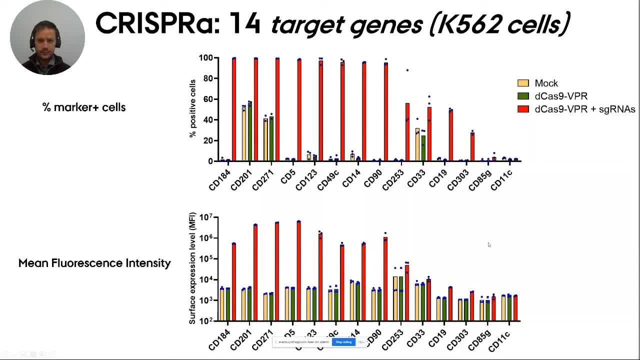 upregulation for four of the genes and upregulation for four of the genes, and we weren't really able to upregulate. we weren't really able to upregulate. we weren't really able to upregulate these two genes. this is then testing again, whether or not. 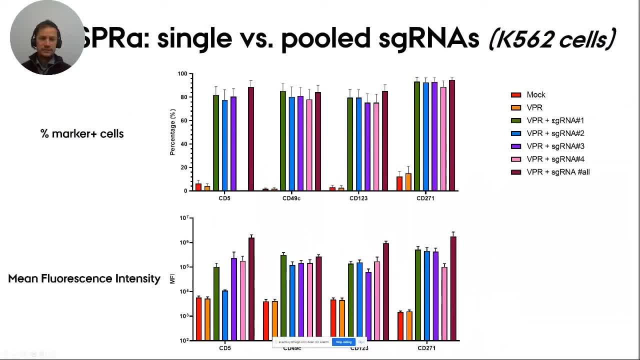 this is then testing again, whether or not this is then testing again whether or not a single guide rna would be a single guide. rna would be a single guide. rna would be sufficient to sufficient to sufficient to perform the upregulation and as you can. 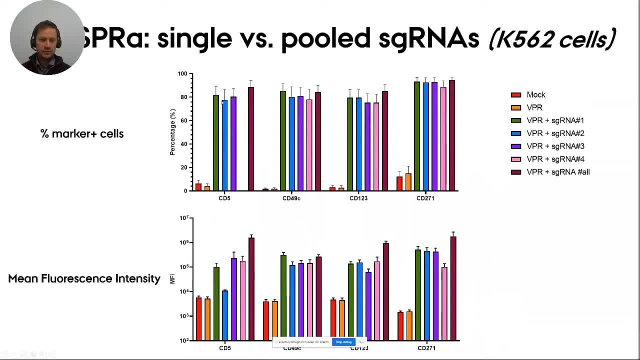 perform the upregulation and as you can perform the upregulation and as you can see, see, for cd5, we only had three guide rnas. for cd5, we only had three guide rnas. for cd5, we only had three guide rnas. they all performed quite similarly and 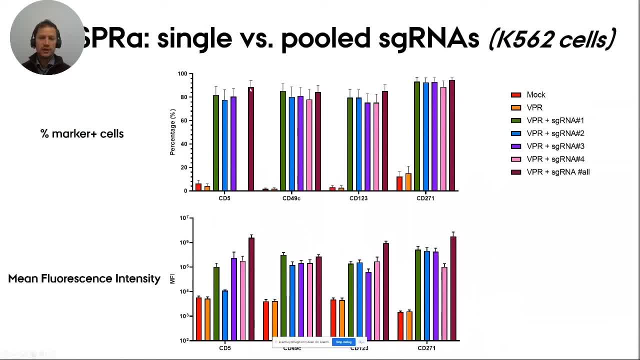 they all performed quite similarly. and they all performed quite similarly, and that was the case, for that was the case, for that was the case for these four genes, and when you combined these four genes, and when you combined these four genes, and when you combined all, all, all three or four guide rnas, we didn't see. 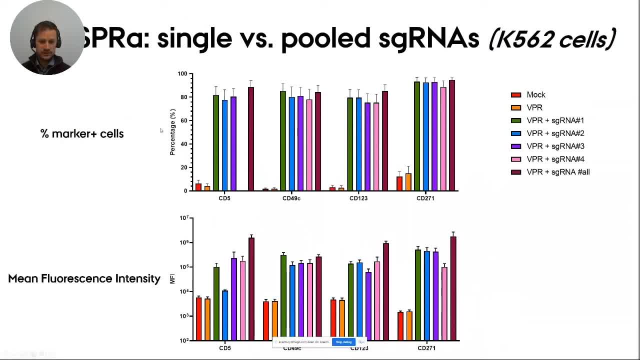 three or four guide rnas. we didn't see three or four guide rnas. we didn't see much higher. at least percent of cells, much higher, at least percent of cells, much higher, at least percent of cells that expressed the target gene. but if that expressed the target gene, but if 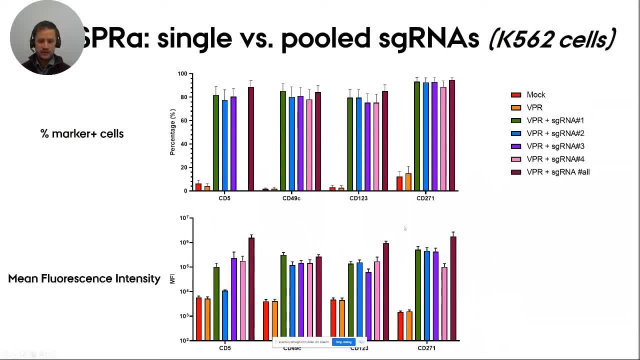 that expressed the target gene. but if you looked at, you looked at, you looked at the mfi of the cells, you could see that, the mfi of the cells, you could see that there was high expression of the, there was high expression of the, there was high expression of the targeted trans genes. when we combined 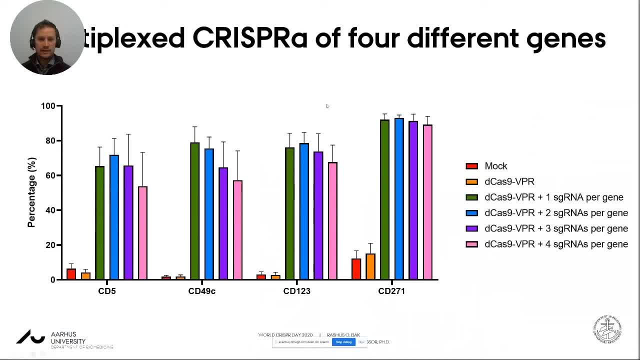 targeted trans genes. when we combined targeted trans genes, when we combined all guide rnas, all guide rnas, all guide rnas, then we tried to multiplex this, could we? then we tried to multiplex this, could we? then we tried to multiplex this. could we target all these four genes? 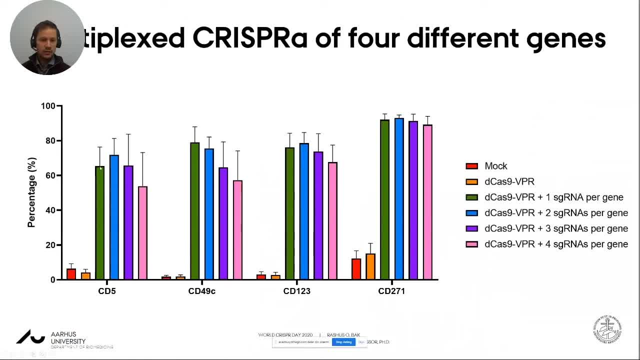 target all these four genes. target all these four genes simultaneously. if we took the most simultaneously, if we took the most simultaneously, if we took the most potent guide rna, we could get all genes. potent guide rna, we could get all genes. potent guide rna, we could get all genes regulated. 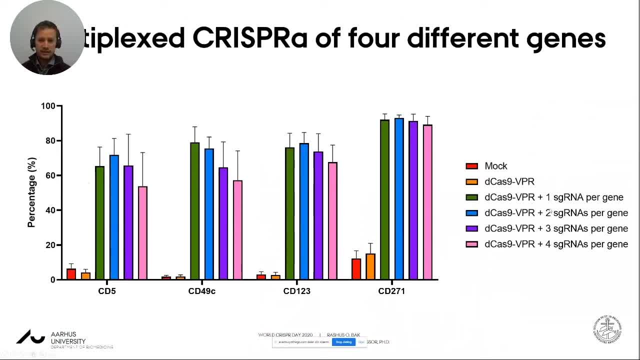 regulated, regulated, upregulated by almost 70 percent, upregulated by almost 70 percent, upregulated by almost 70 percent, and the optimal condition was with two, and the optimal condition was with two, and the optimal condition was with two guides per gene. so that would be. 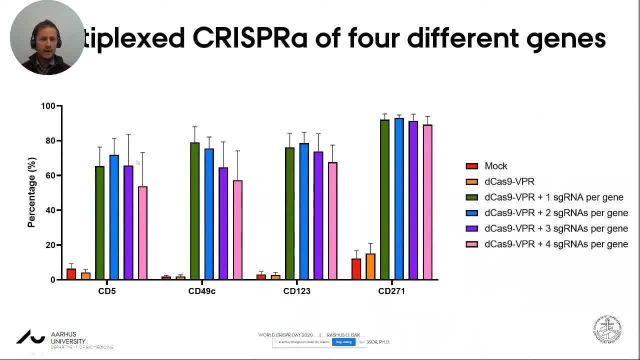 guides per gene. so that would be guides per gene. so that would be electroporation with eight guides in electroporation with eight guides in electroporation with eight guides in total, total, total, and beyond that we would see a decline, and beyond that we would see a decline. 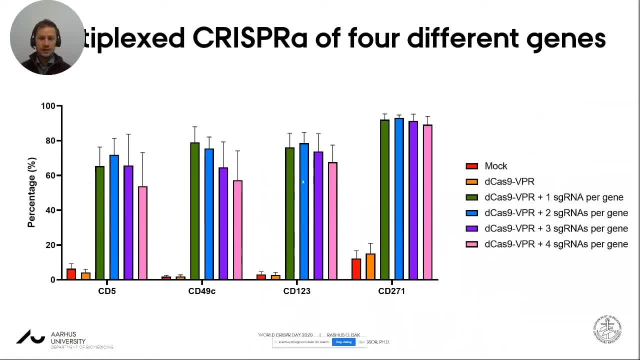 and beyond that we would see a decline in activation, probably because of in activation, probably because of in activation, probably because of saturation of the system. saturation of the system, saturation of the system. so it seems like a single guide, rna per. so it seems like a single guide, rna per. 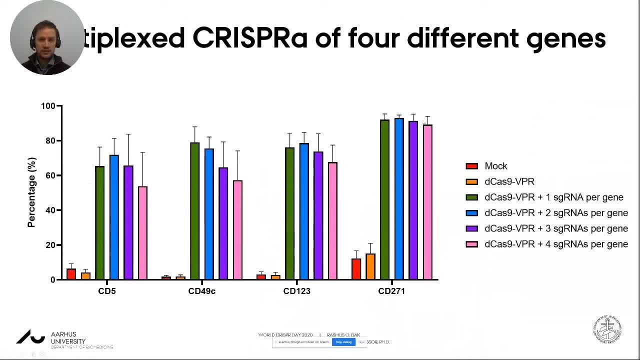 so it seems like a single guide rna per gene. if it's a, if it's an optimal guide gene, if it's a, if it's an optimal guide gene, if it's a, if it's an optimal guide, rna can facilitate, rna can facilitate. 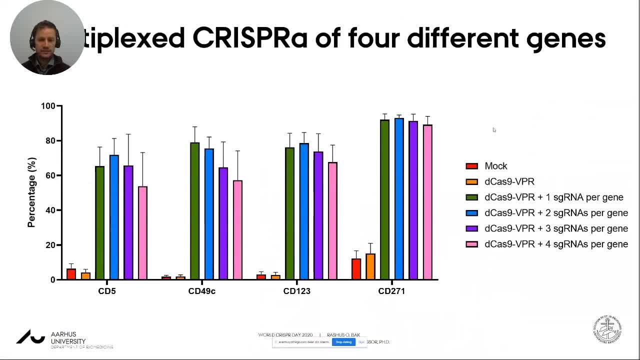 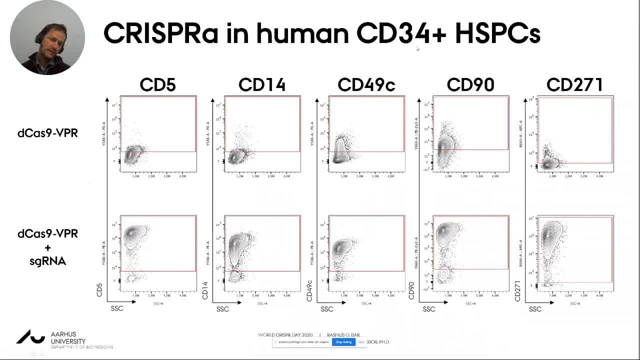 rna can facilitate multiplexed activation simultaneously of multiplexed activation simultaneously of multiplexed activation simultaneously of different genes, different genes, different genes. and then we turned uh towards primary, and then we turned uh towards primary, and then we turned uh towards primary cells. this is data from cd34 positive. 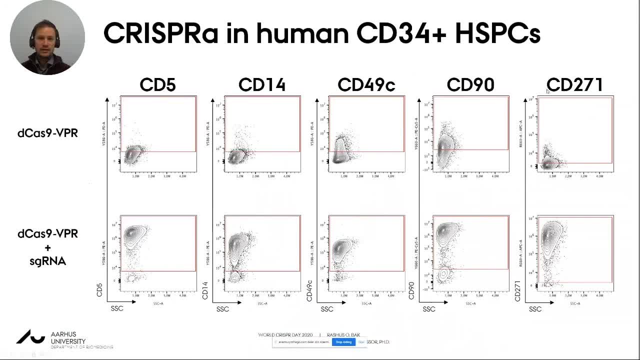 cells. this is data from cd34 positive cells. this is data from cd34 positive hematopoietic stem and progenitor cells. hematopoietic stem and progenitor cells. hematopoietic stem and progenitor cells. and. we targeted these four genes as: and. we targeted these four genes as: 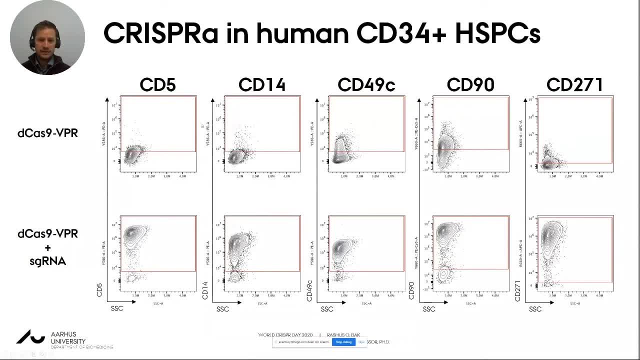 and we targeted these four genes, as you'll see up here. these are the basal you'll see up here. these are the basal you'll see up here. these are the basal levels, expressed levels. expressed levels expressed in cd34 cells. and when we introduce in cd34 cells and when we introduce the crispr activation system. 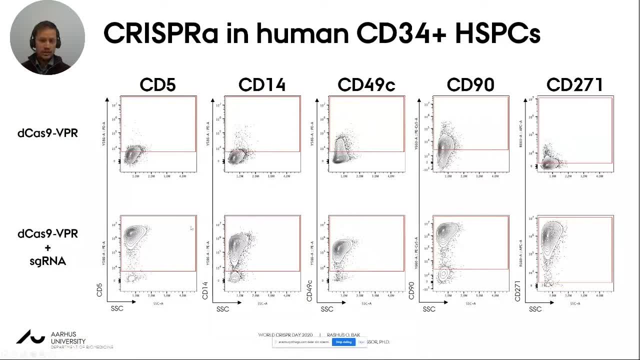 the crispr activation system. the crispr activation system by electroporation. again you see a high by electroporation. again you see a high by electroporation. again you see a high upregulation. i don't have the numbers. upregulation, i don't have the numbers. 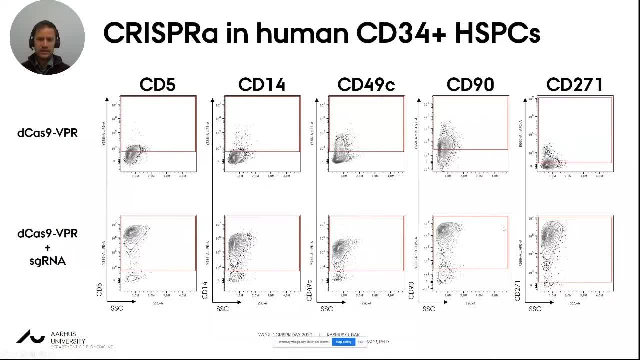 upregulation. i don't have the numbers here, but it's uh, i believe it's above here, but it's uh, i believe it's above here, but it's uh, i believe it's above 85 percent, 85 percent, 85 percent for all these target genes. so 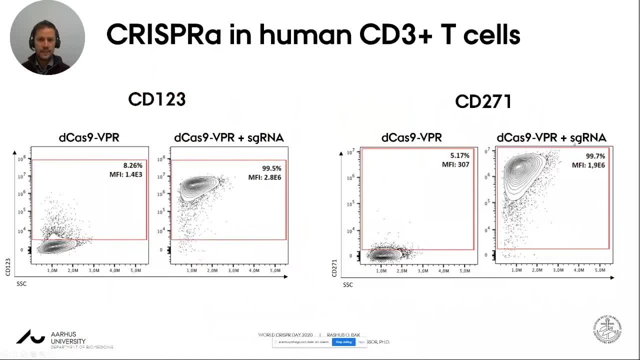 for all these target genes. so for all these target genes. so translating very well to a clinically translating very well to a clinically translating very well to a clinically relevant cell type. relevant cell type. relevant cell type. we also tested cd3 positive t cells with. we also tested cd3 positive t cells with. 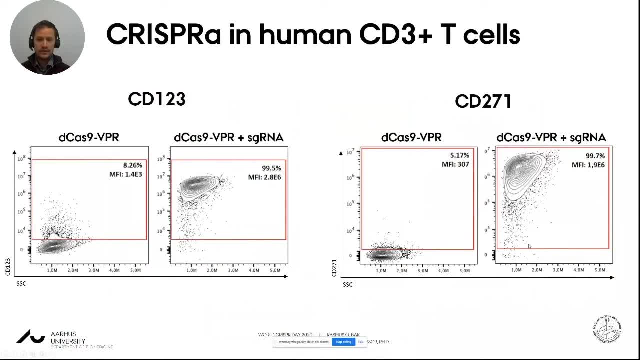 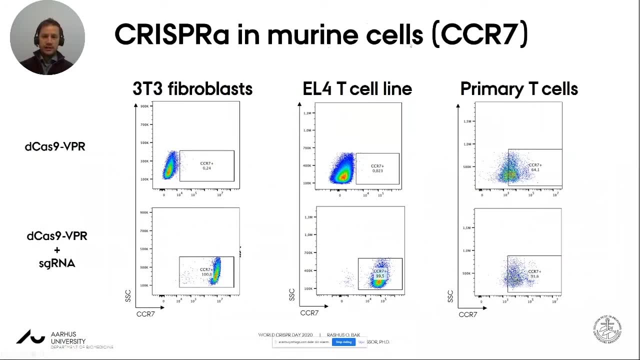 we also tested cd3 positive t cells with these two genes works. these two genes works. these two genes works just as well here in this setting. this just as well here in this setting. this just as well here in this setting. this is human t cells. we also tested it in some murine cells. 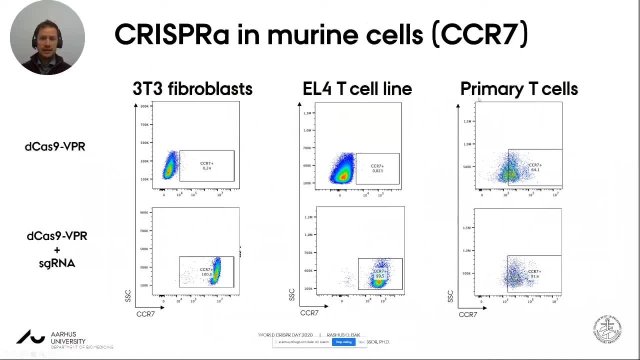 we also tested it in some murine cells. we also tested it in some murine cells. this is: this is: this is 3g3 fibroblasts: a t cell line and primary. 3g3 fibroblasts: a t cell line and primary. 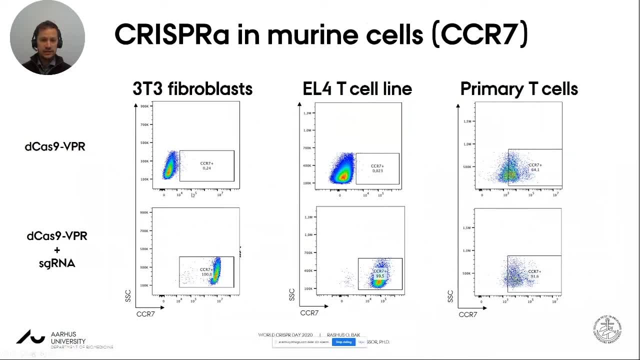 3g3 fibroblasts, a t cell line and primary t cells. this is only targeting a single t cells. this is only targeting a single t cells. this is only targeting a single gene: ccr7. and as you can see, here we get gene ccr7. and, as you can see, here we get 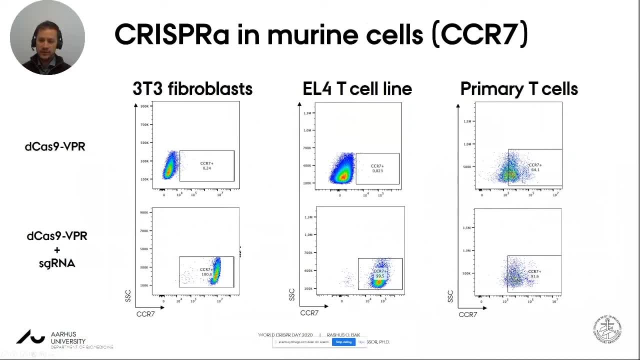 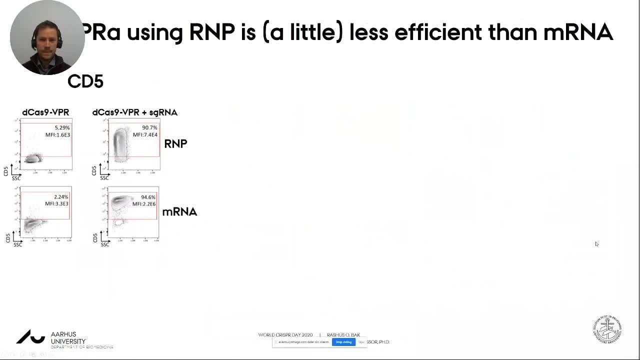 gene ccr7. and, as you can see here, we get potent upregulation in the two cell, potent upregulation in the two cell, potent upregulation in the two cell. a little bit. we then got a hold of uh some. we then got a hold of uh some. 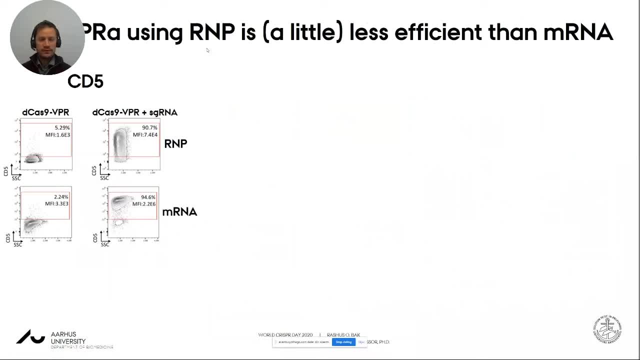 we then got a hold of, uh, some recombinant protein. this is not the recombinant protein. this is not the recombinant protein. this is not the tribe. the tripartite activator domain, the vpr. the tripartite activator domain, the vpr. 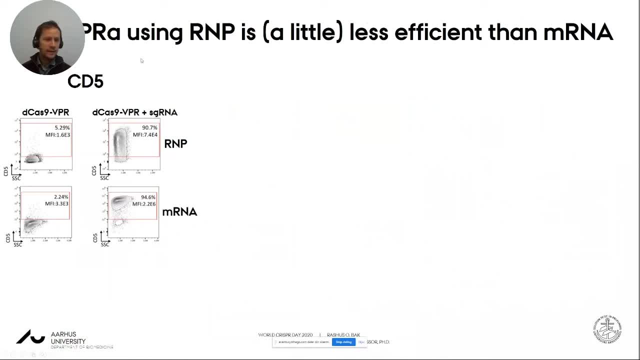 the tripartite activator domain, the vpr domain. this is only the vp64 domain. so, domain, this is only the vp64 domain. so domain, this is only the vp64 domain. so, uh, we would expect, expect this rnp to be. uh, we would expect, expect this rnp to be. 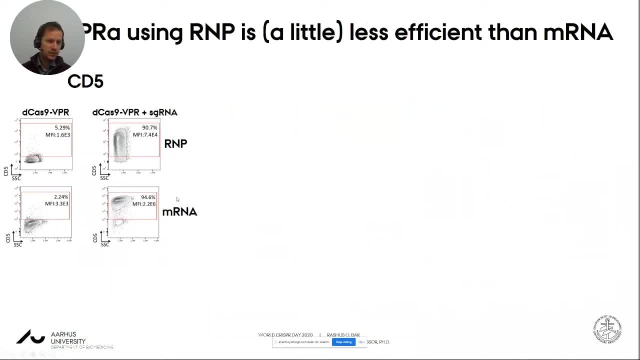 uh, we would expect, expect this rnp to be a little less efficient than the mrna, a little less efficient than the mrna, a little less efficient than the mrna that we are, that we are, that we are using, which is also the case here for cd5. 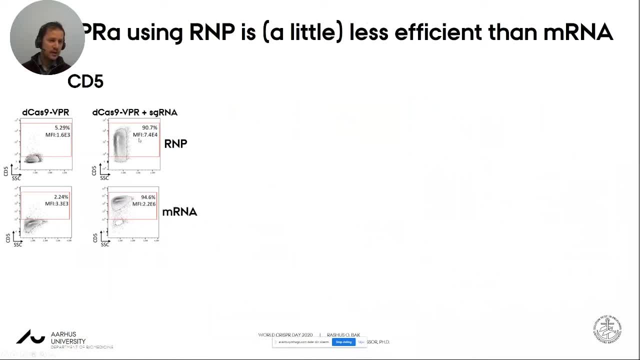 using- which is also the case here for cd5- using, which is also the case here for cd5, if we compare the upregulation, if we compare the upregulation, if we compare the upregulation facilitated by the rmp complex it's facilitated by the rmp complex it's. 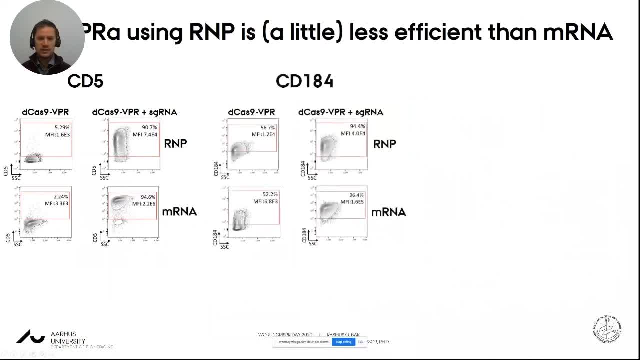 facilitated by the rmp complex. it's potent, but it's not as potent as the potent. but it's not as potent as the potent, but it's not as potent as the mrna or some of the other genes. it's mrna, or some of the other genes. it's. 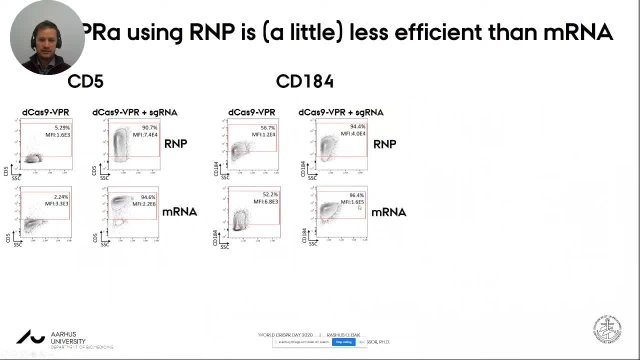 mrna or some of the other genes. it's, it's almost as potent as it's almost as potent as it's almost as potent as messenger rna. this is cxcr4, and finally it's cxcr4. and finally it's cxcr4. and finally, for cd201, you'll see um just as high. 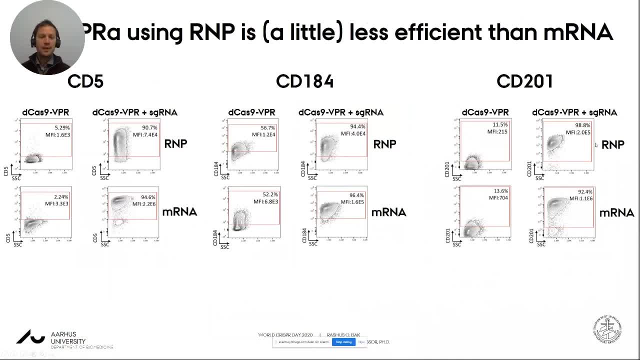 for cd201, you'll see um just as high. for cd201, you'll see um just as high, if not better up regulation with, if not better up regulation with, if not better up regulation with, rmp. and then we turn towards crisper, and then we turn towards crisper. 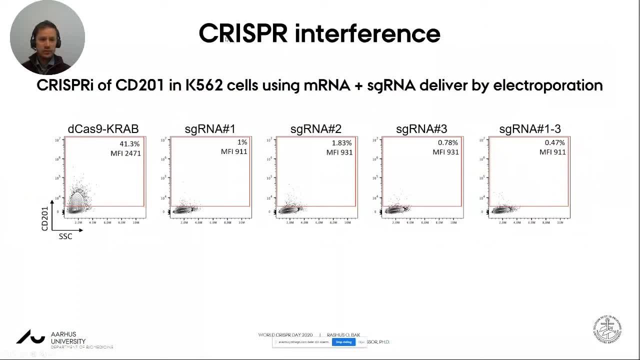 and then we turn towards crisper interference, or crisper eye interference, or crisper eye interference, or crisper eye with the same rna system in vitro, with the same rna system in vitro, with the same rna system in vitro, transcribed, transcribed, transcribed messenger rna with dcas9 crap. 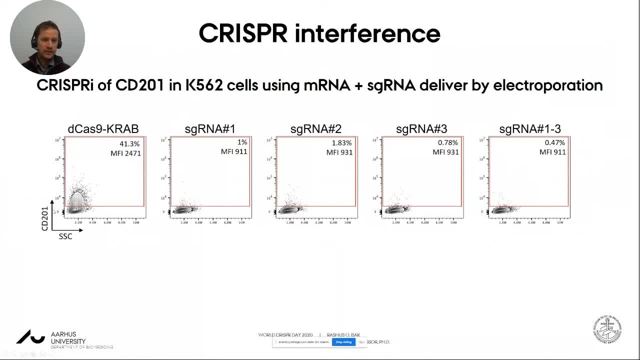 messenger rna with dcas9 crap. messenger rna with dcas9 crap. and here we are repressing the cd201 and here we are repressing the cd201 and here we are repressing the cd201 gene in k562 cells. it's not highly. 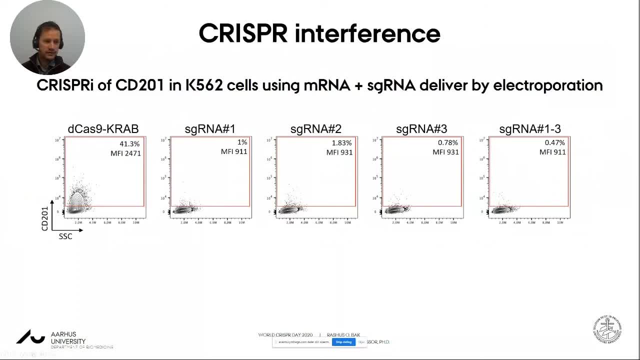 gene in k562 cells. it's not highly gene in k562 cells. it's not highly expressed in k562 cells and it's not expressed in k562 cells and it's not expressed in k562 cells and it's not that difficult to down regulate it this. 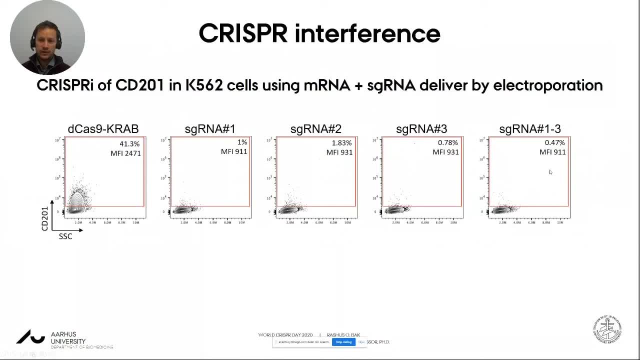 that difficult to down regulate it? this that difficult to down regulate it. this is just using single guide rnas or a is just using single guide rnas or a is just using single guide rnas or a combination of three guide rnas and we. combination of three guide rnas and we. 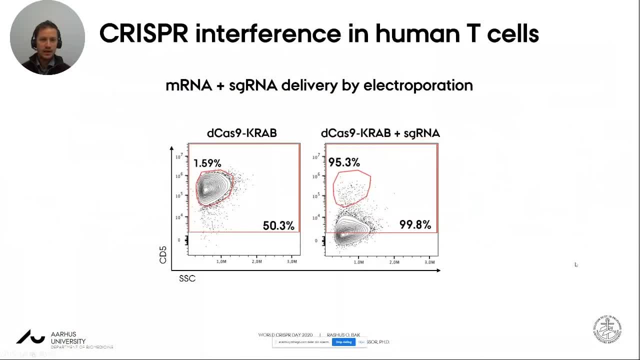 combination of three guide rnas and we can completely suppress the expression, can completely suppress the expression, can completely suppress the expression of this gene. then we turn to, then we turn to, then we turn to human t cells and try to repress a highly human t cells and try to repress a highly 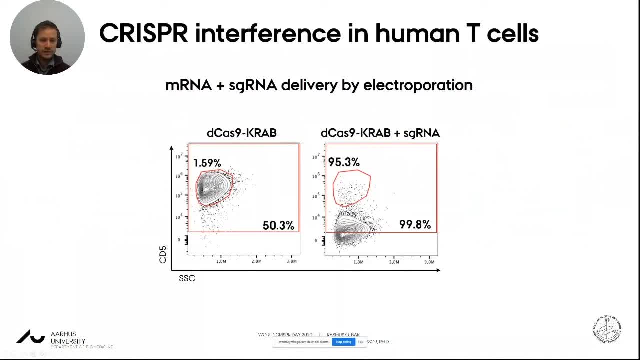 human t cells and try to repress a highly expressed gene. this is cd5 expressed gene. this is cd5 expressed gene. this is cd5, as you'll see here in this gate, and we, as you'll see here in this gate, and we, as you'll see here in this gate, and we can actually get all the cells out of. 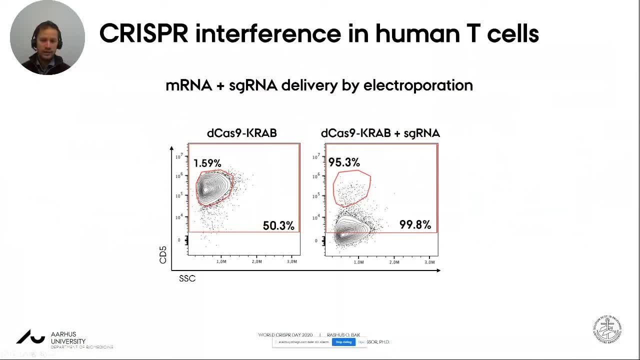 can actually get all the cells out of, can actually get all the cells out of this gate, or almost at least. but we this gate, or almost at least. but we this gate, or almost at least, but we can't fully, can't fully, can't fully repress this, this gene. 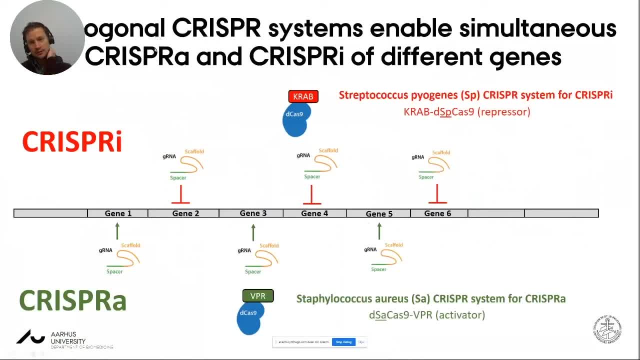 and finally we also try to do orthogonal, and finally we also try to do orthogonal, and finally we also try to do orthogonal or or or, opposing gene regulation. so here we have to turn to orthogonal crisper, have to turn to orthogonal crisper, have to turn to orthogonal crisper, systems for the repression we can use. 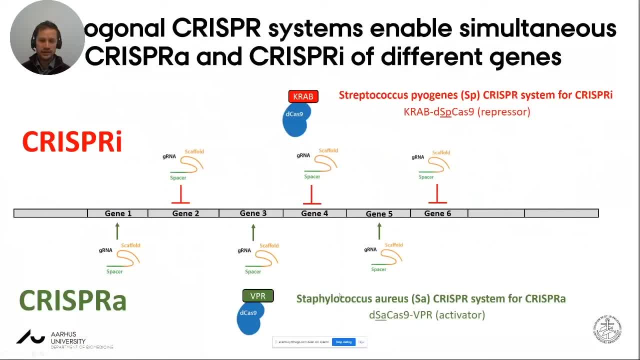 systems for the repression. we can use systems for the repression. we can use the sp, the sp, the sp crisper system and for activation we can crisper system and for activation we can crisper system and for activation we can use the sa crisper system so that the 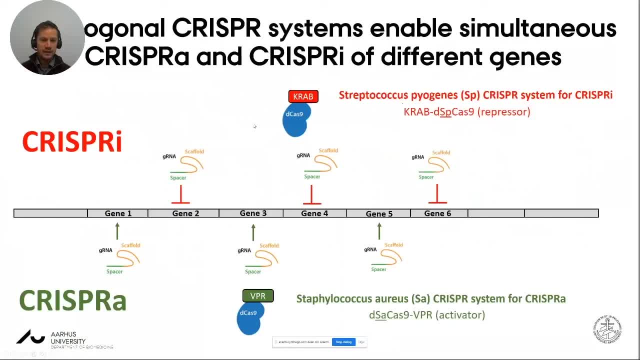 use the sa crisper system so that the use the sa crisper system so that the guide rnas do not interfere with each guide rnas do not interfere with each guide rnas do not interfere with each other other other. so we try to do that and this is an. 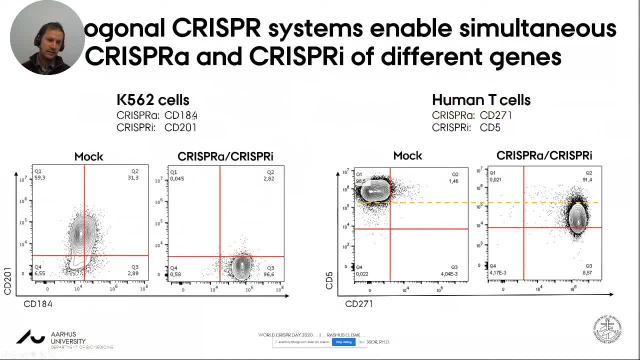 so we try to do that and this is an. so we try to do that and this is an experiment in k562 cells- up regulating experiment in k562 cells, up regulating experiment in k562 cells, up regulating cxcr4 and down regulating cd201. so we 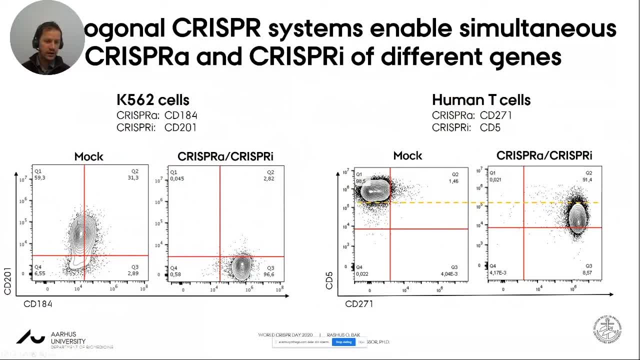 cxcr4 and down regulating cd201. so we cxcr4 and down regulating cd201. so we are looking here at the basal levels, in are looking here at the basal levels, in are looking here at the basal levels in k562 cells and we are then hoping to. 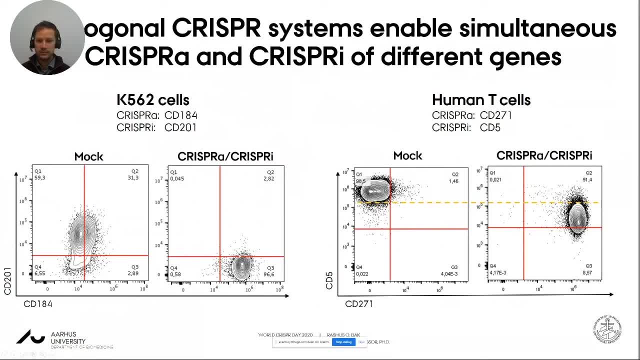 k562 cells and we are then hoping to k562 cells and we are then hoping to see all the cells turn to quadrant three, see all the cells turn to quadrant three, see all the cells turn to quadrant three. and that's exactly what happens here. and that's exactly what happens here. 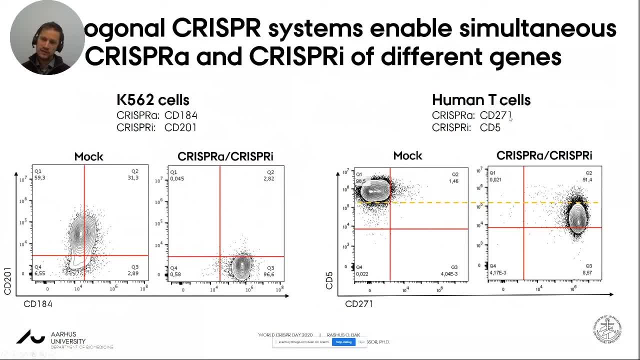 and that's exactly what happens here: very potent, very potent, very potent in human t cells. we activated cd271 in human t cells, we activated cd271 in human t cells, we activated cd271. and down regulated cd5, and again we. and down regulated cd5, and again we. 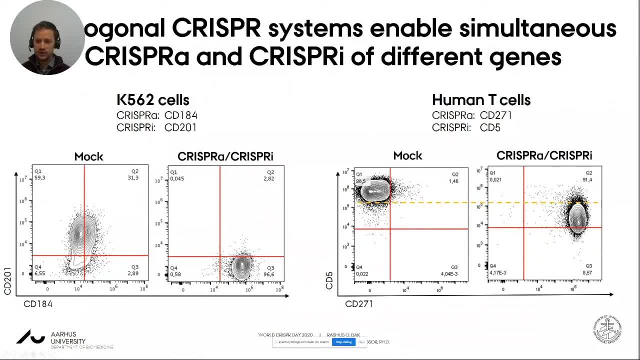 and down regulated cd5. and again, we can't completely repress cd5, but we can. can't completely repress cd5, but we can can't completely repress cd5, but we can. we can get them under the level of the. we can get them under the level of the. 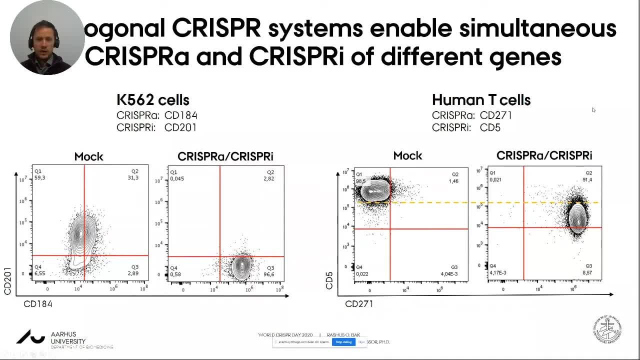 we can get them under the level of the highly expressing cells here, highly expressing cells here, highly expressing cells here. so it looks quite promising, although we so it looks quite promising, although we so it looks quite promising, although we cannot fully repress some of the genes, cannot fully repress some of the genes. 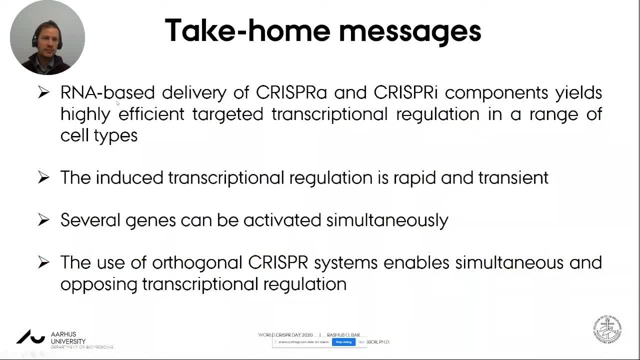 cannot fully repress some of the genes, at least, at least at least. so. the take-home messages here is that an so. the take-home messages here is that an so the take-home messages here is that an rna-based delivery of rna-based delivery of. 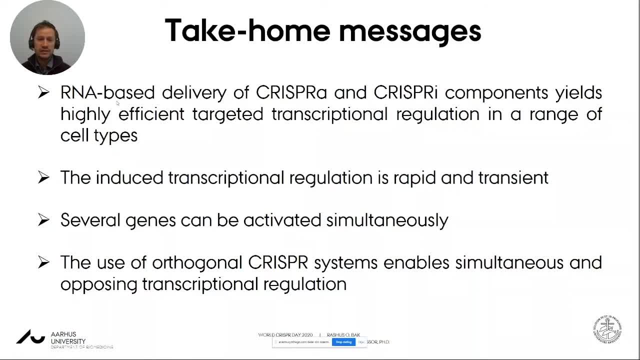 rna-based delivery of CRISPR-A and CRISPR-I components. can CRISPR-A and CRISPR-I components, can CRISPR-A and CRISPR-I components can give very high efficiencies of give very high efficiencies, of give very high efficiencies of targeted transcriptional regulation. targeted transcriptional regulation. targeted transcriptional regulation. we've done this in a bunch of cell. we've done this in a bunch of cell. we've done this in a bunch of cell types now, and it seems to be highly. types now, and it seems to be highly. 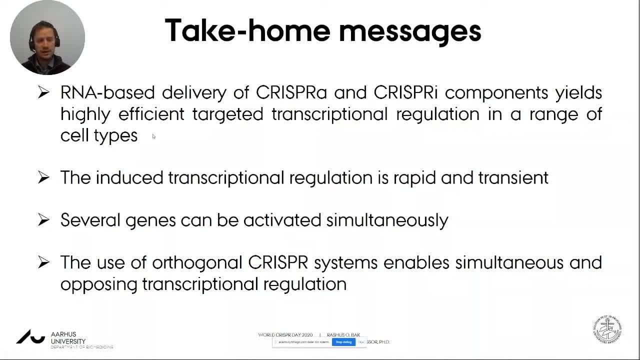 types now, and it seems to be highly functional, at least for most of the functional, at least for most of the functional, at least for most of the genes. there are genes that we genes. there are genes that we genes. there are genes that we cannot seem to regulate at the moment. 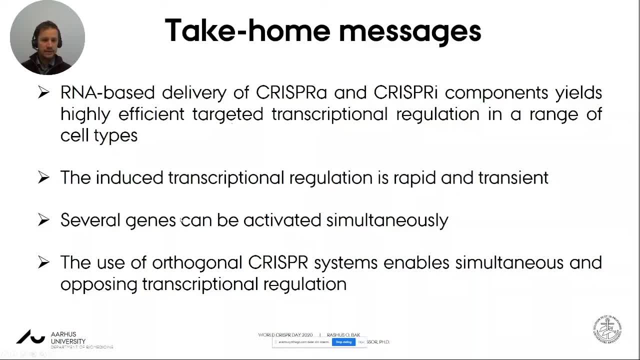 cannot seem to regulate at the moment. cannot seem to regulate at the moment. a little bit, a little bit, a little bit, depending on the choice of the guide, depending on the choice of the guide, depending on the choice of the guide, rnas and we can activate rnas and we can activate. 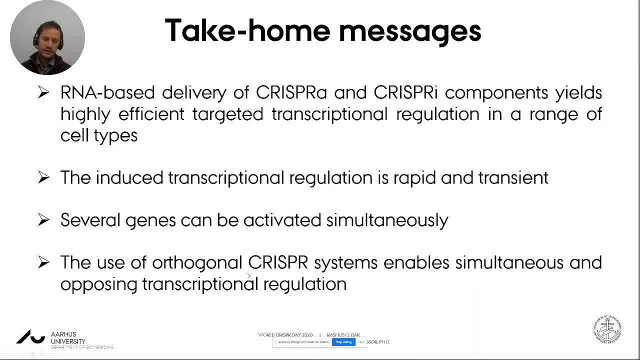 rnas and we can activate several genes simultaneously, and we can several genes simultaneously and we can several genes simultaneously and we can use this orthogonal use, this orthogonal use, this orthogonal CRISPR system to um to to do opposing CRISPR system to um to to do opposing. 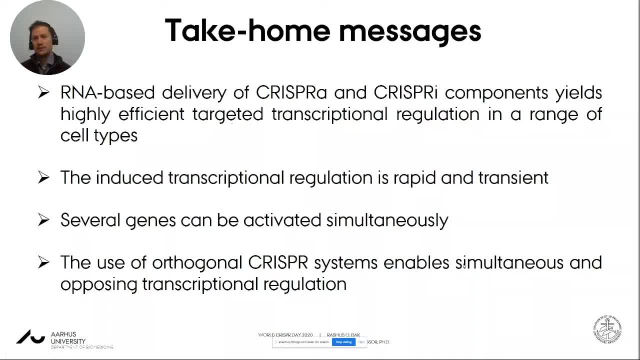 CRISPR system to um, to to do opposing transcriptional regulation at the same transcriptional regulation at the same transcriptional regulation at the same time. so i think this is a time, so i think this is a time, so i think this is a really promising tool to to study basic. 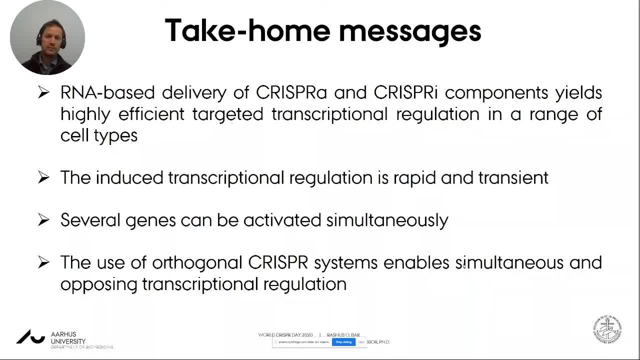 really promising tool to to study basic, really promising tool to to study basic biology of some of these primary cell biology, of some of these primary cell biology, of some of these primary cell types, but it also might be possible to types, but it also might be possible to. 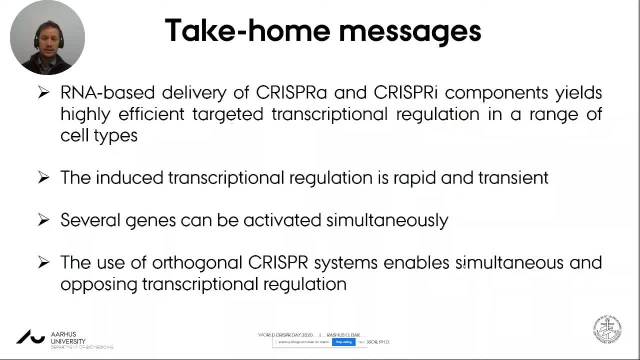 types, but it also might be possible to implement this technology. these implement this technology, these implement this technology. these technologies um in cell therapies and technologies um in cell therapies and technologies um in cell therapies and even gene therapy. to to enhance some of even gene therapy. to to enhance some of 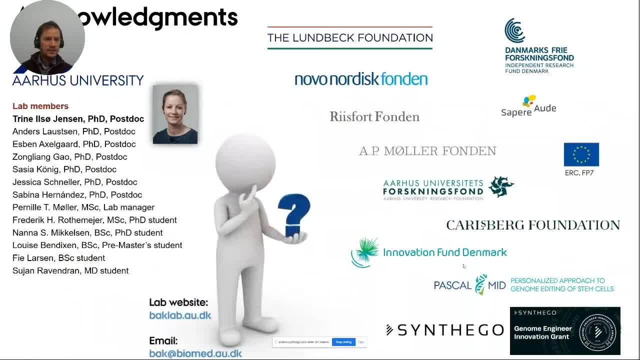 even gene therapy to, to enhance some of these cell products, these cell products, these cell products and acknowledgements here the work was and acknowledgements here the work was, and acknowledgements here the work was mainly driven by a postdoc, Trine Jensen, mainly driven by a postdoc Trine Jensen. 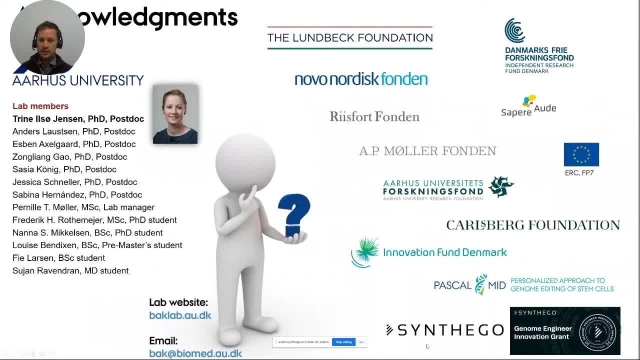 mainly driven by a postdoc, Trine Jensen, together with other members from the lab, together with other members from the lab, together with other members from the lab. and I also have to acknowledge the and I also have to acknowledge the and I also have to acknowledge the support from Synthego. I won a genome. 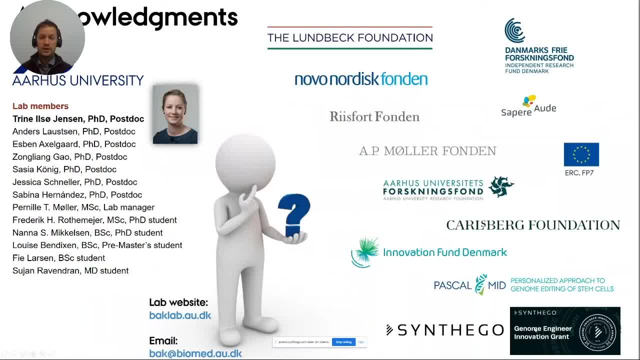 support from Synthego. I won a genome support from Synthego. I won a genome engineer innovation grant that supported engineer innovation grant. that supported engineer innovation grant. that supported precisely this project, precisely this project, precisely this project, and with that I'd like to to thank. 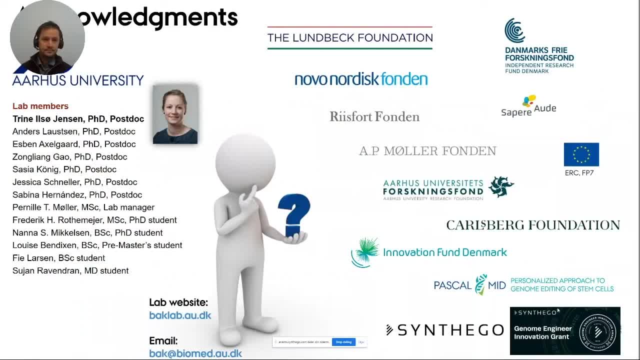 and with that I'd like to to thank, and with that I'd like to to thank again Synthego for inviting me and I'd again Synthego for inviting me and I'd again Synthego for inviting me and I'd take questions. great, thank you, Erasmus. that was really. 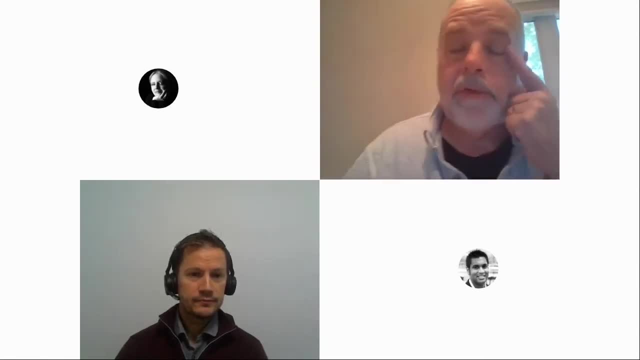 great. thank you Erasmus. that was really great. thank you Erasmus. that was really impressive, impressive, impressive. so we have one question for you in the. so we have one question for you in the. so we have one question for you in the q a and I have one of my own. 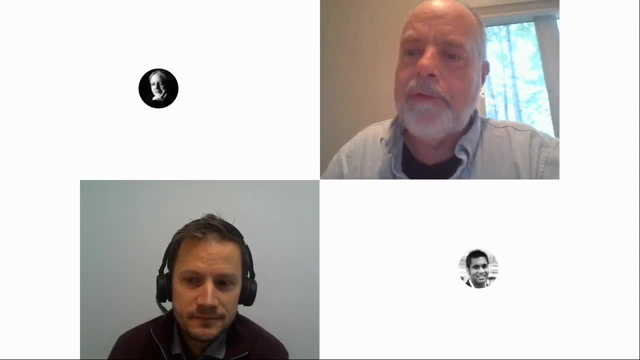 so the question is: do you see the same? so the question is: do you see the same? so the question is: do you see the same four-day kinetics in four-day kinetics, in four-day kinetics, in cd35 plus and cd3 plus, as in k562, cd35 plus and cd3 plus, as in k562? 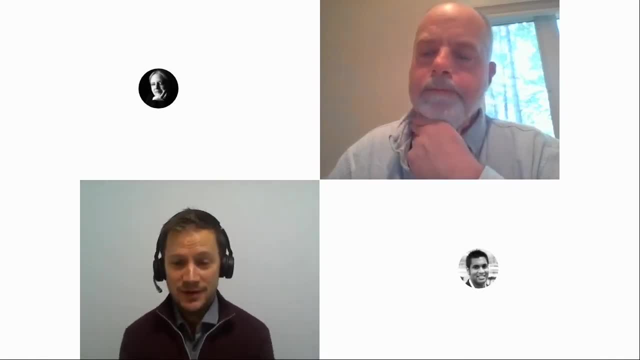 cd35 plus and cd3 plus, as in k562. yeah, so we're actually performing those. yeah so we're actually performing those. yeah, so we're actually performing those. experiments, experiments, experiments. right as we speak, almost um so I can. right, as we speak, almost um, so I can. 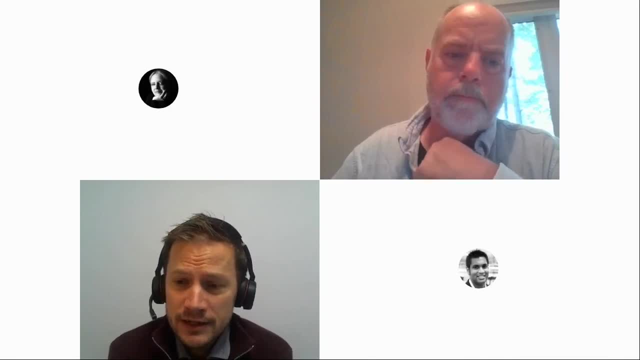 right as we speak, almost um, so I can. I can actually only say what we're seeing. I can actually only say what we're seeing. I can actually only say what we're seeing in the cd34 cells, as in the cd34 cells, as in the cd34 cells, as as the expression turns on, not as it. as the expression turns on, not as it as the expression turns on, not as it wears off, but it's. it seems to be turned, wears off, but it's. it seems to be turned, wears off, but it's. it seems to be turned on just as fast within. 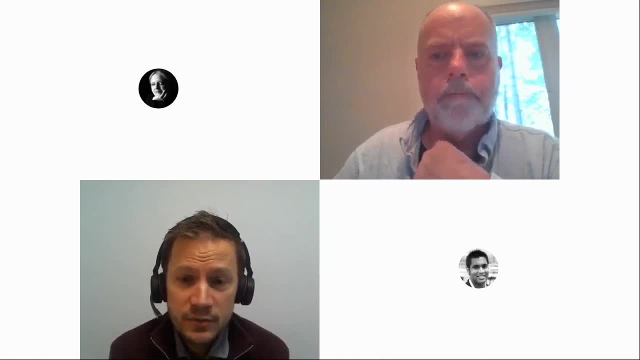 on just as fast, within, on just as fast, within within hours, we can see the first cells. within within hours, we can see the first cells. within within hours, we can see the first cells start expressing these target genes. so start expressing these target genes. so start expressing these target genes. so it's quite amazing. I would have thought. it's quite amazing. I would have thought it's quite amazing. I would have thought it would take longer, but within two it would take longer, but within two it would take longer. but within two hours after electroporation we see. hours after electroporation, we see. 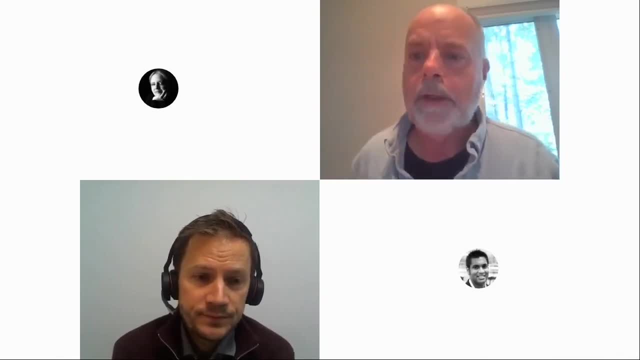 hours after electroporation we see expression okay, a second question has come in. do okay, a second question has come in. do okay, a second question has come in. do you see any difference in toxicity? you see any difference in toxicity? you see any difference in toxicity between using rna versus rnp? 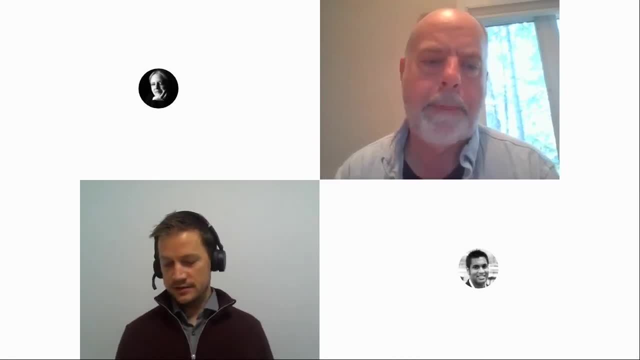 between using rna versus rnp, between using rna versus rnp in primary cells. yeah, of course that's in primary cells. yeah, of course that's in primary cells. yeah, of course that's been a been a been a long-standing question in this field. long-standing question in this field. 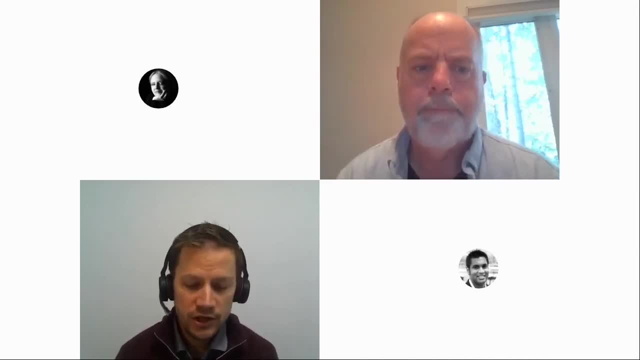 long-standing question in this field- also for introducing indels and doing also for introducing indels and doing also for introducing indels and doing hdr and targeted gene correction. hdr and targeted gene correction. hdr and targeted gene correction. there is some toxicity with the rna. there is some toxicity with the rna. 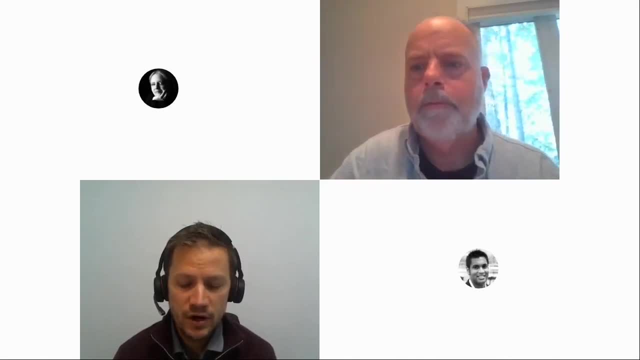 there is some toxicity with the rna based systems. you can tweak these a based systems. you can tweak these a based systems. you can tweak these a little bit by little bit, by little bit, by by changing or modifying some of the. by changing or modifying some of the. 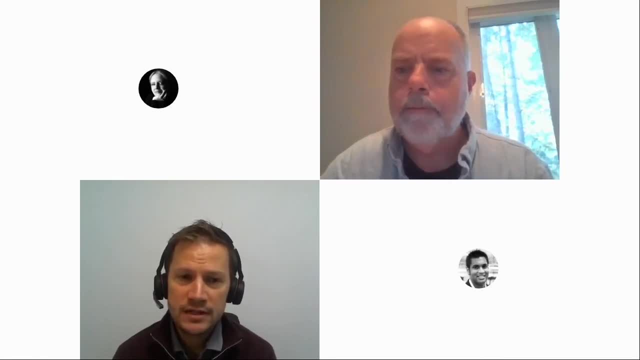 by changing or modifying some of the nucleotides during the in vitro nucleotides during the in vitro nucleotides during the in vitro transcription, transcription, transcription. but there is some sensing of these rnas. but there is some sensing of these rnas. but there is some sensing of these rnas inside the cells. 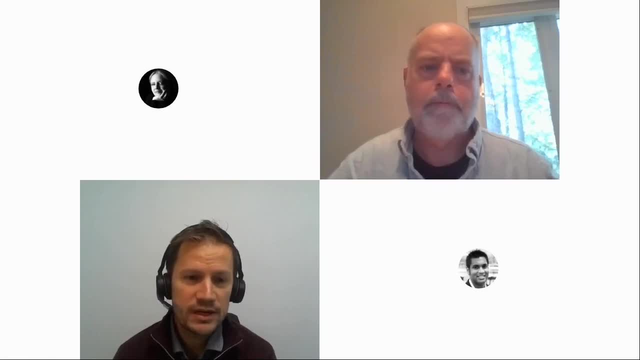 inside the cells, inside the cells, and it does impact the cells a little and it does impact the cells a little and it does impact the cells a little bit, not too much. it doesn't compare to bit, not too much. it doesn't compare to bit, not too much. it does compare to plasmid delivery at all. that's just. 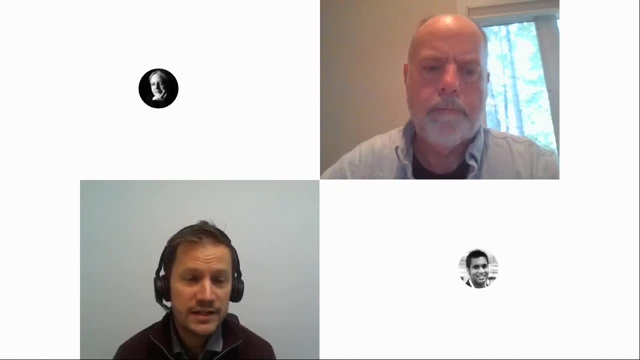 plasmid delivery at all. that's just plasmid delivery at all. that's just completely toxic to these cells, but. but completely toxic to these cells, but. but completely toxic to these cells, but. but rmp is generally, rmp is generally. rmp is generally less toxic. um. 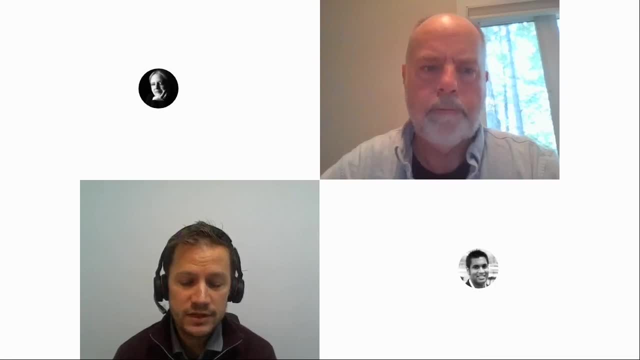 less toxic um, less toxic, um. so, if it's possible, i would definitely so. if it's possible, i would definitely so. if it's possible, i would definitely advise, advise, advise to use this system. okay, one last question: did you check the? okay, one last question: did you check the? 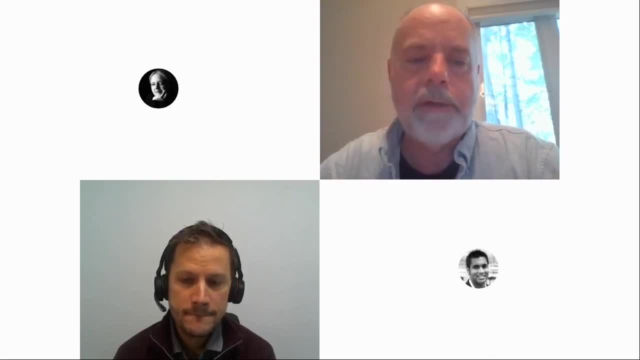 okay. one last question: did you check the differentiation progenitor potential of differentiation? progenitor potential of differentiation? progenitor potential of the hscs after activation of your target: the hscs after activation of your target: the hscs after activation of your target gene. 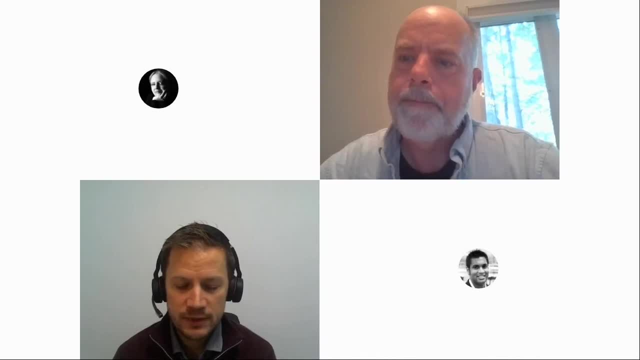 gene gene. yeah, i know we we haven't tested that. but yeah, i know we we haven't tested that. but yeah, i know we we haven't tested that. but we are looking in uh into transplants. we are looking in uh into transplants. we are looking in uh into transplants and we'll have data from that at some. 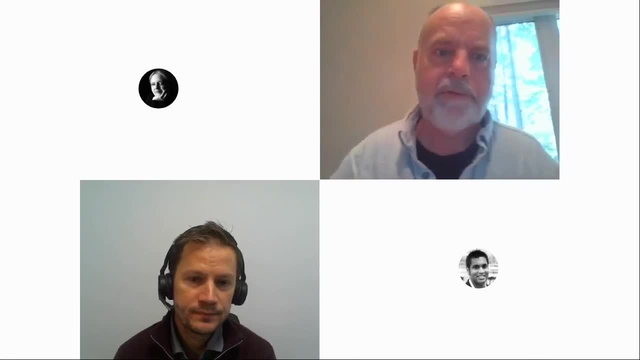 and we'll have data from that at some and we'll have data from that at some point, point, point. okay, there are questions that are okay. there are questions that are okay. there are questions that are continuing to come in, but i think we continuing to come in, but i think we. 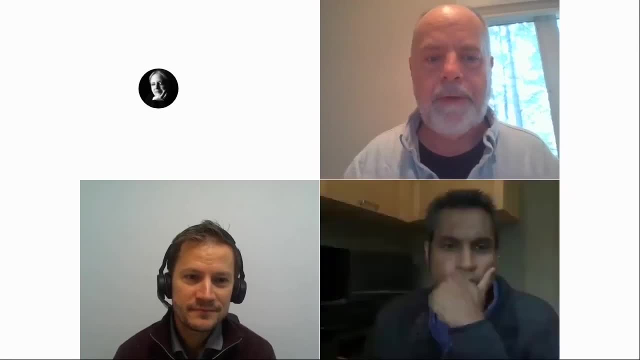 continuing to come in, but i think we should stop there at the end of the, should stop there at the end of the. should stop there at the end of the session, session session. thank you very much. thank you very much. thank you very much, erasmus and chris, for your wonderful. 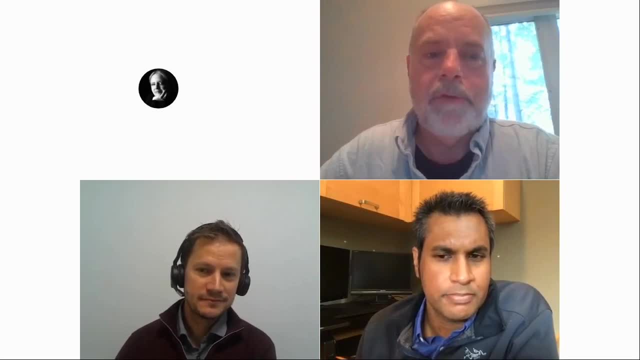 erasmus and chris for your wonderful erasmus and chris for your wonderful talks, talks, talks. and i would just say, and i would just say, and i would just say, enjoy the rest of your day on crisper. enjoy the rest of your day on crisper. enjoy the rest of your day on crisper world day. 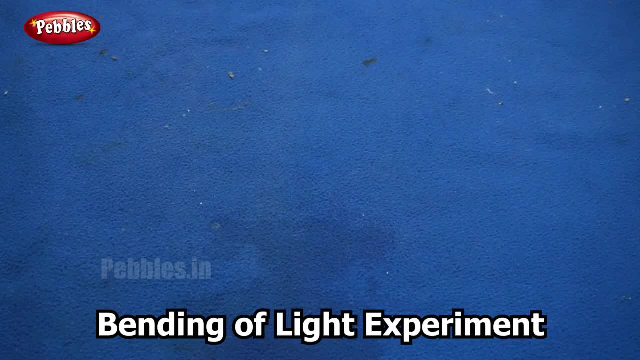 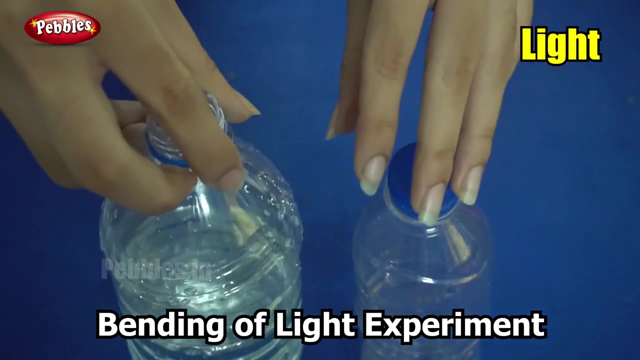 Now, in this experiment, I am going to show you how light gets reflected and refracted when it comes to the interface between two medium. For this, you will need a plastic bottle and some water. You will also need a source of light, like a torch light In this. 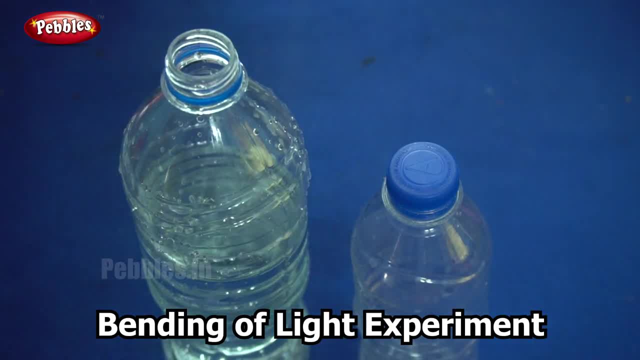 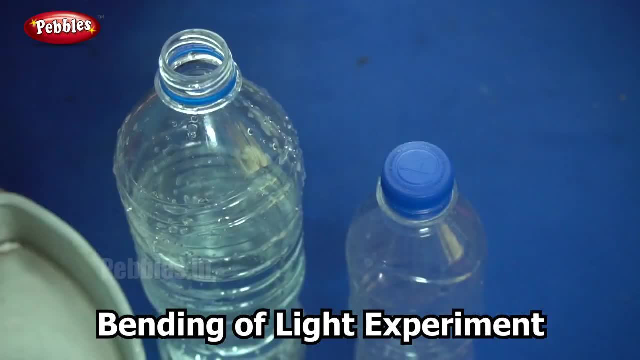 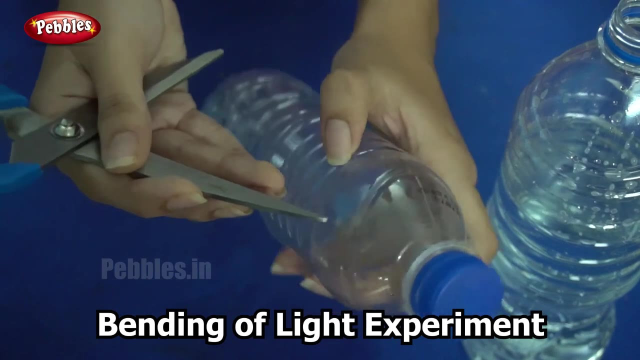 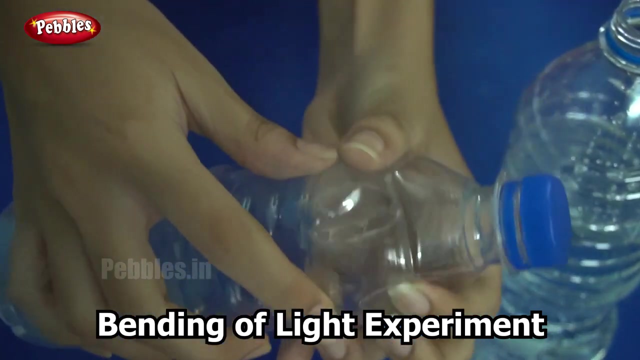 case, I will use my phone torch and you can use a sink. Here I am using a tray so that the water doesn't spill all over the table. First step is to make a hole in the bottle. I am making the hole towards the top, So I have made a hole in the bottle You can. 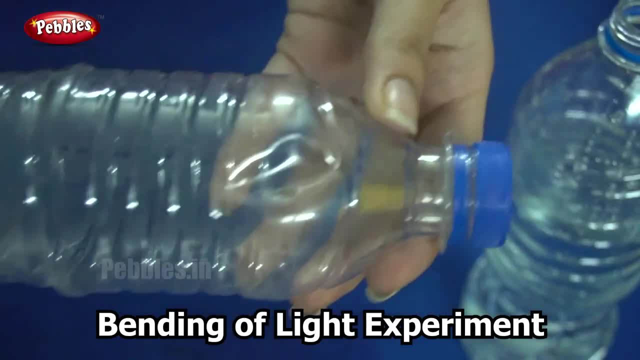 see it's a very small one. Next step is to make a plan for any待 strain. We need to make a spoon at the top, So I have made a hole in the bottle. You can see it's a very small one. Next step: I have told